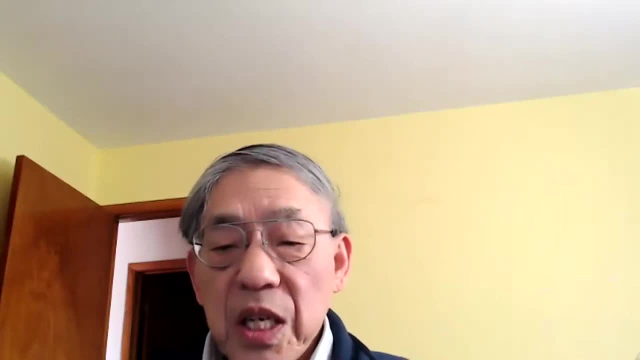 University. For the past 15 years, Dr Kelly and his students have conducted extensive research on rare plant biology and conservation in ecosystems across New Jersey. This year, the New Jersey Native Plant Society has started partnering with Dr Kelly with these projects. 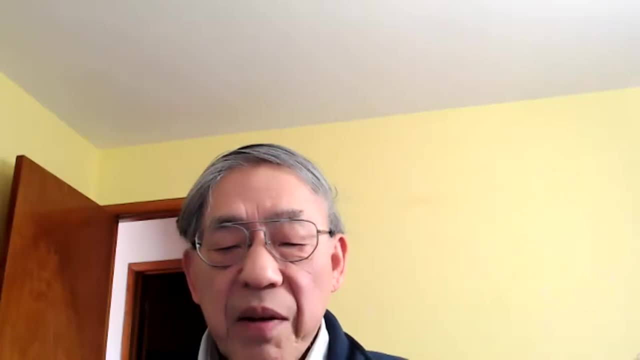 In addition, he's been working on the impacts of deer and invasive species and other factors on New Jersey forests. He and his students are conducting ongoing research into the long-term results of deer exclosures, Hunting programs, prescribed burnings and native plantings. We may also hear a few words about his 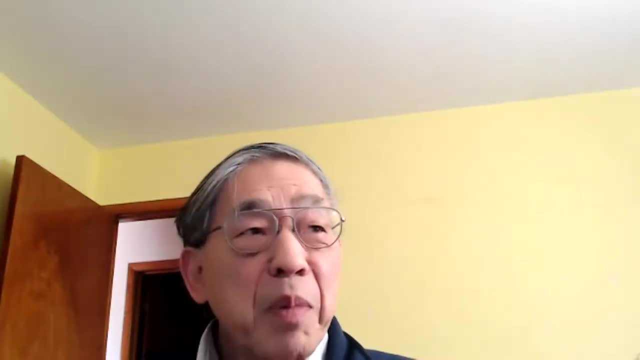 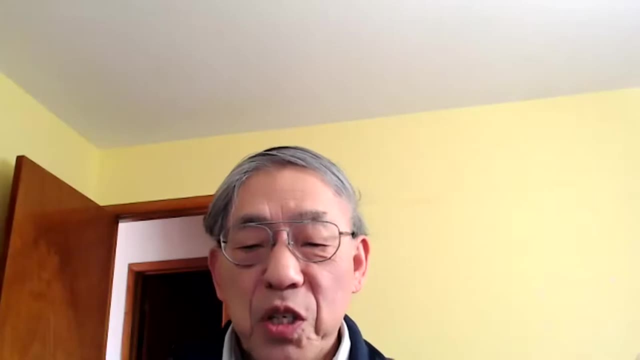 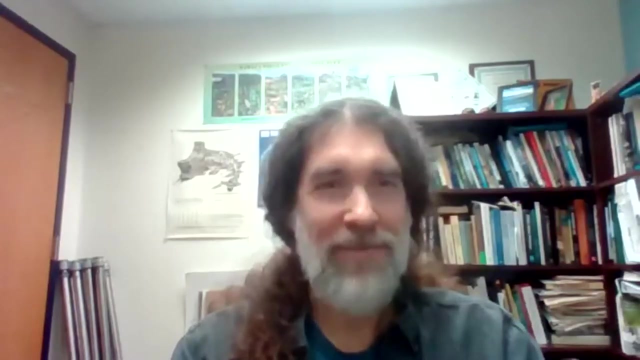 Sea-Beach Amaranth Conservation Project and public participation in that kind of those endeavors. So I'm very pleased to introduce Dr Jay Kelly to everybody And the floor is yours, Dr Kelly. Great Thanks, Can you hear me okay? Yes, All right, So I'll try to share my screen now. 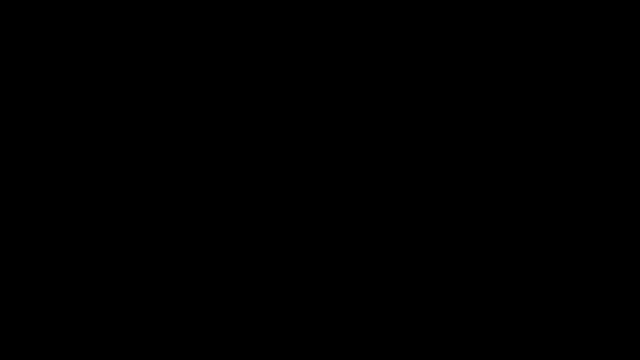 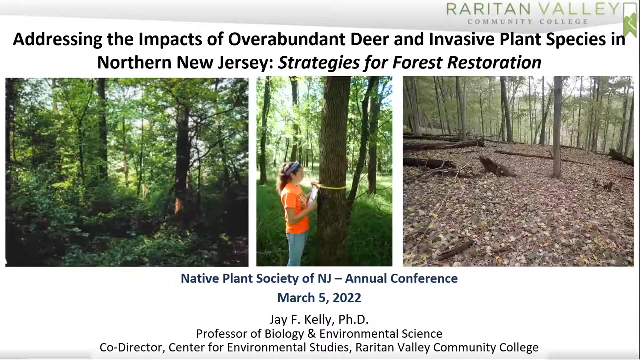 Hopefully this goes without a hitch. Sure, All right. So I'll try to share my screen now. Hopefully this goes without a hitch. Great, Yeah, All right, That looks okay. Yep, Great Well, thanks again, Hubert, for the invitation to come talk to you all. 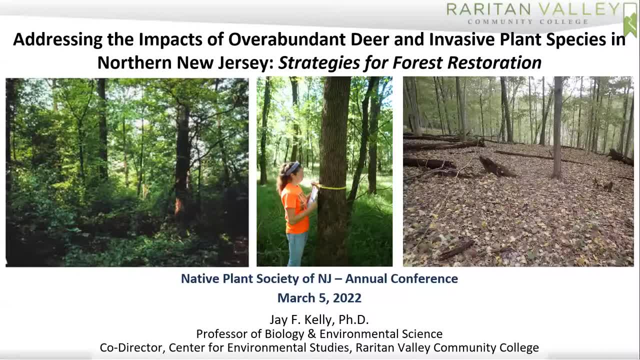 to the Society as well. Hopefully next year we'll all get to meet in person. It's always really encouraging and inspiring to be around other plant lovers in the state. So I guess we'll just have to make do this year through Zoom and be grateful that we. 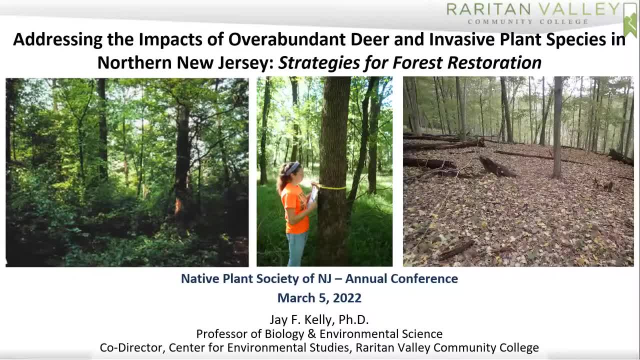 at least have this way to connect with each other. So I'll be talking to you today about the impact of deer and invasive plant species on our forests, primarily in northern New Jersey, and then I'll review some of the different solutions and strategies for tackling these. 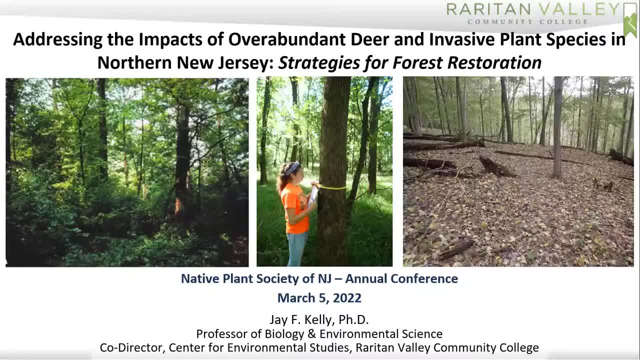 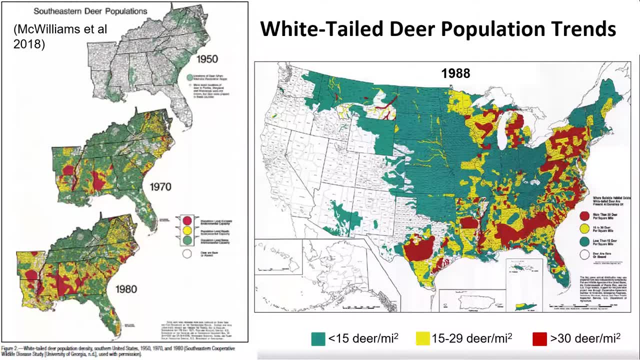 problems based on some of the research that we've been conducting, as well as others in the region. As members of a Native Plants Society, I'm sure the problem of deer populations is not new to you. but before we get into some of the impacts that deer are having on our forest, 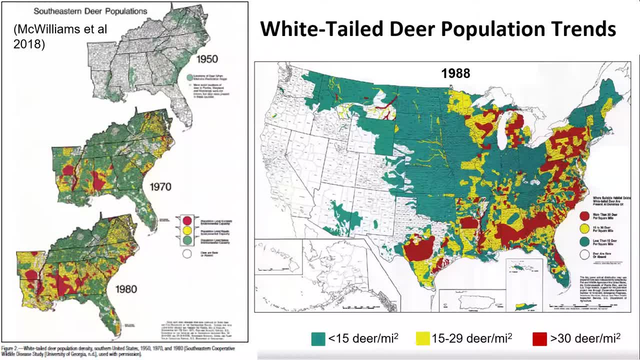 it's important to take a step back and realize that the recovery of deer in our area really represents a conservation success story, and it's recognized around the world as such, because approximately 100 years ago, around the end of the 1800s, deer had been exterminated throughout most. 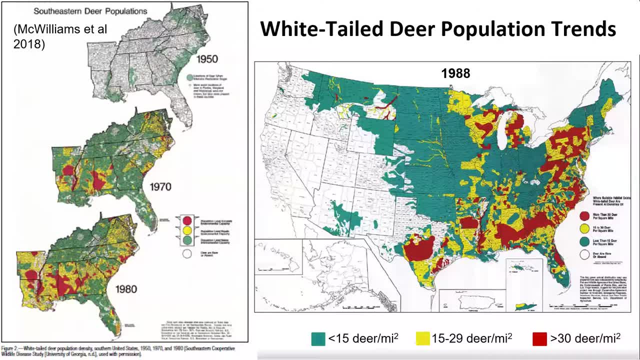 of their range in North America, white-tailed deer in particular, including in New Jersey, and it was really only through the work of generations of conservationists and hunters and legislators that deer were able to make a comeback. So you can see some data from the 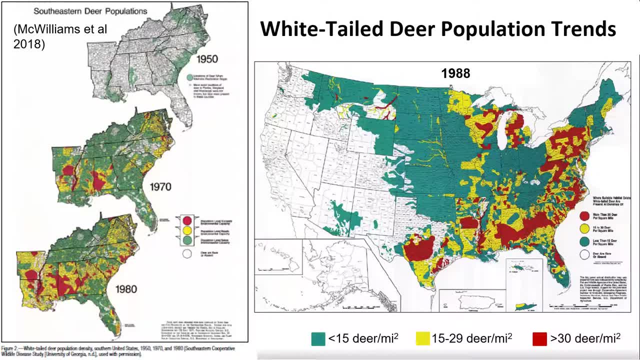 University of Georgia that they compiled for the southeastern states on the left, and you can see that still by 1950, white-tailed deer were still absent from much of their historic range. but by 1970, they had largely recovered throughout most of that range and were already starting to. 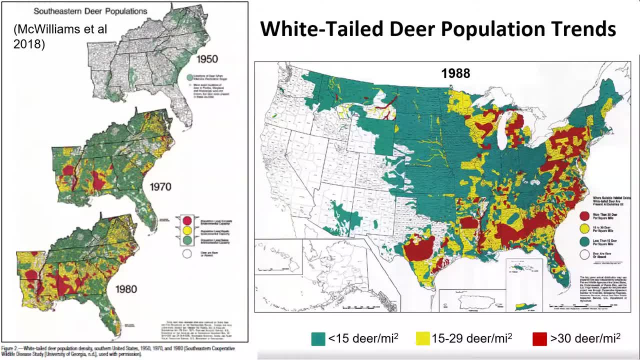 show some signs of problematic levels. returning to some areas And the reasons why deer populations exceeded their background historic levels is because a number of conditions had changed during the course of the last century that allowed them to rise to levels that had never been seen before. The first thing that happened was the historic extermination of natural predators. 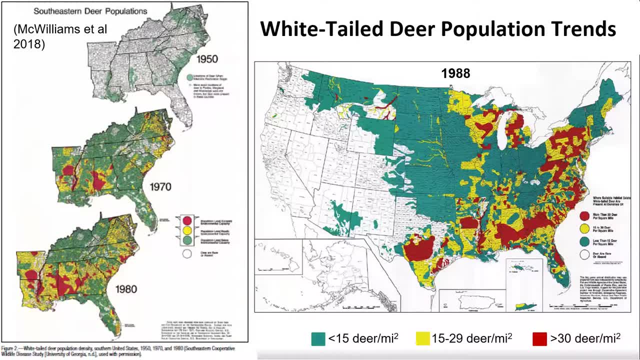 primarily wolves, andıria cattle and N'kaulini bred animals and cougars in my area. But equally important was the fragmentation of forest environments by both agriculture and suburban development Throughout the eastern seaboard, which created the ideal conditions. 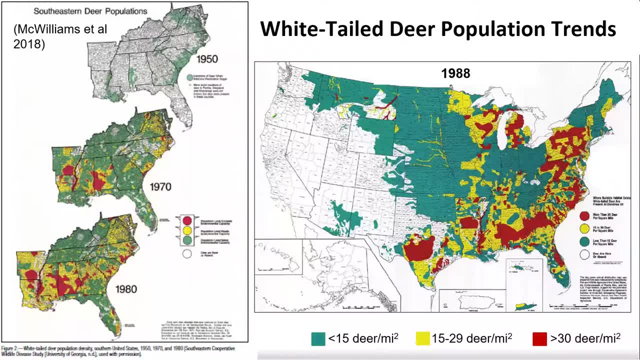 that deer prefer, which are edge habitats in forests, and also provided supplemental food resources in the surrounding landscape that deer rely on- in our yards and our gardens, our landscaping and in farm fields- and that additional food source combined with the lack of predation. 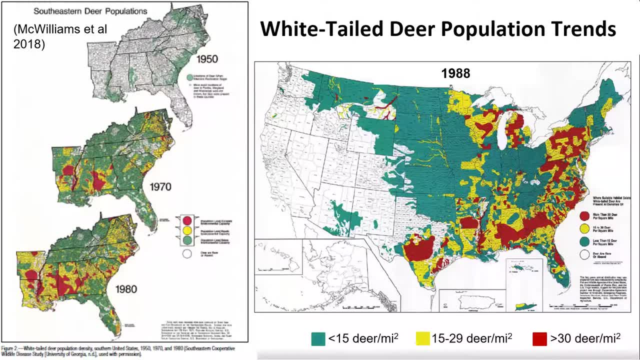 to uh increase exponentially far beyond what had ever been seen um previously on the continent, and so you can see that since the 1970s, deer populations continued to rise such that by around 1990 they had risen to really problematic levels throughout much of the eastern states. 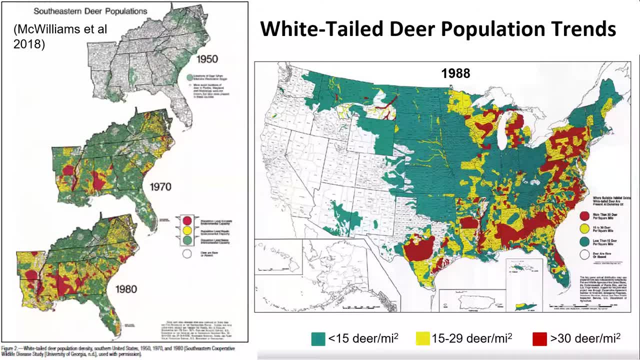 along the gulf of mexico and great lakes region, and certainly in new jersey. the colors that you see on the map here- we'll talk about the significance of these numbers in a second. but yellow indicates populations that are above 15 deer per square mile and red indicates areas. 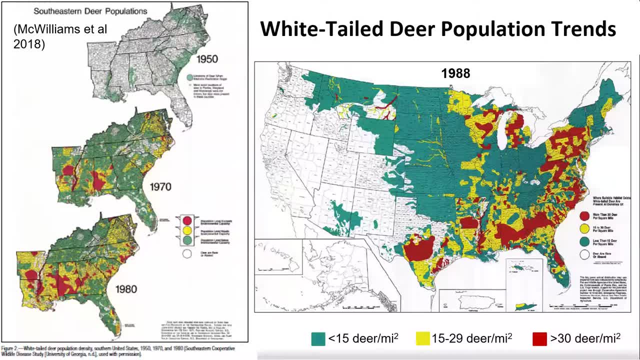 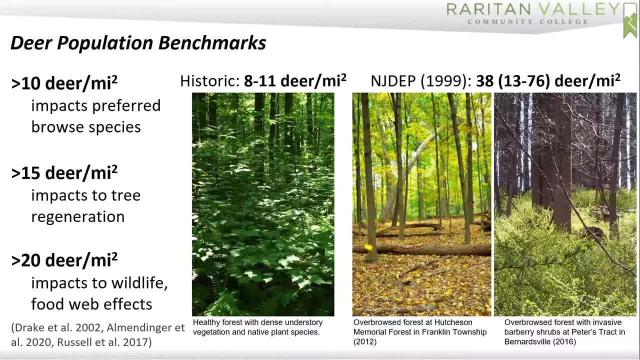 where deer are above 30 per square mile, both of which are problematic to varying degrees. historically, deer were thought to be approximately 10 per square mile and it's important to recognize that deer, again, are a native part of our ecosystem. they play an important role in our forest, serving to disperse the seeds of plants and also to suppress the 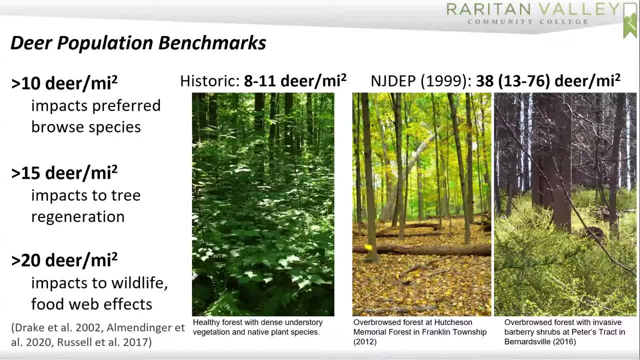 plants that have a competitive advantage over other species, and so when deer are at the the proper population densities, they can actually play an enhancing role in supporting biodiversity in the forest by creating room for other, less competitive species to be able to get a foothold. when deer get above 10 per square mile, though, we've seen a number of studies from our region. 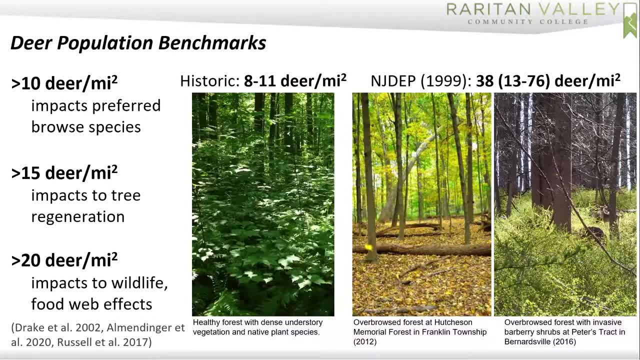 that show that certain kinds of impacts start to take place, and the first thing that tends to happen is that the preferred browse species- the species that are the tastiest to beer- start to decline noticeably in the landscape, and that's been seen with trilliums in pennsylvania and the 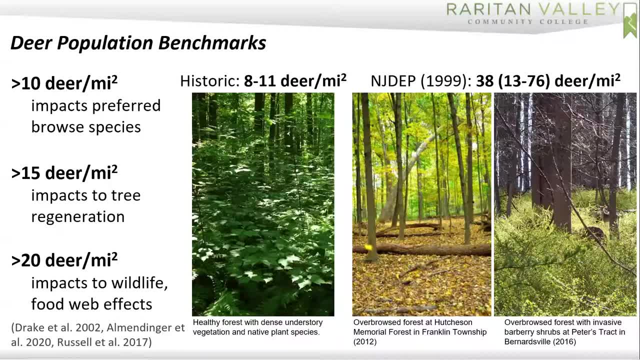 great lakes. it's been seen with swamp pink down in south jersey, which i'll talk about in a minute. it's been seen with hemlocks in the great lakes and the northern states, and so those species that are preferred by deer begin to decline. when deer exceed 15 per square mile, you start to see tree regeneration begin to shut down dramatically. 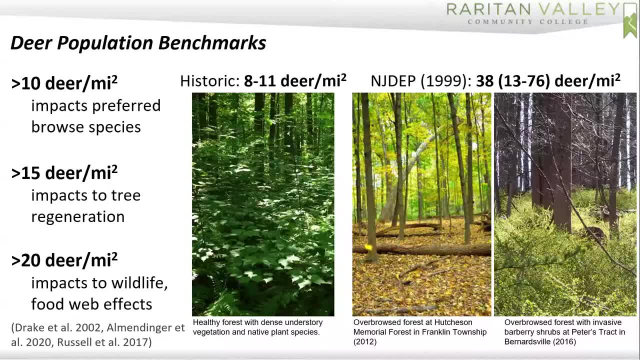 as a whole, with significant declines and really a whole host of tree seedlings in the understory, and then, when you get above 20 deer per square mile, you start to see effects happening throughout the food web, because the vegetation, of course, is the primary food source of everything else. 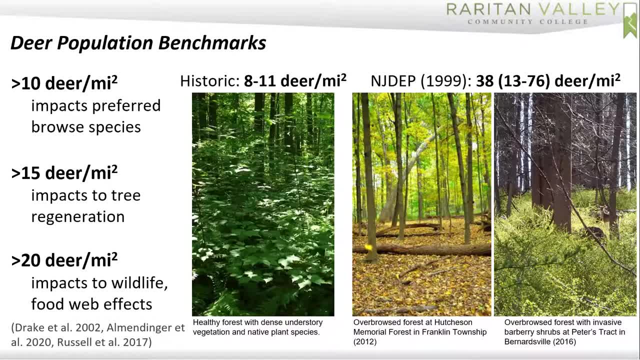 in the forest ecosystem, and so you see declines in the forest, and so there's a lot of, there's a lot of, there's a lot of 青- irresponsible- there's a lot of, and you can't see very far into the forest as a consequence of that really rich vegetation. 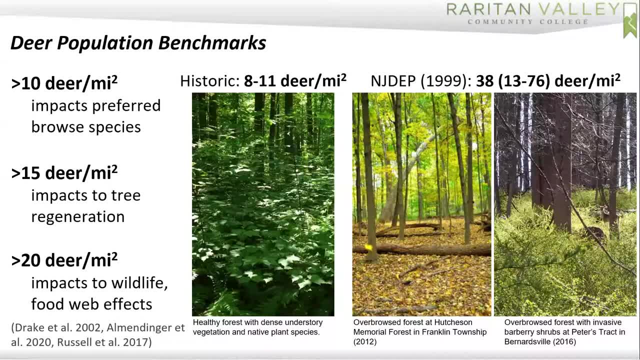 diversity and density. unfortunately, the populations that we see in new jersey today are far above those historic levels that we saw back in the 70s, and the sites that you see today are are what you see in the right two photos, with either: nothing growing in the understory. 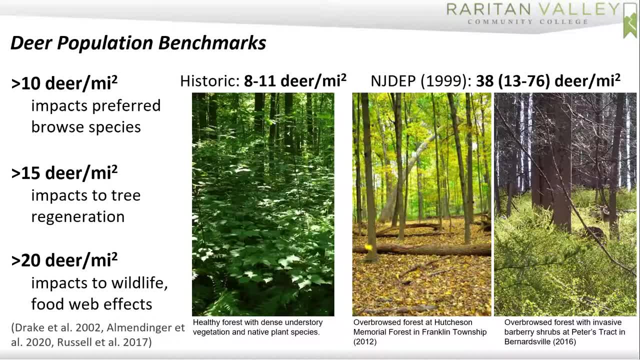 or a diversity, or say a richness of invasive plant species um filling that void that the deer have created. the last statewide population estimates for deer that were published by the state government were conducted in 1998 and they determined that there was an average of 38 deer per square mile, roughly four times the amount of deer that we need for everything to. 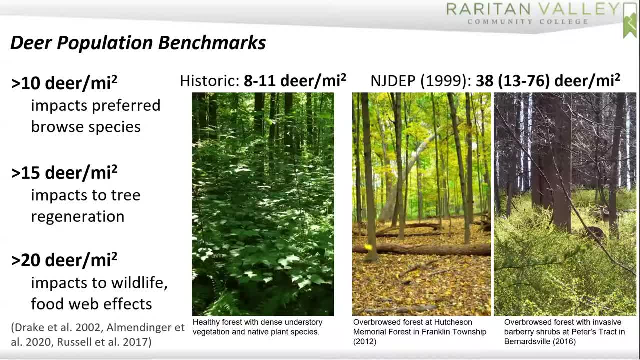 be in balance in the forests, but it was uneven. uneven across different parts of the state, with the pine barrens in south jersey supporting only about 13 deer per square mile and the highest densities occurring here in central new jersey, where our community college is located, of above. 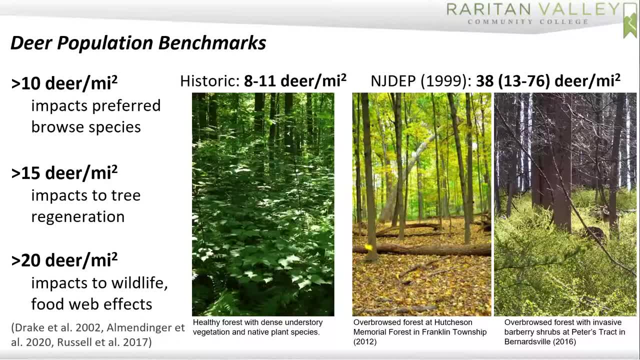 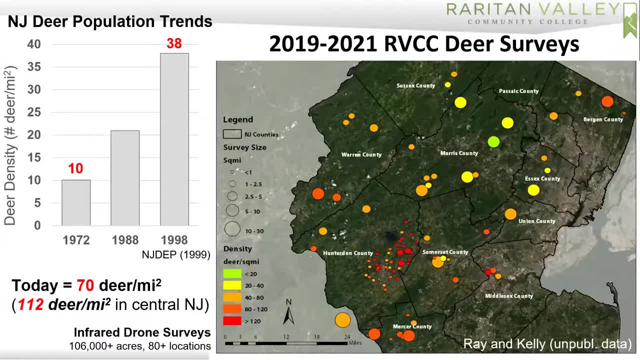 70 per square mile, but this is, you know, data that's 20 years old at this point and we've been doing a lot of research for the past few years to identify current population densities in the state, at least in the northern half of the state, using thermal sensors mounted to drones, which 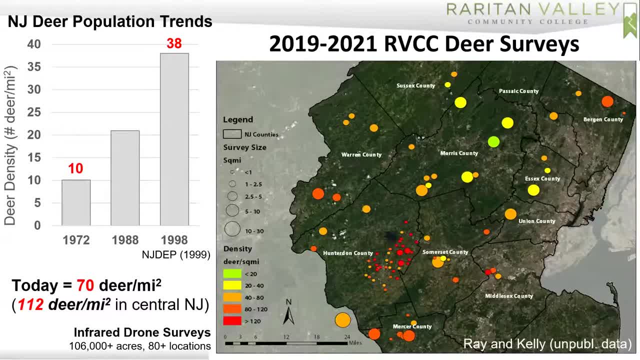 provide the most accurate measures of deer populations in the landscape, and so the historic data you can see in the photo on the top left of, with deer populations increasing from 10 to 38 by 1998. today, the average deer density in northern new jersey is 70 per square mile, and in central 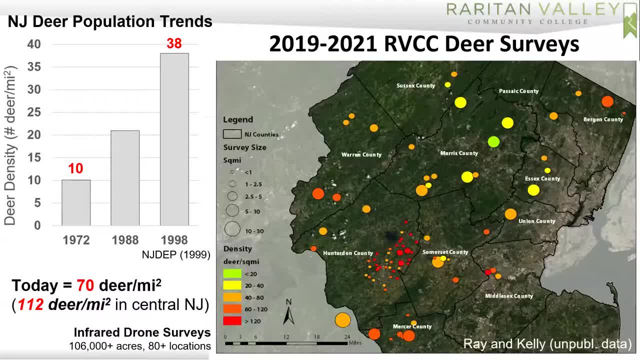 new jersey, where you know, 20 years ago- it was in the 70s, so the average deer density in northern new jersey is 70 per square mile, more than 10 or 12 times the the amount of deer that are needed again for everything to be in balance in the forest and for 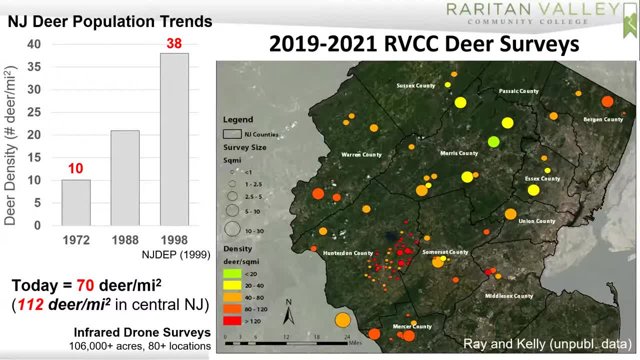 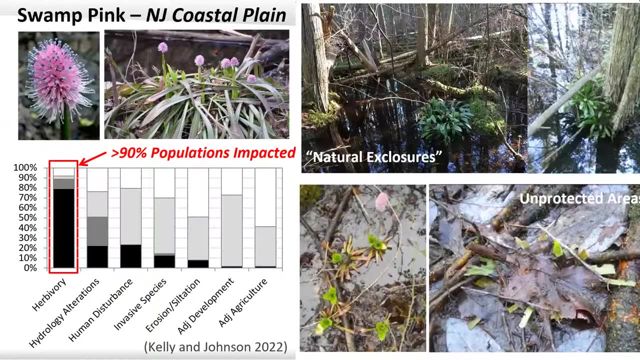 forests to support the full suite of plant and animal species that we all want to see around today and into the future. so this presents a real challenge for us at a really broad regional level. we didn't collect data from south jersey, but we've seen impacts for a lot of the species there as 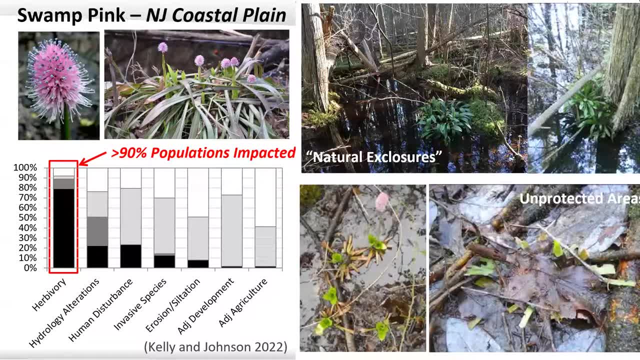 well, hubert was mentioning some of these in the early competition about species of the year. swamp pink is a perennial, evergreen lily species in the atlantic white cedar swamps and shrub swamps of the coastal plain primarily. we did comprehensive surveys of swamping populations around 10 years ago and found that 90 or more had been impacted. 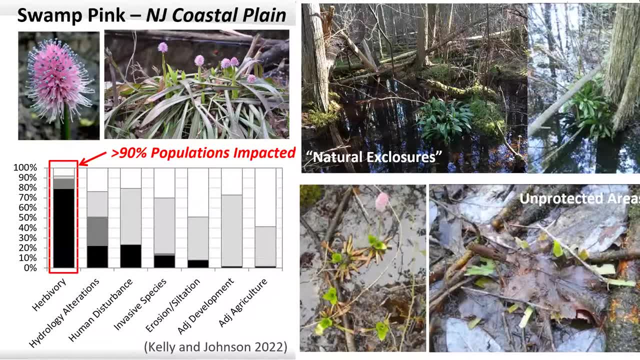 by direct signs of deer brows, and really the only places where swamp pink was thriving were in areas that we refer to as natural exclosures, where the basal rosettes of the plants had been protected by mucky waters that the deer, they provided a barrier for deer movements, and anywhere that 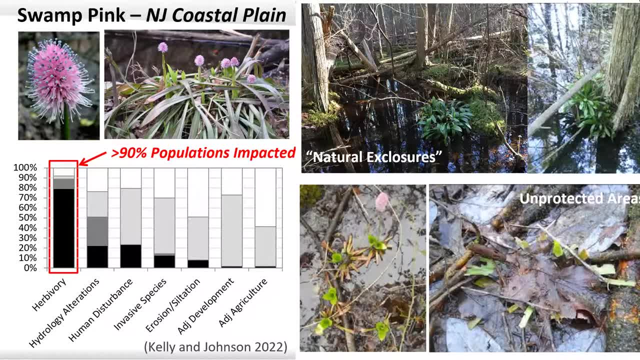 the plants occurred on the mainland areas adjacent to the rivers and streams where deer had access. we saw them being browsed to the ground and you can see some photos of what that looked like in the bottom right. so these are some of the signs that we're talking about of the preferred browse. 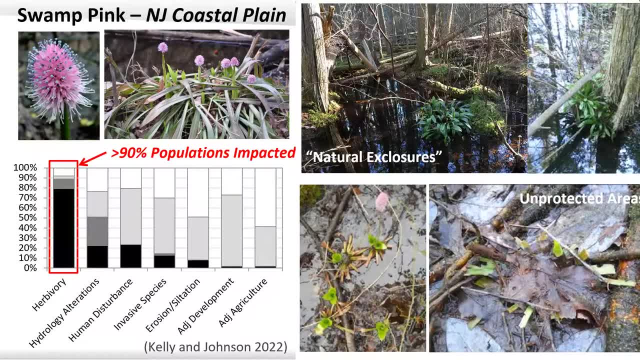 species suffering impacts from deer, and this is the place in new jersey where the populations of deer are at the lowest, and so if that's what's happening in the pine barrens, you can imagine what that means for these kinds of preferred browse species in northern new jersey. 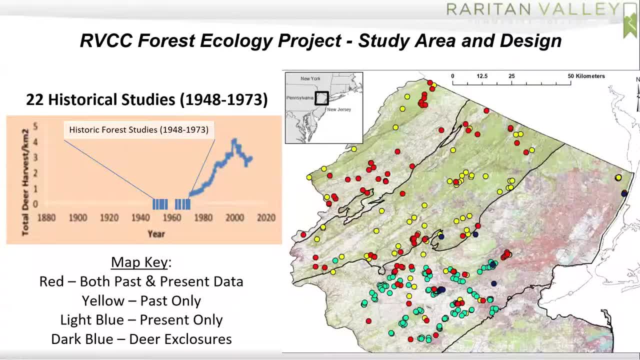 they're just already gone in most parts of the state. so in addition to looking at individual species like that, we've been doing kind of comprehensive surveys of forest structure and composition in northern new jersey, following in the footsteps of rutgers researchers, and we're really fortunate to have a rich data set from rutgers forest ecologist that goes back to the. 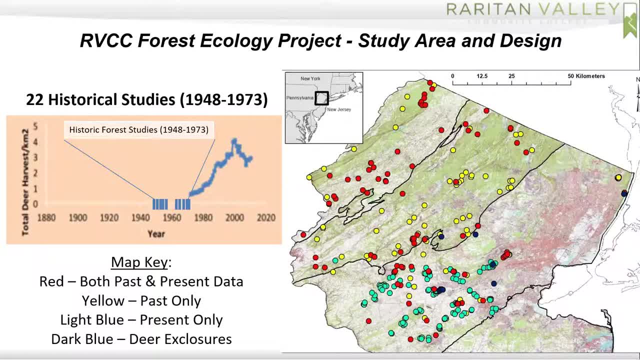 1940s. murray buell, in particular, set up shop in 1948 and he and his grad students in the next 25 years documented forests across central and northern new jersey and we're really fortunate to have that data set in front of us so that we can look at that, and we're really fortunate to. 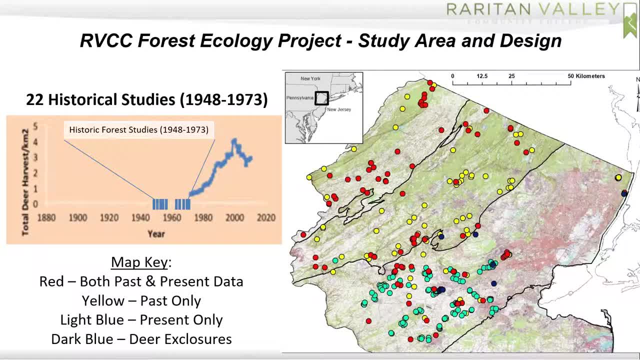 be able to look at this data set, and the data set and the data set that it has is really important to us to be able to see what it looks like in the forest in the past few years, and so we've been looking at that data set in the past few years and we've been looking at it in new jersey, looking at 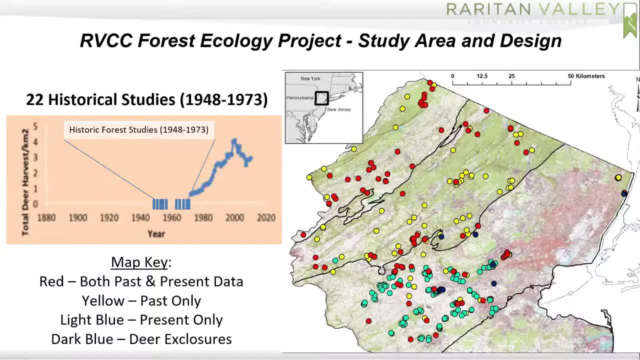 basic conditions and plant diversity and density and structure, and so we tried to identify as many of those exact locations as possible and recollect the data that they had collected during that time period. and the beauty of this data set that for us, is that all that data that 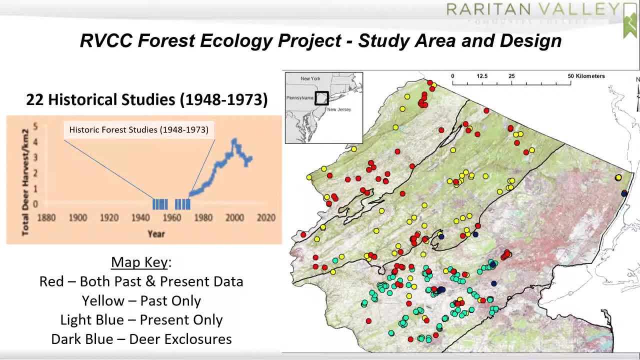 murray buell and his students collected was prior to the deer population explosion that we've seen in new jersey, so it's an invaluable reference data set so we can see exactly how our forests have changed. So all the red dots that you see on the map, there are places where these historic studies were conducted and we were able to identify the location and follow up with present-day data. 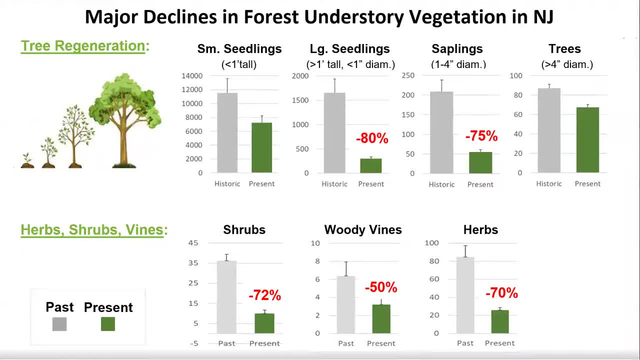 And the short of it is depicted largely in this slide. We saw major impacts to tree regeneration. in particular, The small seedlings did not show major signs of decline, even though it looks like that in the bar graph. And in each of these figures you can see from left to right, the historic data set is in the gray and the same site study today are in green. 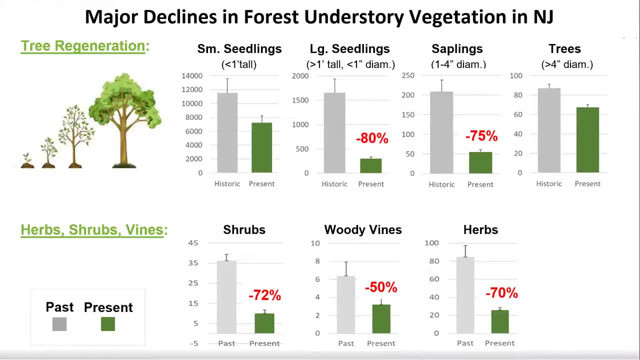 And even though it looks like there's changes in small seedling levels, those numbers are replenished every year from seeds raining down from the canopy, And they're inherently more variable because they're responding to precipitation and massing of the different tree species. 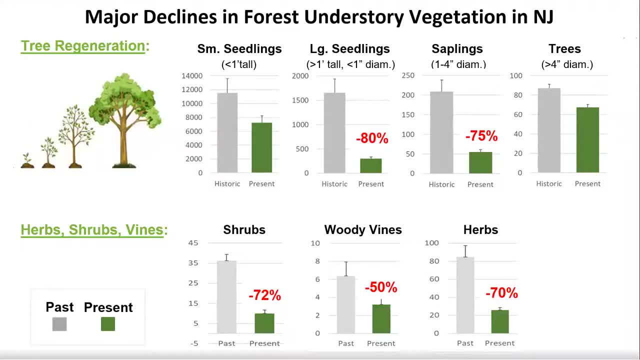 The problem is that those small seedlings rarely survive into larger size classes. So the next graph that you see here- we see in the top center- are the large seedlings that are more than a foot tall. We saw 80% declines in the densities of those large seedlings and that translated into 75% declines in the next size class. 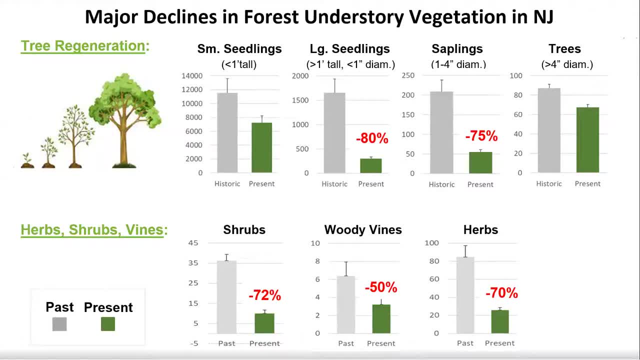 And the concern is that, if these trends continue, we're going to start to see these declines translating into actual reductions in canopy trees as well, because the trees aren't going to live forever And, with the increased mortality that we're seeing from storms and invasive pests and diseases, there's a real deficit in the understory of young trees that are waiting to fill their ranks. 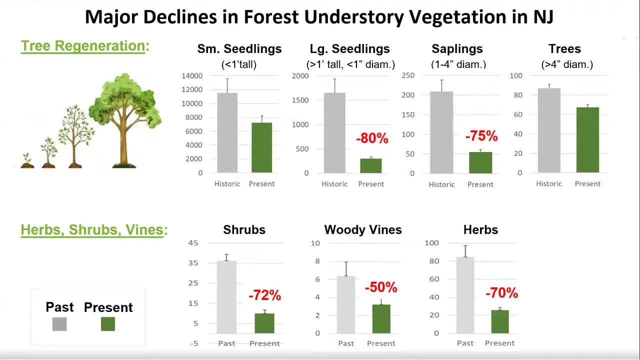 And if these trends continue, we're going to see a decline in the density of those large seedlings And if these trends continue, we're very likely to see forest losses taking place. in much of northern New Jersey, We also saw declines in other categories of understory vegetation, including the native shrubs, woody vines and herbaceous plants, which we lumped together everything from wildflowers to ferns, grasses and anything that was non-woody. 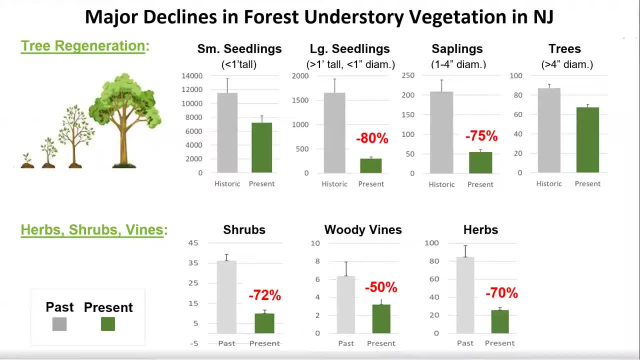 And so you know, we're seeing 50 to 80% declines in almost every category of understory vegetation, which is really catastrophic for the species that are depending upon them, not just the plant species themselves. There was variation regionally in the state, and deer are an edge species, as I mentioned. 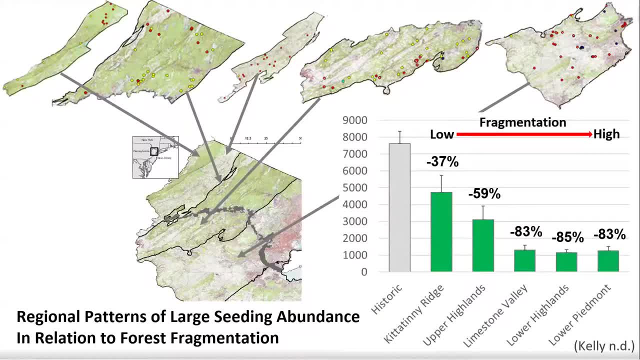 And so the places that have the largest, most intact forests. in the northern highlands, above the glacial moraine and the Kittatinny Ridge, we saw the least amount of declines of tree regeneration. But there were still worse, significant declines even in those places where the forests were most intact. 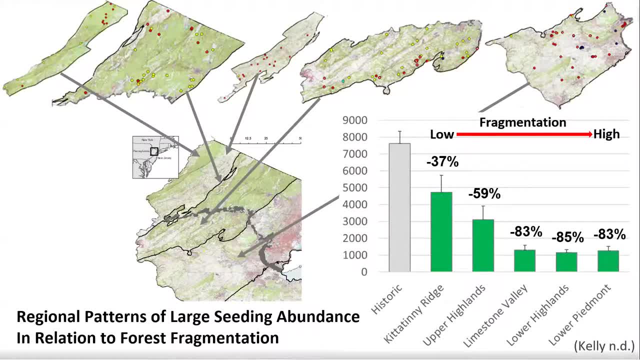 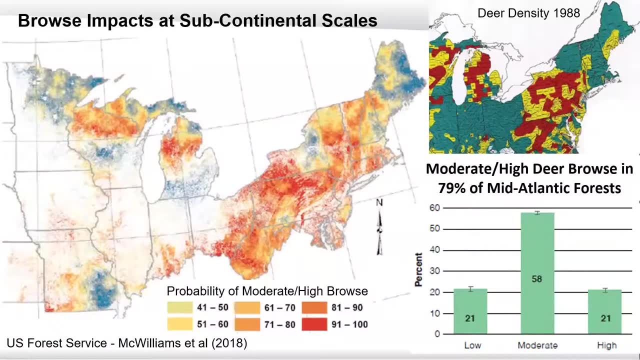 The places where forests were most fragmented, in the areas that historically had been used for agriculture, had the greatest amount of vegetation. They had the greatest amounts of regeneration deficits, And these phenomena really extend far beyond New Jersey. This is not just a continental phenomenon, but really a global phenomenon at this point, because we've successfully, unfortunately- eradicated predators throughout much of the planet. at this point, 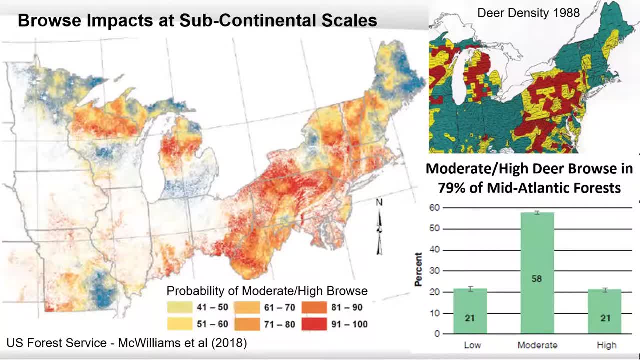 And so white-tailed deer are increasing throughout much of the range in eastern North America, In the western parts of the continent. you can see other deer species increasing, with research from Vancouver Island and elsewhere showing impacts. You can see other deer species increasing, with research from Vancouver Island and elsewhere showing impacts. 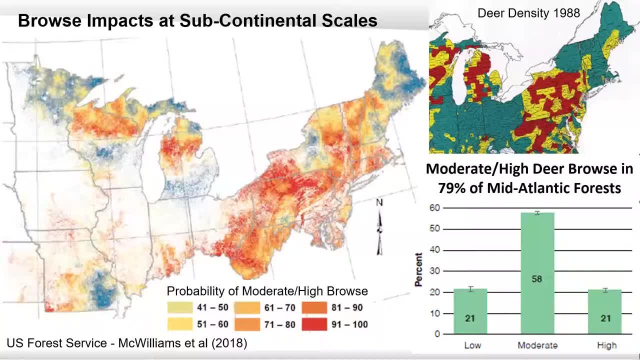 For instance in the United States, as I think the sprawling woods are increasing. You can see research from Japan and Europe and pretty much everywhere that there's large ground-dwelling herbivores. Their populations are increasing. we're seeing a forest decline as a result of um excessive population levels. 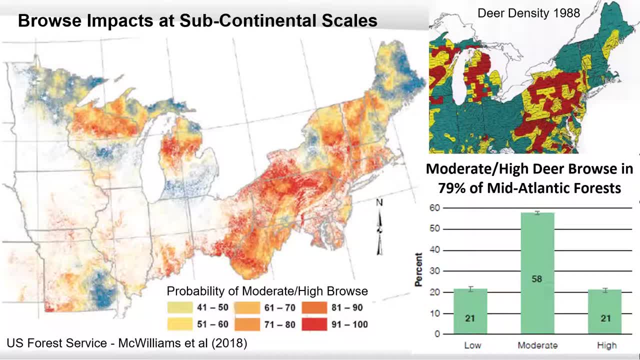 And so again you can see how the regeneration deficits and the increased browse severity is the greatest in the mid-Atlantic region where we're located, according to the US Forest Service here, And that corresponds really closely with the areas with the highest deer densities from that earlier study from University of Georgia. 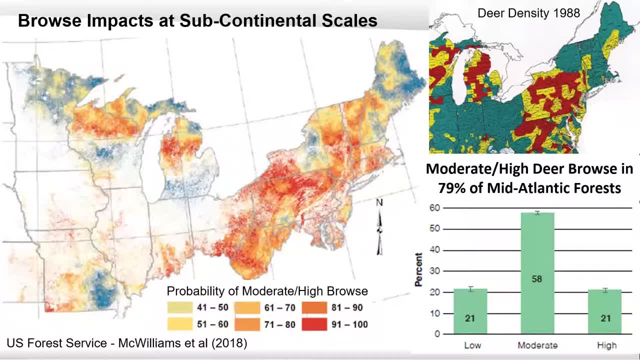 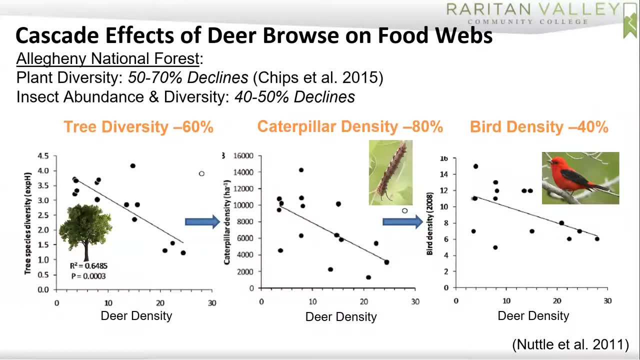 percent of our forests in this region are suffering from moderate to severe levels of deer browse. as i mentioned, the decline in vegetation translates into declines of the other species that depend upon them, and you see these cascade effects or trickle down effects through the food web. a cascade is another word for waterfall, and so it's a very large trickle. 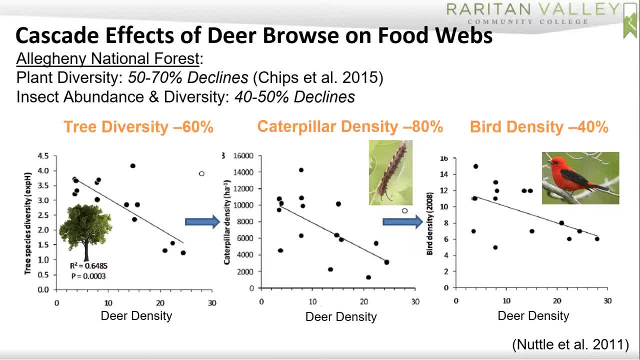 so to speak, and there's been a lot of really good research from the allegheny national forest in western pennsylvania documenting these kinds of cascade effects, using deer enclosures where they kept captive deer at different densities to see how the forest responded to those variable deer. 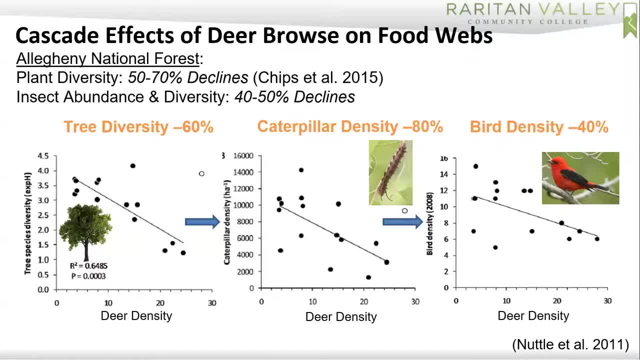 populations, and what they found was that as deer populations increase, you see declines in tree diversity, which translates into declines in caterpillar density, and after hearing dr talamy's talk this morning, i'm sure that should be no surprise, given the diversity and specialization of these uh lepidopteran. 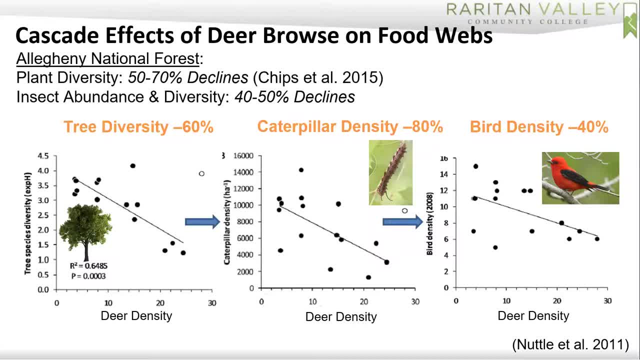 on the particular species that they depend upon, and the caterpillars are the preferred food source of many bird species in the forest. most of our forest birds are insectivorous, at least at certain stages in their life cycle, and so the declines in caterpillars have translated 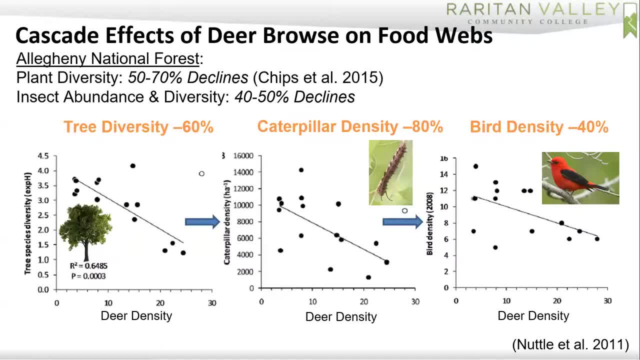 into declines in bird populations, the high end of the x-axis that you see here. these are in number of deer per square kilometer, but that trade translates into about the same levels of deer that we're seeing in northern new jersey on average today, and so in the allegheny national forest 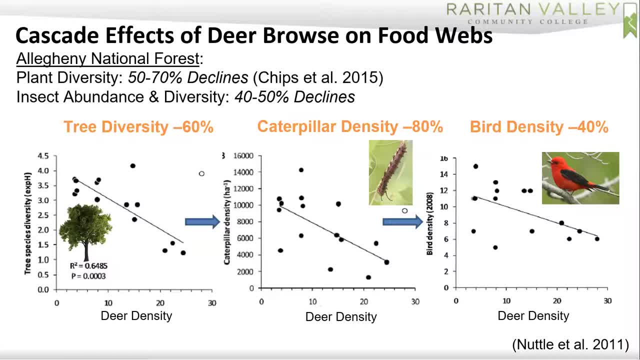 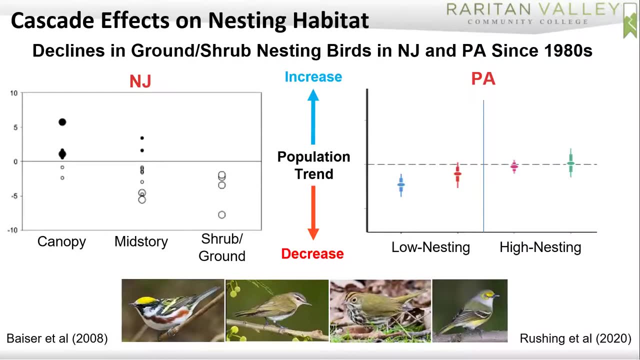 map we're seeing likely a definite change to their size, so it's a good sign for them to be in the high end and that is the state of the sun in new jersey, um, so if this is a field of deer- and we have a lot of deer in the west- thats what we're seeing as well. 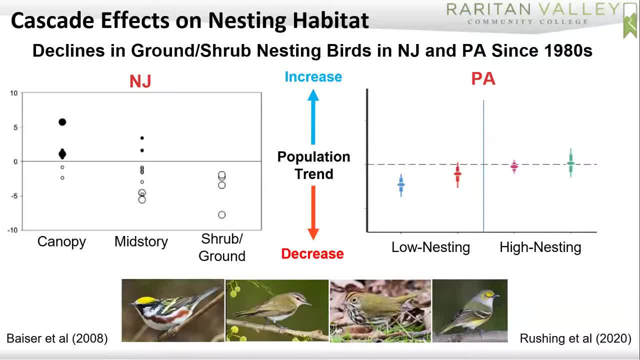 so in the area where we might see some verdeer deer and we would expect to see a certain kind of decline. so we're seeing a lot of um, and so the studies that have been taking place here in new jersey and pennsylvania in the last 20 years have shown predictably declines in shrub and ground nesting birds. so the study on the left 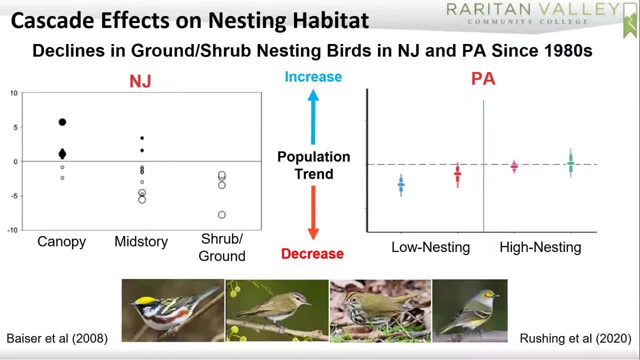 here is from the rutgers research forest and they looked at changes in bird populations since the 1980s based on where species nest in the forest environment, and each circle there indicates a different species and the large circles indicate significant changes. anything below the line is. 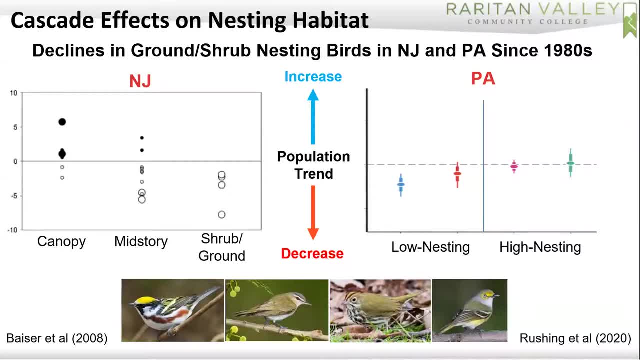 a decrease, and so you can see that 100 of the shrub and ground nesting birds in that forest had declined significantly since the 80s, and the majority of mid-story canopy nesters had as well. because we're talking about decades worth of deer pressure, that's translating into a deficit in the 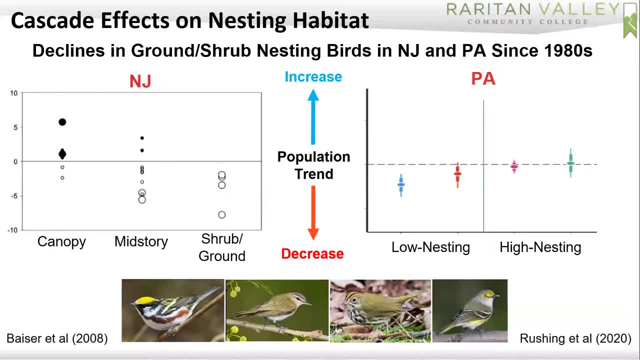 entire understory in many forests. that was just from one forest in new jersey but more recently, just a year or two ago, a study was conducted in with all of pennsylvania bird data showing more or less the same thing, panning out, with all of the low nesting forest birds declining significantly. 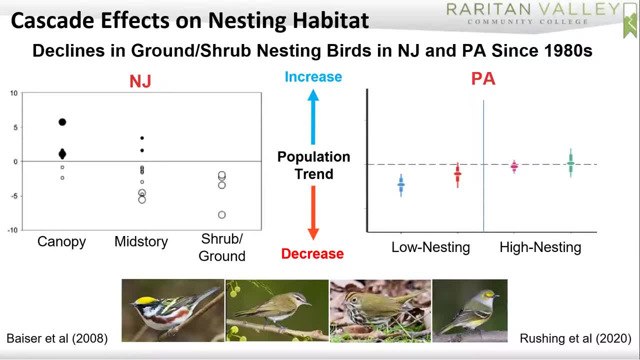 and the high nesting forest for is not showing any meaningful changes over time. other studies that have compiled data for the entire continent by rutgers and other researchers have shown this to be more or less consistent across that entire range. so again, this is a global phenomenon. it's 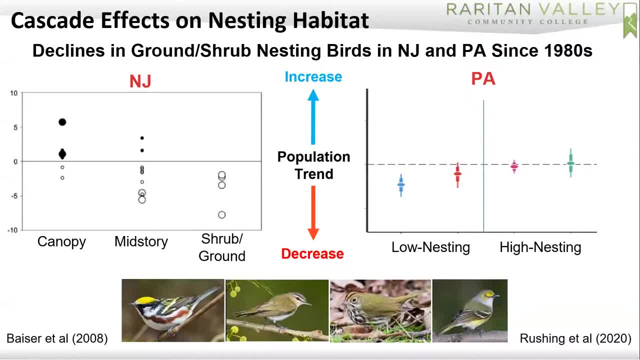 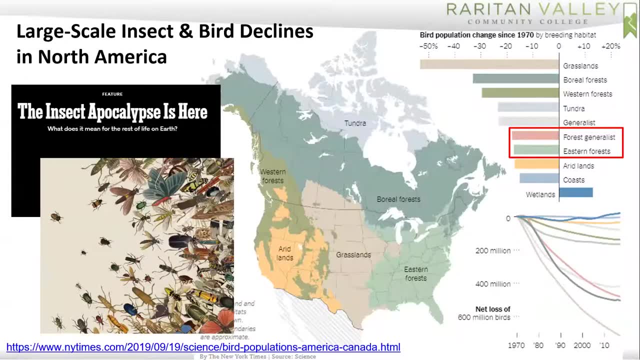 not just happening in locally here in new jersey or at the state level, and this is certainly a factor for many of the large-scale declines that we're seeing globally, both for insects and for bird populations. so there's been a number of major studies in the past few years documenting really catastrophic declines in insect populations. 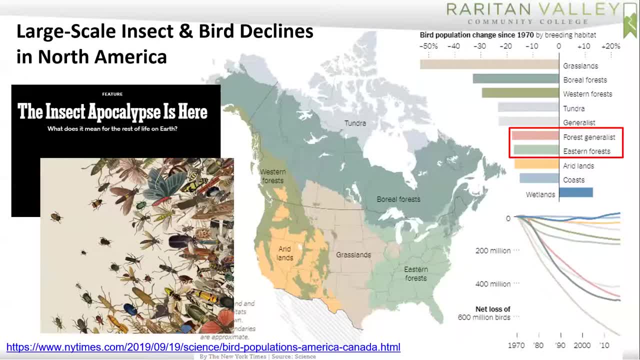 in europe and north america, as well as birds. since the 1960s and 70s, and while forest birds haven't declined as much as some other bird species, they have experienced about 20 percent declines, and there are many reasons for that, including loss of wintering habitats. 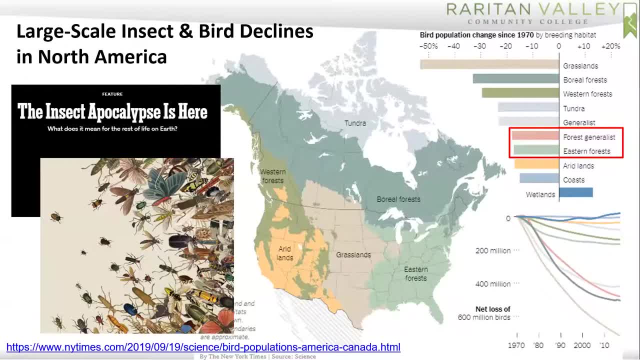 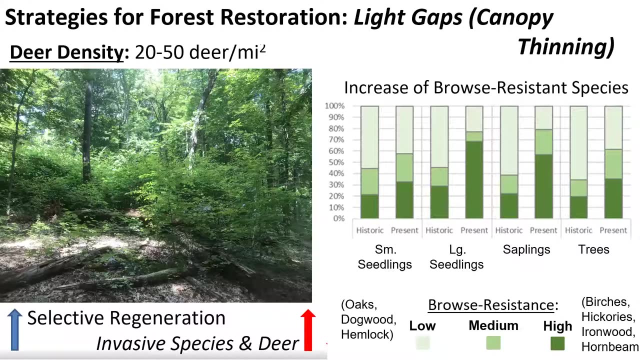 pesticide exposures, all sorts of things that are impacting birds and insects, but clearly this is a major factor that's contributing to these widespread declines and unfortunately, it isn't given the same attention as some of these other more conspicuous factors. so, in terms of strategies for addressing these sorts of problems, 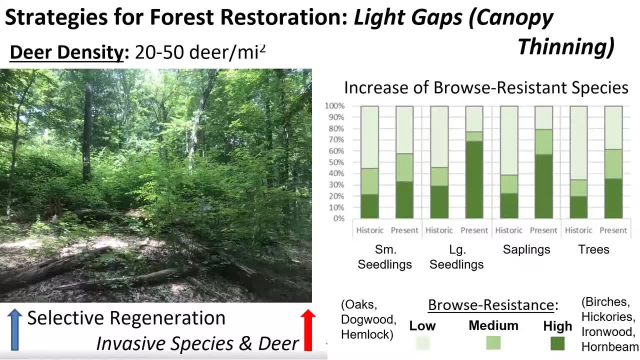 the one of the places where regeneration historically was most obvious were in light gaps, as a tree would fall in the forest. it creates increased light conditions that favors tree growth. trees and other plants typically grow faster when there's when they're exposed to more light. as i'm 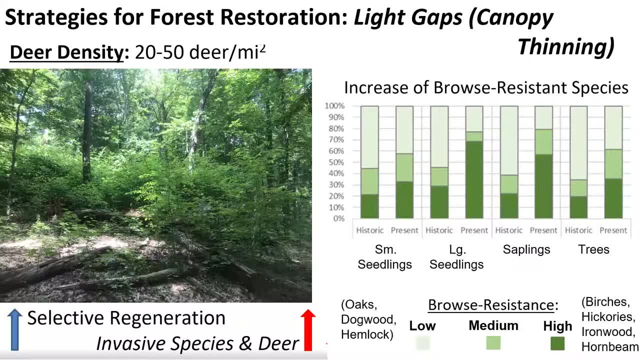 sure you're aware, and so in those light gaps you tend to find much denser and more vigorous regeneration, and so, because of that, one of the measures that are traditionally used to increase tree regeneration in forest environments is canopy thinning. many foresters will use such prescriptions to you know. 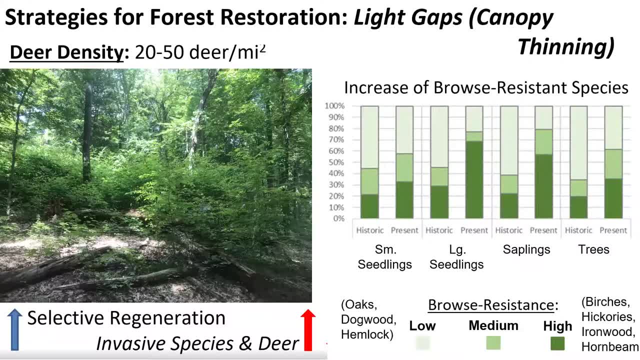 stimulate tree regeneration and understory growth. and if you have moderate to high deer populations- about 20 to 50 per square mile- you can still see that sort of regeneration taking place in new jersey with with vigorous growth in those light gaps in the forests. the problem is that the deer 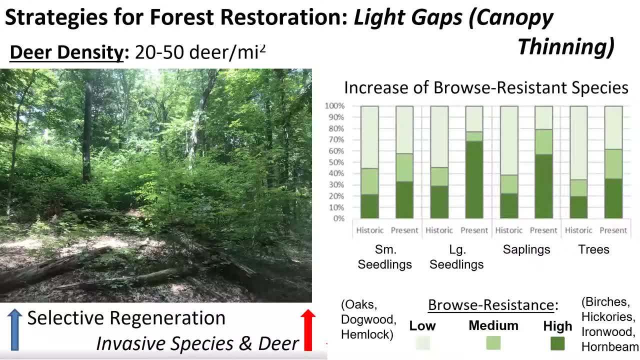 are still there and they're selectively removing the things that are tasty and they're not going to be tastiest from that, and so certain species like oaks and dogwoods and hemlocks are going to get removed from that growth and you're going to get the growth favoring. 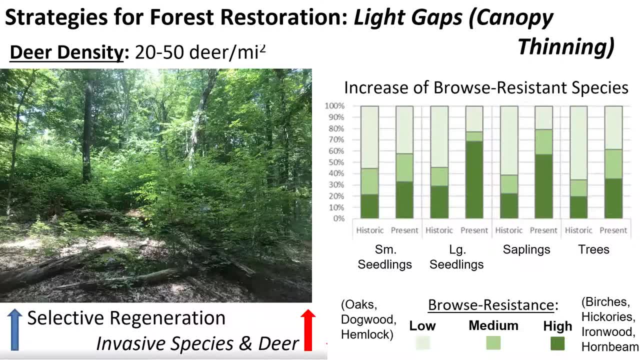 the species that are least palatable to deer, like hickories and different birch species and so forth. and so we saw, in our comparisons of past to present forest conditions, dramatic changes in species composition in our forests, with this shift to increased abundance of the species that are least palatable. and so, while oaks are really important for so many, 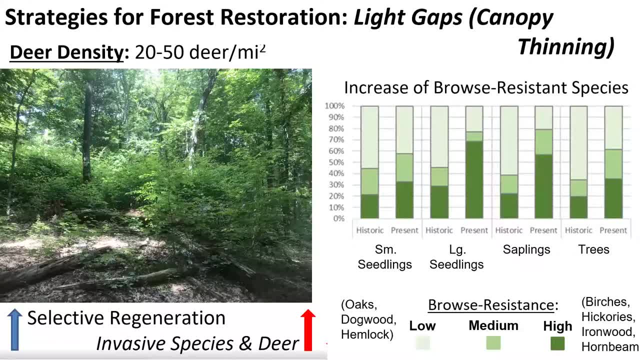 species of animals in general, and i just wanted to close a little bit out of today's talk and also let you know that, in many ways, dare to do what i think is the best way to do so, and so you can see that, even though the species that are least palatable in the forests are, 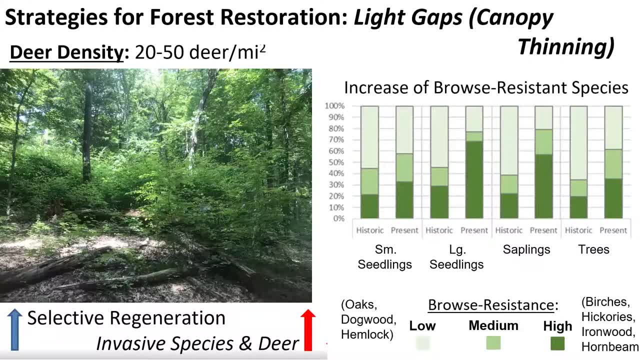 more soимone of the most palatable species: moths, butterflies and many others that depend upon them. they are some of the most preferred species that deer like to eat, and so if we're interested in increasing oak regeneration, it's really important to tackle deer as a part of that. 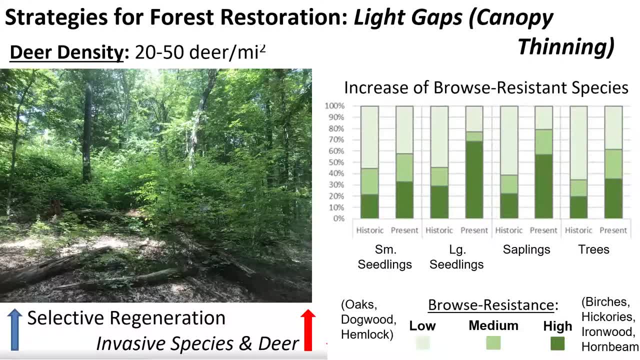 forest and growing, and the growth does provide additional food for deer, and so if you're not simultaneously managing deer while you're using canopy thinning, you're actually going to make the deer problem worse, because you're feeding deer populations and canopy thinning traditionally has been used as a as a main tool for deer management throughout the region. for folks that are trying. 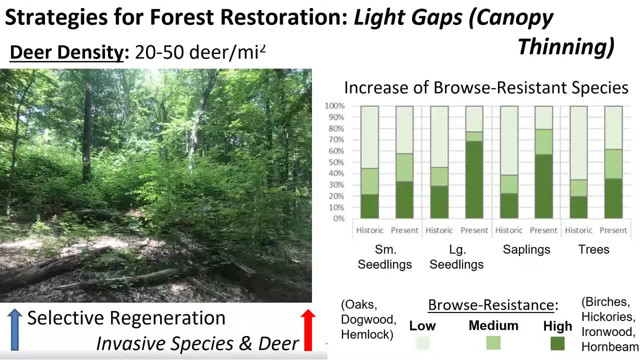 to increase deer populations. canopy thinning is a really great strategy because you're going to increase food sources on the forest floor to support deer population growth. so that's at you know: moderate deer levels of 20 to 50 per square mile. as we talked about deer, many of our 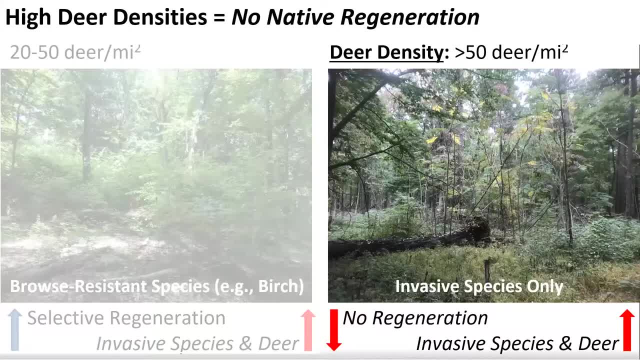 forests have many, much higher levels of deer at this point and when you get into those kinds of situations, you don't get any native regeneration at all. if you look at light gaps in places like Washington Valley Park and many others in central New Jersey, the light gaps are just full of nothing. 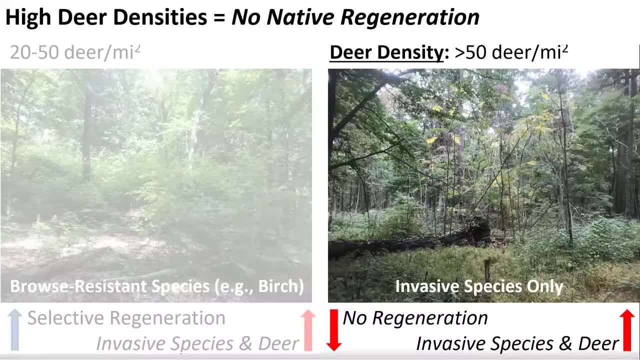 but invasive species. so there's no young trees growing up in the ways that we would expect to see or historically did see, instead, what you find in this image. here you can see Japanese angelica tree, but it's really a shrub. coming up. beneath that you've got Japanese wineberry and on the 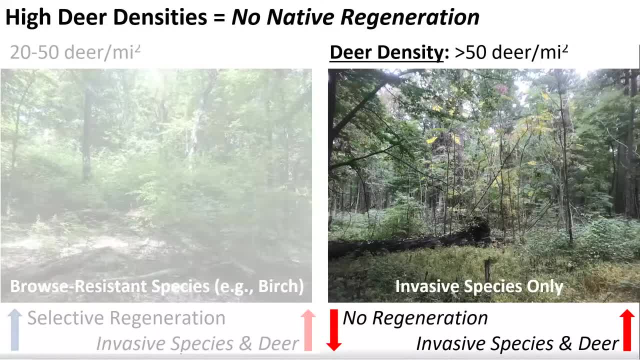 forest floor. it's a monoculture of Japanese stilt grass, and so if you have these really high deer populations in the area and you use canopy thinning as a tool, you're actually going to be really potentially irreparably harming these forests by stimulating invasive plant species. 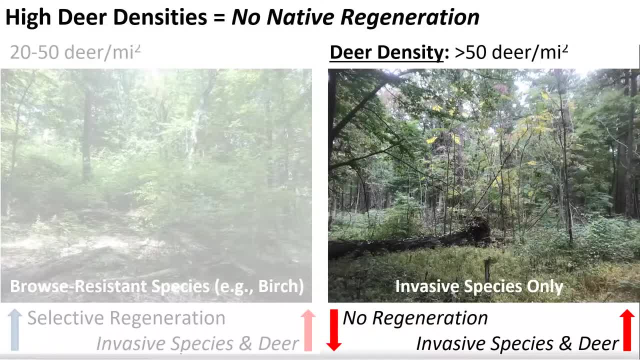 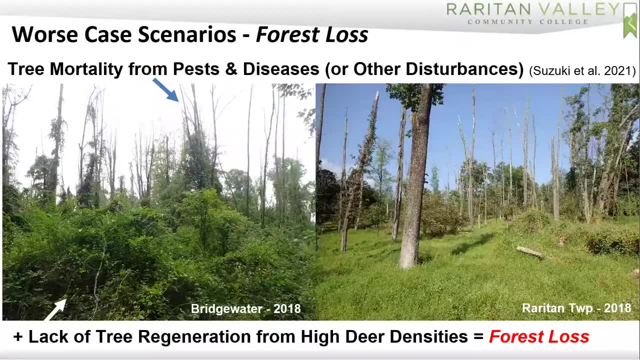 growth, you're not going to get benefits for native regeneration at all and you're still going to be supporting increased deer populations because the deer are going to be removing everything from that understory that's native, that's growing. the worst case scenarios are when you combine these severe deer population levels and lack of 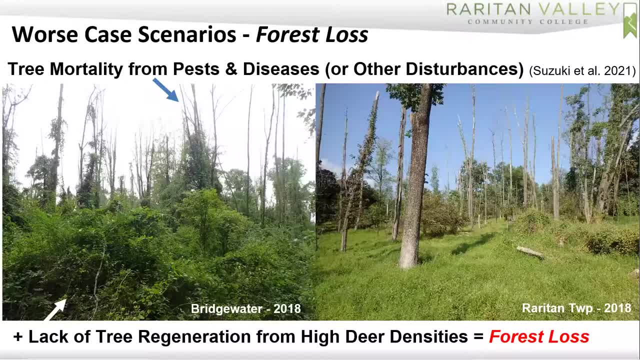 tree regeneration with the other kinds of impacts that are happening to forests, whether it's severe storms from climate change or invasive pests and diseases. so in our area we're seeing widespread devastation of forests, from emerald ash borer, for example, and ashes were really important in. 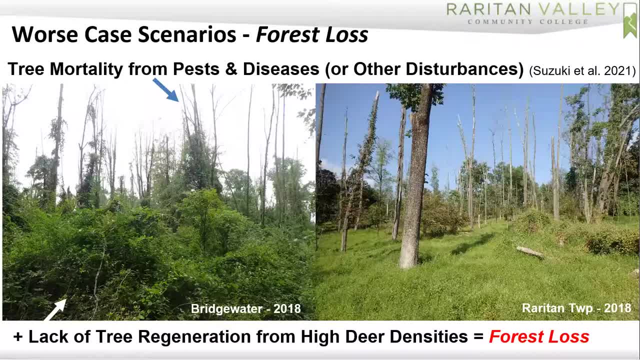 important for recovering forests and post-agricultural soils, and so in many of those places where forests have regrown as farms were abandoned, you see really low densities of trees, with ashes being one of the dominant trees, and as they disappear from emerald ash borer, what we're seeing is the forests are not recovering. 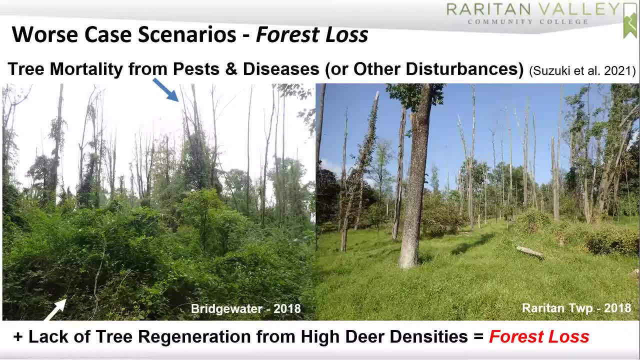 from that um event. instead, what you get are- on the left, here is an example from bridgewater- a thicket of invasive shrubs and vines. or on the right, here, an image from raritan, where there are nothing but herbaceous wetland plants or invasive species to replace them. and so, if these trends continue, 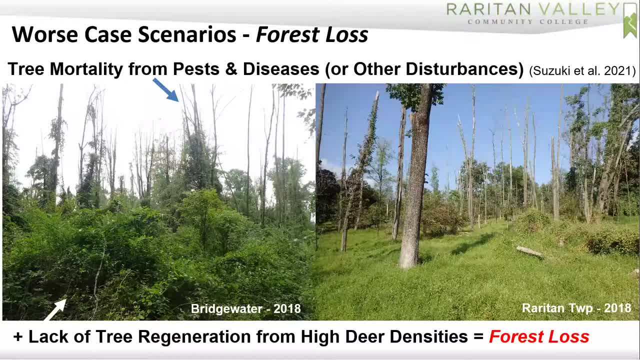 again and we have continued impacts from uh, pests and disease species affecting our trees or increased severity of storms, we're going to begin to see forest loss taking place in much more widespread areas in the state if we don't address this fundamental problem of elevated deer population densities. so this is clearly a priority for future forest restoration. 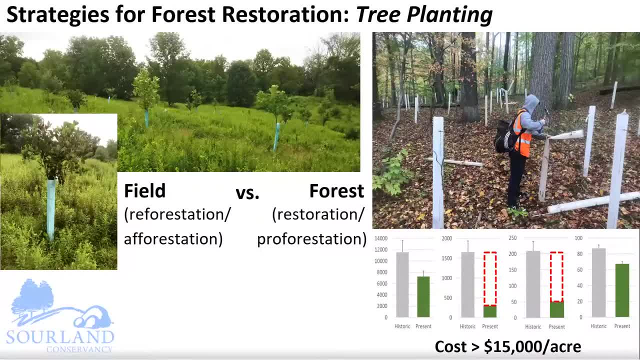 and conservation. one of the other strategies that's really popular, especially right now when everybody's interested in planting trees to combat climate change, is tree plantings. everybody loves planting trees, it feels good, it's a wonderful thing to engage in, to do, but depending on what trees you're using and what the situations are, it might have varying degrees of effectiveness or be 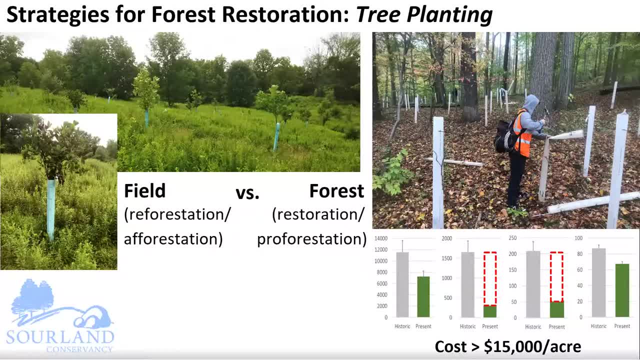 in some cases counterproductive. So if you're using trees to return forest to an area through reforestation, or what's sometimes referred to as afforestation, this can be a really beneficial measure to kind of accelerate the rates of tree colonization into open farm fields, for example. 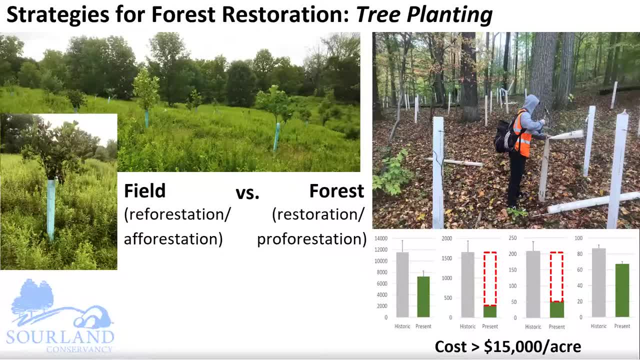 whether it's along a stream, buffer or any other area you're trying to get a forest to return to. It's beneficial because then the trees get a foot up above the, competing with the herbaceous plants which grow really densely and vigorously that they'd otherwise have to compete with. 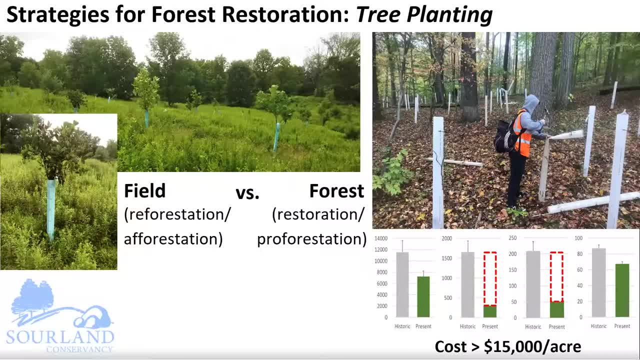 And many tree species, especially the large nut-bearing species like hickories and oaks, tend to disperse less readily than the wind-dispersed species. So if you're trying to get oaks and hickories or other large nut-bearing species to grow, planting the trees themselves. 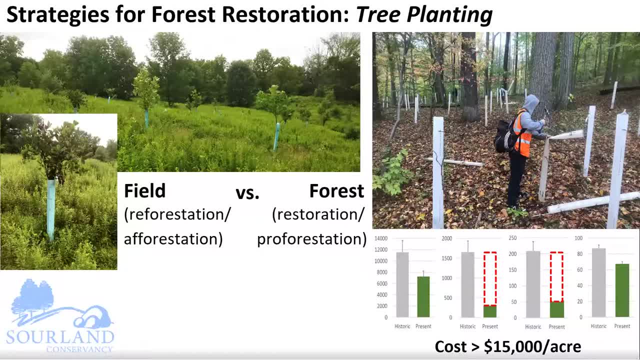 is a good way to get that started, to accelerate that recovery. Planting trees in forest environments doesn't necessarily make as much sense, because the trees are already putting far more seeds and seedlings into the landscape. We can actually predict exactly how many we should be planting to restore the understory. 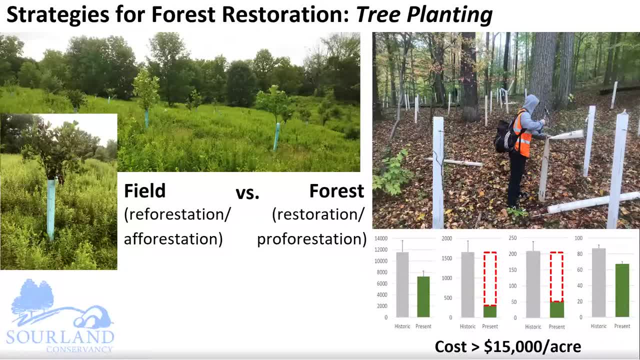 conditions there and what the costs of that would be, And that translates into more than $15,000 per acre if you're going to actually replant all the large seedlings and saplings in the forest that are no longer present, And that's not really feasible for us to be doing. 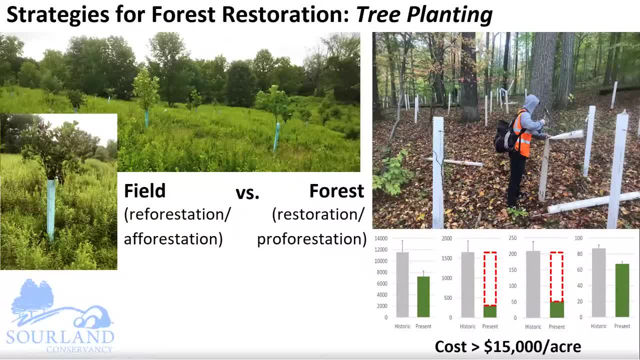 at the scales at which we need to to restore our forest understories throughout the state, And so right now we're actually partnering with the Powerlands Conservancy to do some research to figure out whether planting trees in understories and protecting them from deer even yields any kind of success in terms of tree survival and growth. 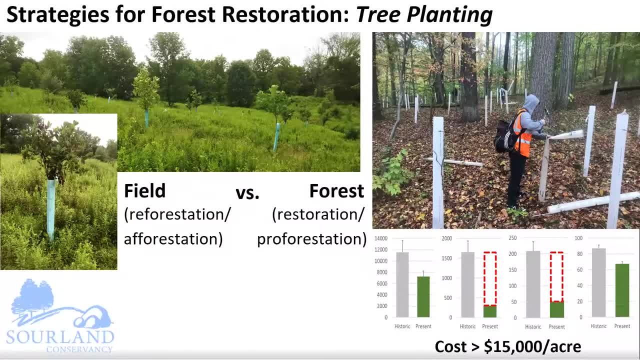 and also comparing that to putting these sorts of deer cages around native seedlings that are regenerated on their own, So the seeds that are sprouting and germinating naturally. we also protected some of those and we're going to be comparing their survival and success over the next couple years to see what the relative benefits of those two strategies for. 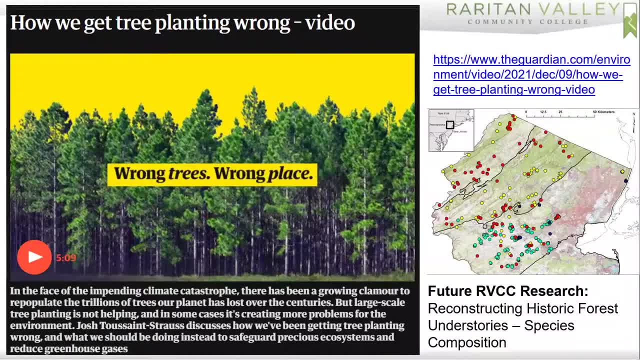 forest restoration are. There was a recent video that was put out by some researchers through The Guardian. if you're interested in some of these concerns about large-scale tree planting efforts and some of the nuances related to that, It can be really beneficial in combating climate change. 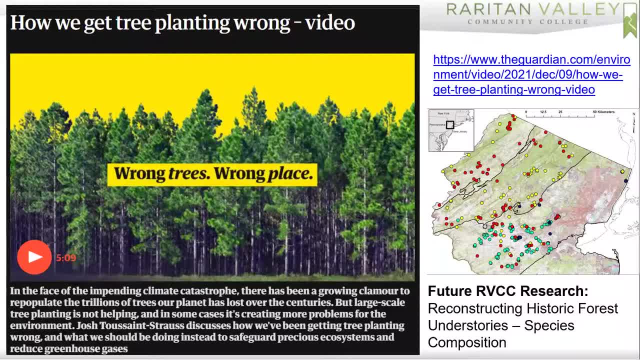 or for forest conservation efforts, but it also can be counterproductive, as I mentioned, and so that's a pretty good primer on some of the issues that are involved, from around the world where people are planting billions of trees right now to try to combat climate change. 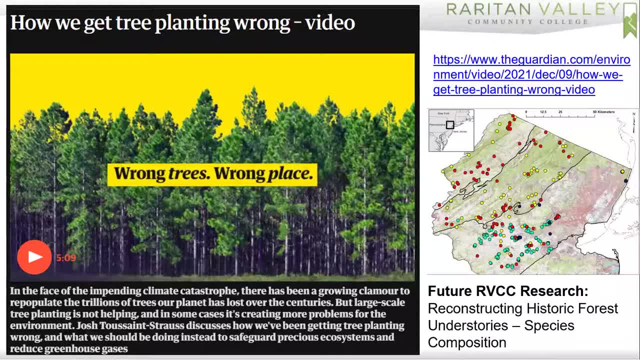 And to try to inform these efforts in New Jersey. since we have this historical data set that we've compiled. in the next year we're going to be trying to produce some materials that can help inform these efforts locally. So if people are interested in planting trees in the Sowerlands, 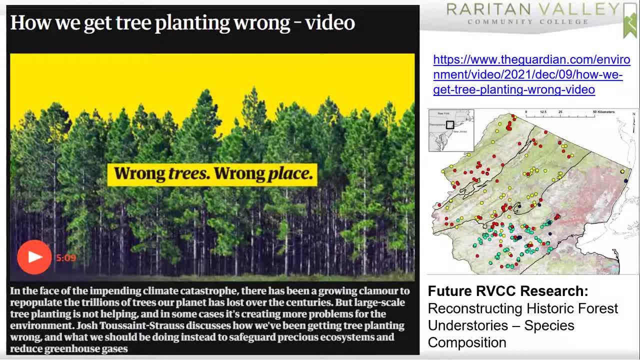 or the Piedmont or elsewhere. we can refer to these historical data sets to see what kind of species are most appropriate to those situations, whether it's trees or other understory species that might be of interest, And so hopefully we'll be able to produce that sometime soon. 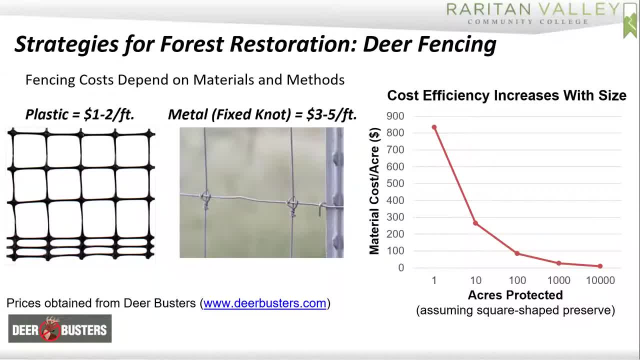 Since the trees are planting themselves and are far more effective at it than we are. a more cost-effective way of taking advantage of that is using deer exposures or deer fencing. Depending on what kinds of materials you use and how large the exposures are, they may be more or less cost-efficient. So typically, if you're using the cheapest kind, 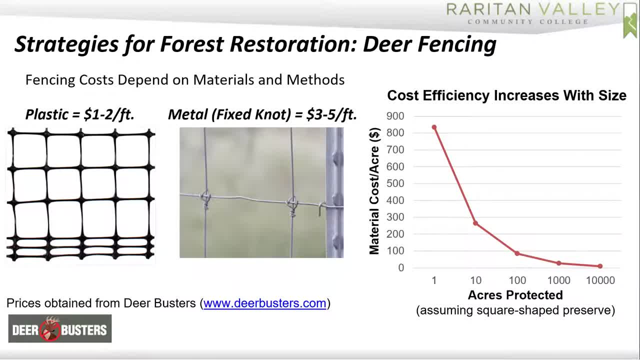 of materials and you're trying to protect about an acre worth of property. it'll cost between $800 and $1,000 for an individual acre to be protected, But because of the math that's involved, the larger the exposure, the cheaper it is per acre in terms of forest protections, And so when 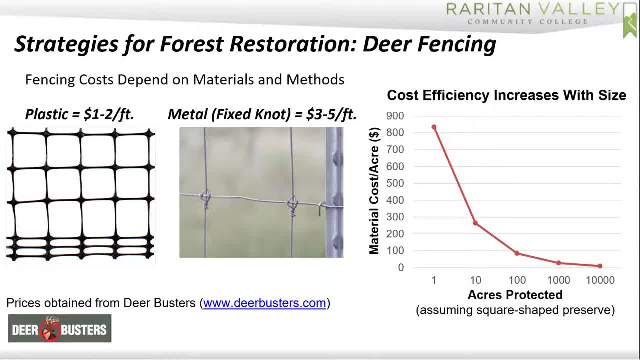 you get up to 100 or 1,000 acres that you're protecting with an exposure. you can see that they become much more cost-effective. But this is just the installation and just the material costs. You have to pay for labor, And then the other thing is that you have to make sure that the 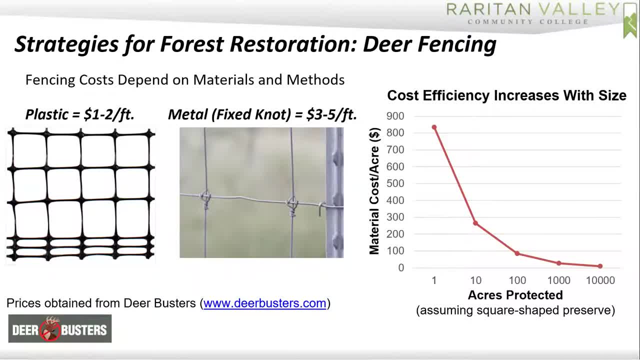 fences are maintained- And they need to be maintained for more than 10 years to have effective forest restoration take place, because trees are going to fall on the fence and bring it down, Deer are going to break through the fence And a number of other things can go wrong as well. 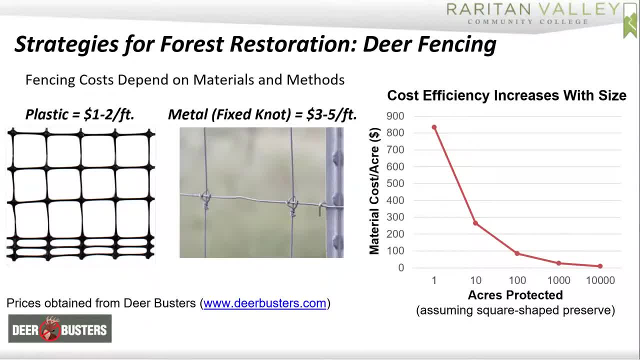 And if deer get in there, they can get trapped in there and can actually make browse impacts worse if they're not addressed right away, And so it's a really important restoration tool that can be very cost-effective at small scales, But it's problematic at really large scale levels because of its expense. 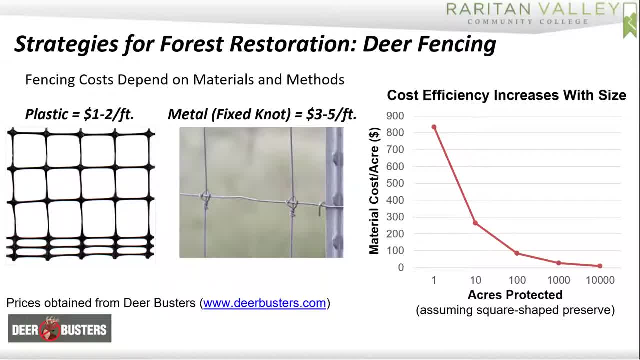 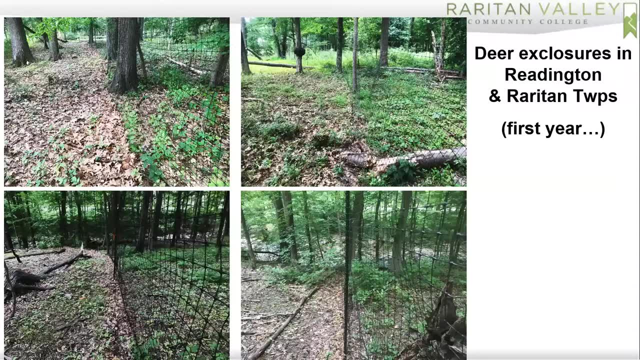 and the difficulties in doing this at the regional level that we have these kinds of concerns. But one of the nice things is when you put up a deer fence. usually the effects are almost immediate If there is a seed bank in place, even in the very first year after the fence is installed. 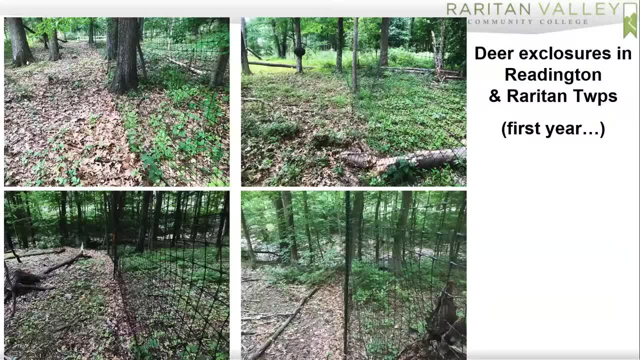 you can start to see the wildflowers bounce back and tree seed then start to bounce back really vigorously And the shrubs that might have been browsed to the ground are going to start to appear really lush and grow like gangbusters inside the fence compared to adjacent areas. 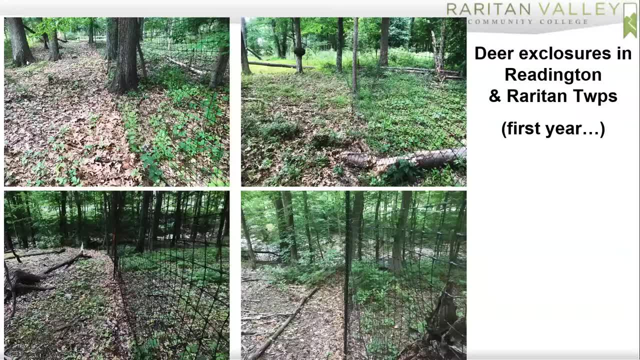 So these are just some photos from the dozen or so exclosures we installed in our area in the past few years, with really clear early signs. So you can see some of those early signs of success already taking place just in that very first growing season. If the fences are maintained over time you can look to some of our conservation. 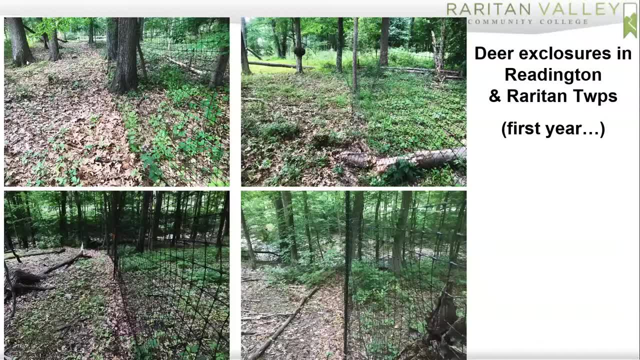 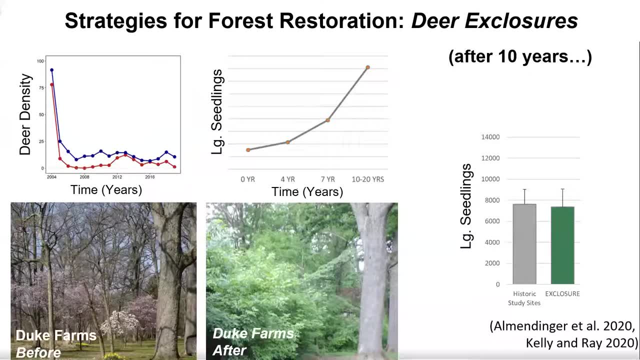 partners in the region that have had much greater foresight and have done this for decades now, In places like Duke Farms, where they reduce their deer population and have a square mile deer exclosure that they've maintained for more than 15 years. at this point you can see really clear. 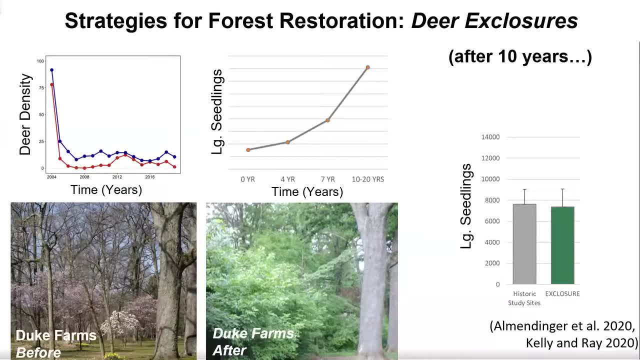 trajectories of tree seedling growth happening within those places, with the large seedlings in particular bouncing back to historic levels. So if you look at the next slide, you can see the growth that took place in young trees within Duke Farms and that's clearly one of the best showcases for looking at the impacts of deer management on forest recovery. 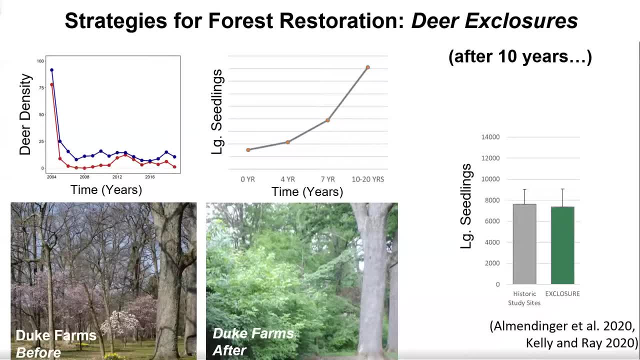 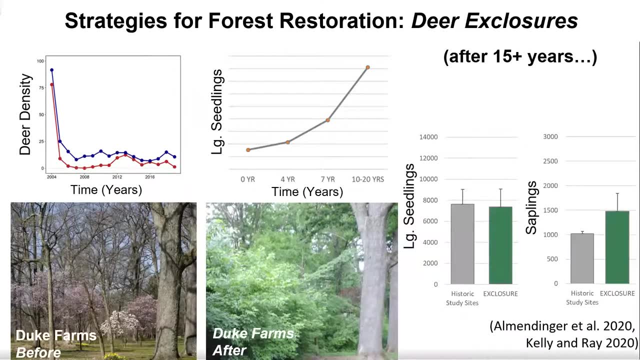 and regeneration within our area. If you keep those deer exposures installed even longer, you can start to see the sapling level layer recover as well. After about 15 years that next large size class of trees recovers and I would imagine in about 10 to 15 years longer you'd. 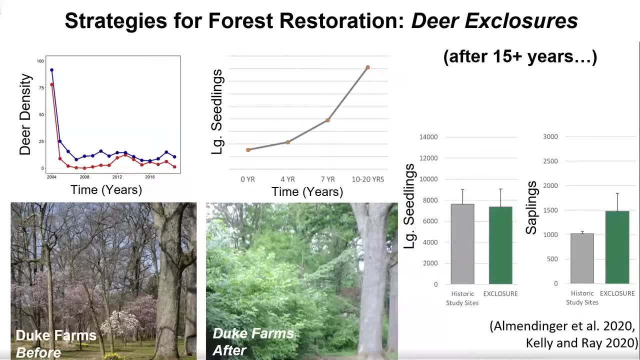 start to see recovery of the tree layers as well, And this is again doing nothing more than putting up a deer fence and maintaining it, with moderate levels of deer occasionally occurring within there, And this is a really clear indication that deer are the primary factor to address with tree. 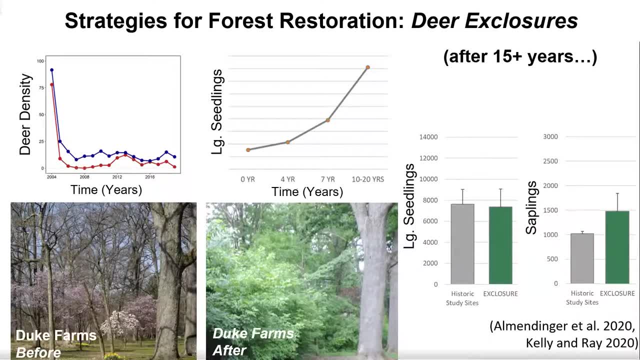 regeneration, because all the other factors that are impacting our forests are still occurring within these deer exposures. There's still acid rain and climate change and invasive pests and diseases. There's trails and human disturbance. There's invasive species And yet, despite all those things taking place in our area, if you just correct the deer part of the equation, you can see. 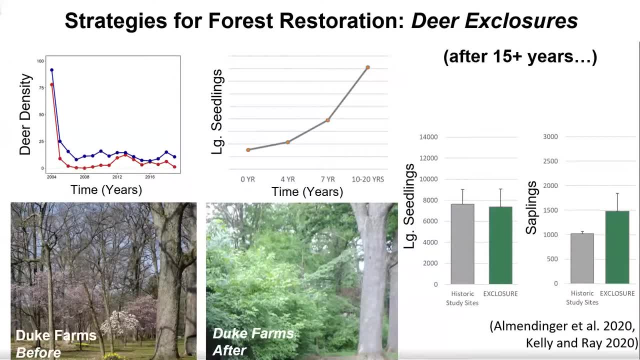 the forest respond really vigorously without any additional effort, And so there's some real signs of hope that we can have a better future for our forests, And I think that's really important. And then we also have a little bit of a difference in the species, So I think that's a really good 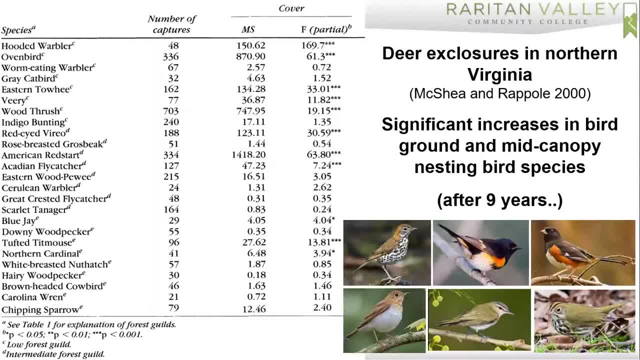 example of what we have to do if we really take this issue seriously. And then you can also start to see from some other research that's been conducted elsewhere in our region. This is a study from Virginia that found that after about nine years of a deer exposure being in place, 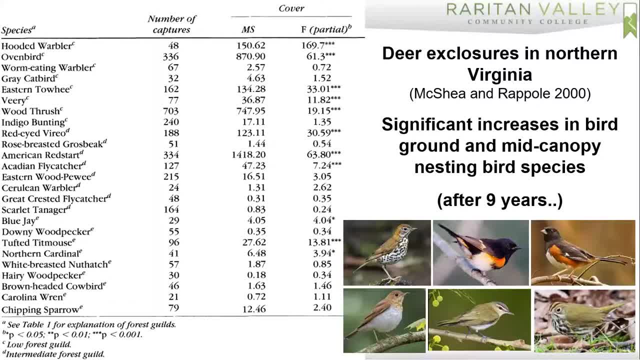 you start to see the bird populations bounce back as well, And so those cascade effects that we talked about earlier that are leading to declines in our animal populations and ultimately to the positive effects translated from just addressing this problem with deer And so just to turn it on its head. 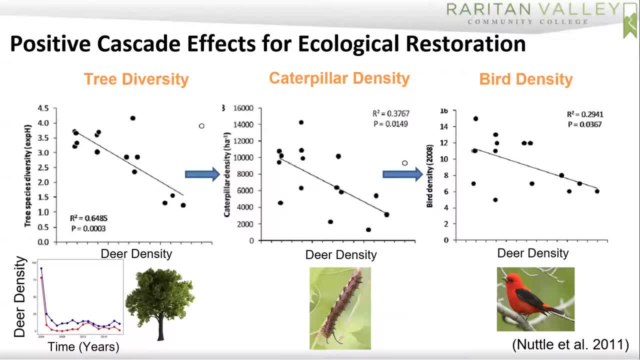 I tried doing a little animation here. Let's see if it works. So if we can correct the deer problem, referring back to these cascade effects, we can see tree diversity bounce back And with the return of tree diversity we can see, hopefully, improvements in caterpillar. 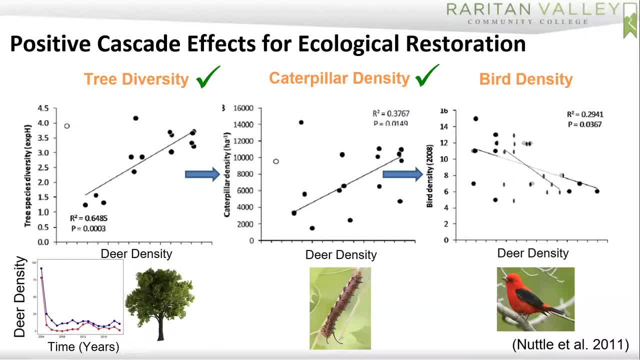 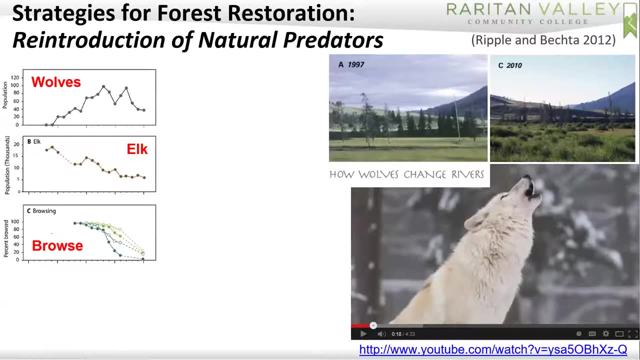 and other insects, fauna returning And with that in place we should get to see, as we just saw from the previous slide, benefits for bird populations And this kind of positive cascade effects for restoration were actually observed in Yellowstone National Forest after wolves were introduced in the 1990s. 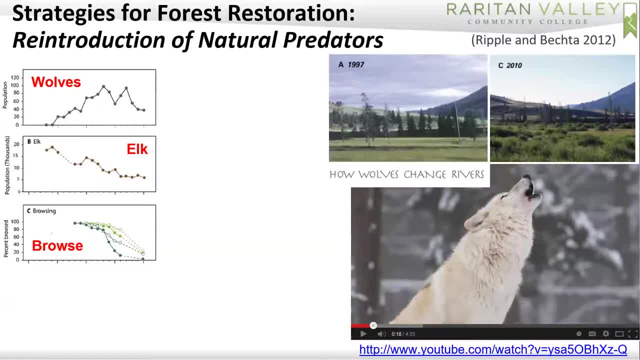 I should say they were reintroduced And you can see in the top left there. when wolves were brought back into Yellowstone, elk and other herbivore populations declined initially, with consequent decreases in browse impacts to vegetation, And because of that we saw the different tree species occurring in that area. 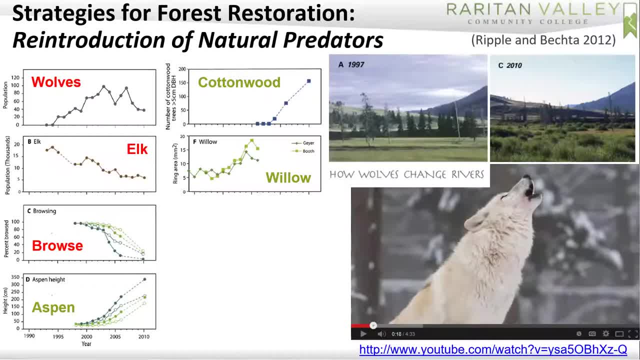 as well as shrubs and other as well as vegetation, recovering. in response to that decrease in browse effects of elk And because of the benefits of the increased vegetation, we saw wildlife populations increase. This is just data for bison and beaver. 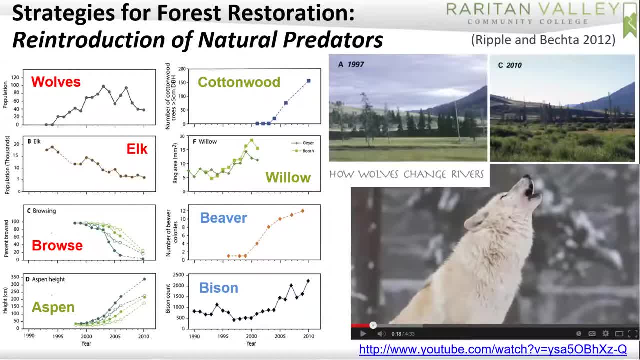 But if you read some of the other research by Ripple and Beshta, they've shown improvements to insects and birds and grizzly bears- all translating- as a result of this just initial reintroduction of wolves. that corrected the herbivore problem And so, while it's unfortunately very unlikely, 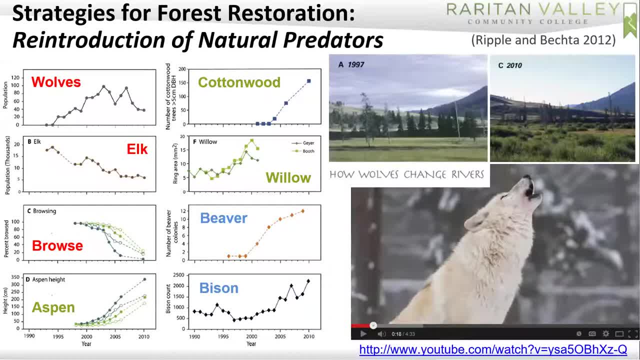 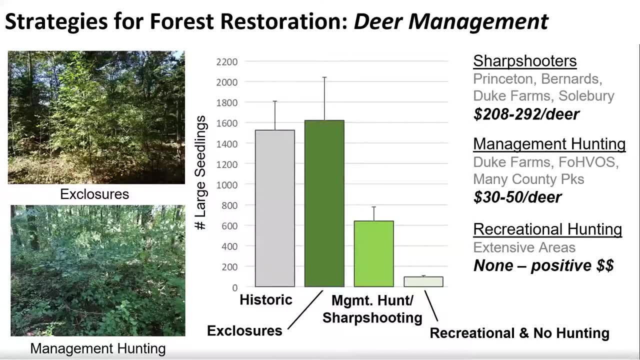 that reintroduction of natural predators is going to take place in the near future, at least intentionally. in New Jersey we do have similar techniques that we can use through predation to bring deer populations back under control through hunting or deer management- Unfortunately, recreational hunting alone. 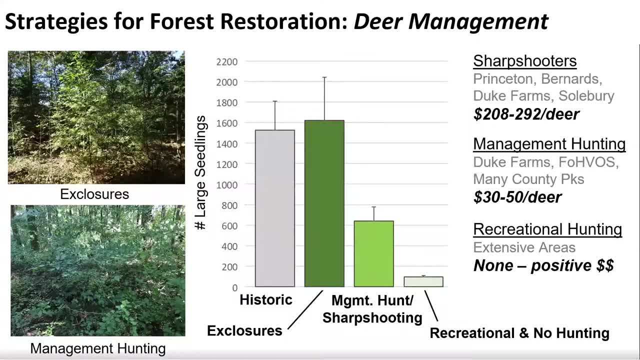 is not likely to be sufficient to correct these deer problems. This has gone on in New Jersey for decades And, while there's still many areas that need to be opened up to hunting to have some kind of impacts to deer populations, we're not seeing major, major, major, major, major major. 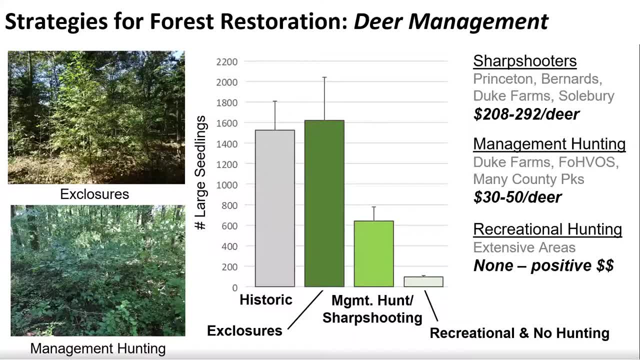 responses in forest understories, in places where recreational hunting is occurring. However, if you turn, put the proper kinds of incentives and policies in place for identifying what local deer populations are and figuring out how many deer you need to take out of the forest to get these kinds of recoveries to occur. 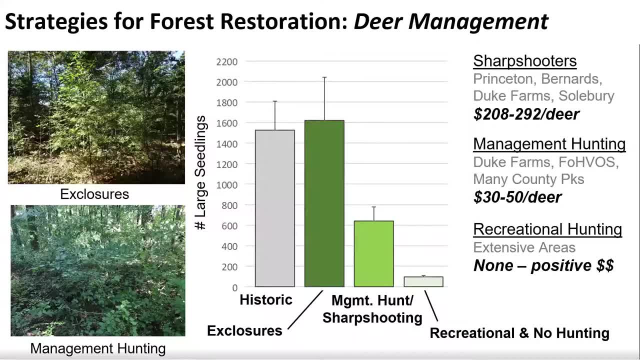 using harvest goals and quotas for hunters to try to achieve. this is referred to as management hunting. And in the places where that's occurring or sharpshooting is occurring, we do see meaningful benefits. We see benefits in forest understory vegetation. Sharpshooting is the fastest way to accomplish this. 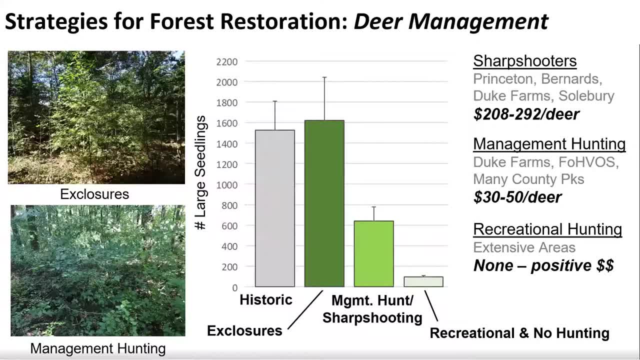 If you bring in professionals from the USDA or private sector outfits like White Buffalo out of Connecticut, this can be accomplished in a matter of a few evenings or weeks. The problem is, it's really expensive to do it that way. It can cost anywhere, typically from 200 to $300 per deer. 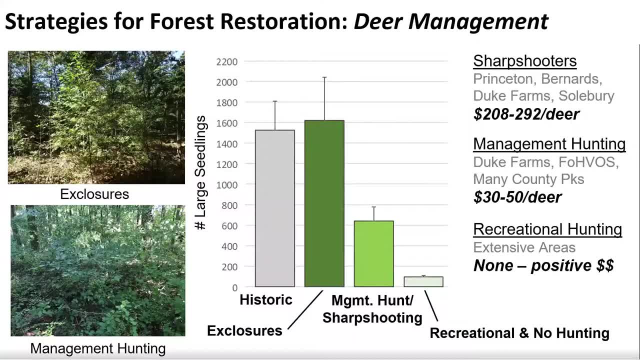 for these means to be used, but it is effective and you get results that will last you several years afterwards. Management hunting can be then used to keep the deer populations much lower once they've been reduced by culling, And that can also be joined with recreational hunting. 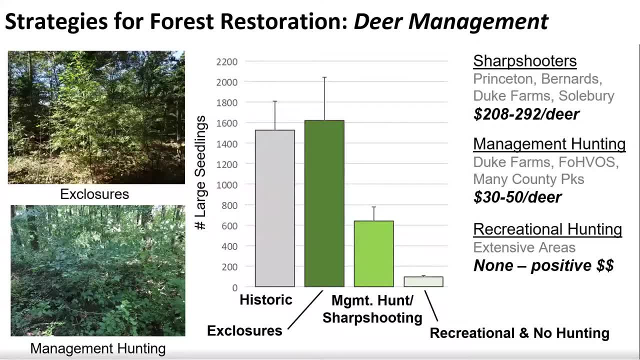 at the same time, which can provide some opportunities for people to get the benefits of hunting, but also have some management goals taking place to further suppress deer populations in those areas, And so you can see in the photo in the bottom left, this is an area that was management hunted. 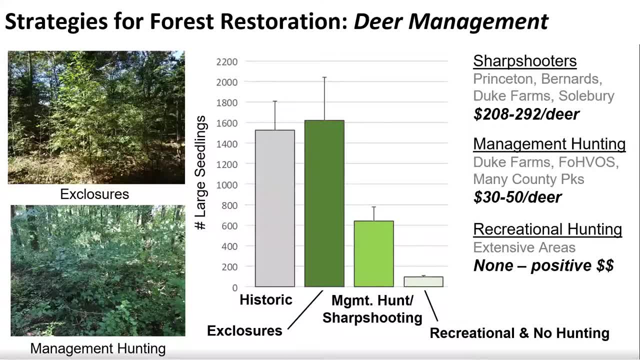 in Northern New Jersey And you do see signs of a healthy understory taking place there. Not quite as much as you'd get with an exclosure or as much as occurred historically, but still meaningful benefits. The problem is that this is again really expensive. 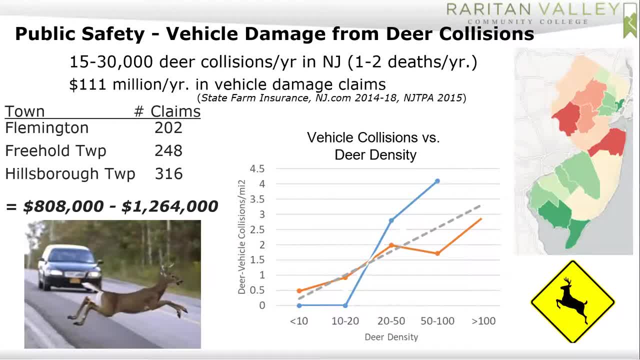 The idea of spending a couple hundred thousand dollars a year, or every few years, to hire sharpshooters to cull the deer herd is not something that a lot of townships would find possible or favorable. But if you turn that around and look at what we're actually paying, 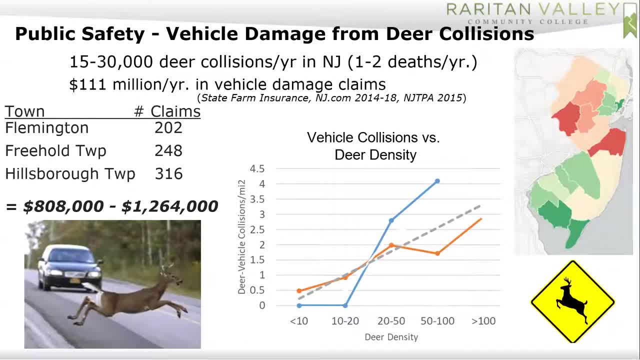 in terms of the costs to farmers and crop losses and to our landscaping and our vegetation impacts in our gardens, as well as to deer vehicle collisions, that factor alone would easily make the cost of sharpshooting worthwhile. This is data from State Farm Insurance. 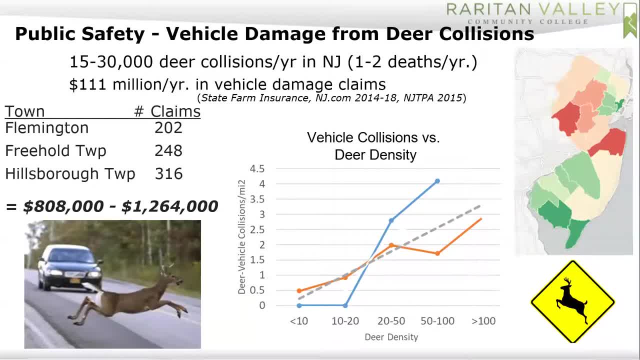 from the past couple of years You can see that some of our local townships have several hundred vehicle claims a year where people are reporting vehicle claims to the insurance company- damage from deer vehicle, deer collisions- And with State Farm estimating that each about $4,000,. 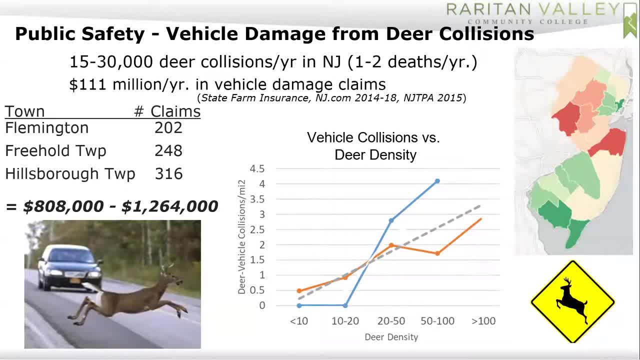 that's translating into $800,000 or more in vehicle impacts alone to repair the vehicles, not to mention the pain and suffering and hospitalizations and injuries and, unfortunately, deaths that are resulting from these collisions as well. And so if we, as communities, 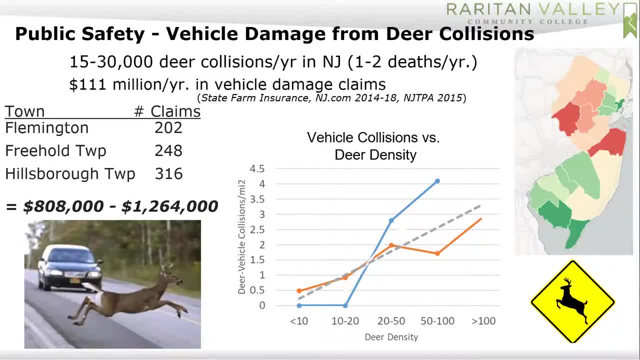 invested a hundred or $200,000 a year in culling the deer herd to bring it back down to levels that are manageable by recreational and management hunting, we would see tremendous cost savings in our community in declines in vehicle damages, because there's really clear relationships. 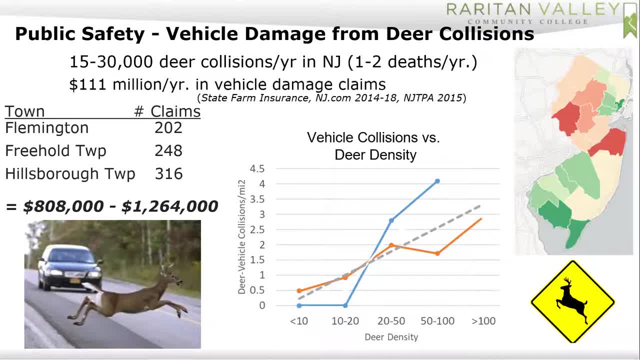 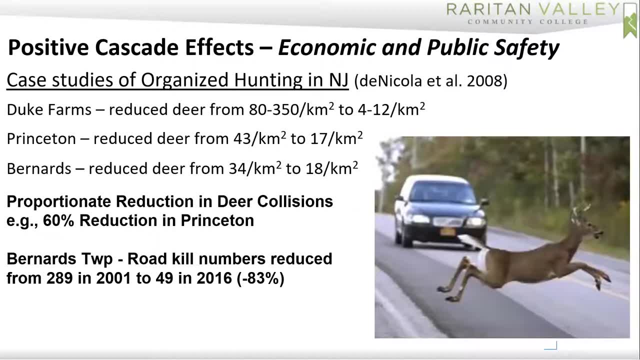 that we've seen from our research in local deer densities and the amount of collisions that take place in those places, And this is borne out by research as well. So some of the earliest communities that started sharpshooting in New Jersey, in Princeton for example- 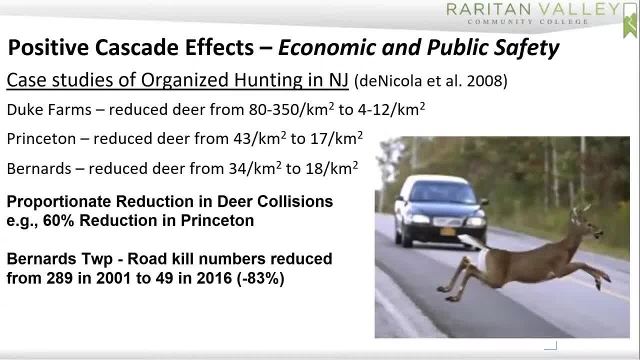 the very first year they engaged sharpshooters, they reduced their deer population by about 60%, and that same year they saw a 60% decline in deer vehicle collisions. And so what you get, essentially in the same way that we get positive cascade effects. 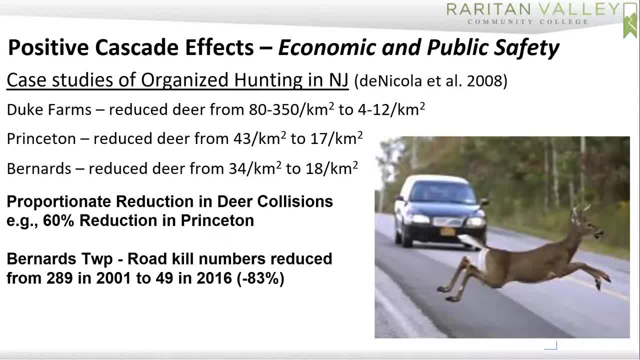 for ecological restoration, you get positive cascade effects for the social and economic effects that we're seeing resulting from deer populations as well, And so we could expect to see benefits for farmers, benefits economically and for public safety in terms of reductions in deer vehicle collisions. 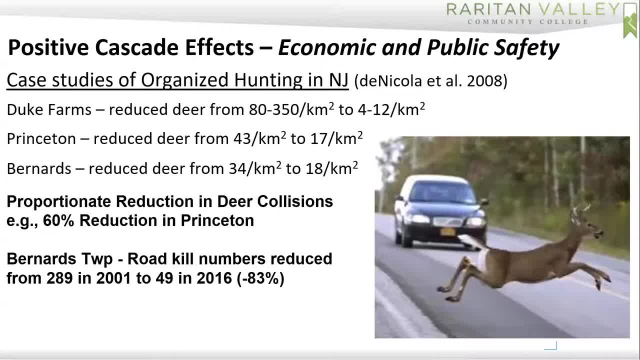 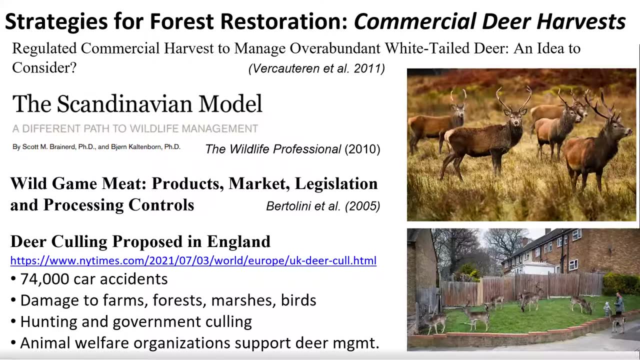 as well as public health in terms of Lyme disease and other infectious disease prevalence. that's related to tick populations as well, because deer are the main vectors of ticks throughout the landscape in this area. And, to make it even more affordable, we can also look to what other nations have done. 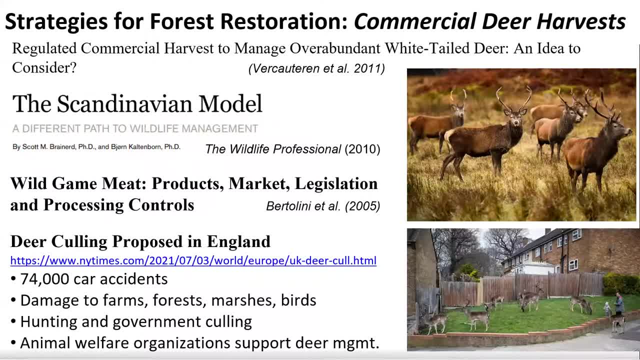 to tackle these same kinds of problems. As I mentioned, this Superabundance of large herbivores is happening throughout the Northern world, whether it's in England or continental Europe, Japan or elsewhere, And a lot of other nations have chosen. 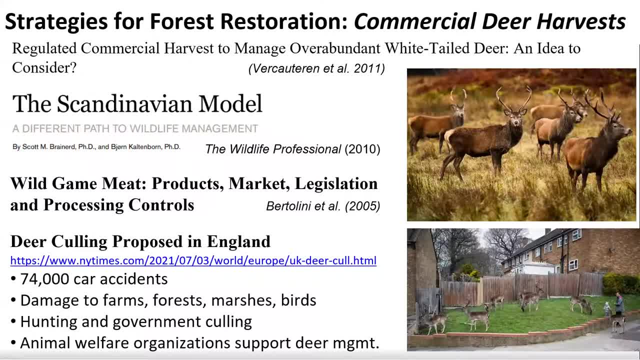 to return to commercial harvesting of deer, to allow deer meat to be sold in restaurants and, in some cases, in markets, to provide an economic incentive to reduce those populations. And so, whether you're looking to the Scandinavian countries, like Norway and Sweden, they've been doing this for years. 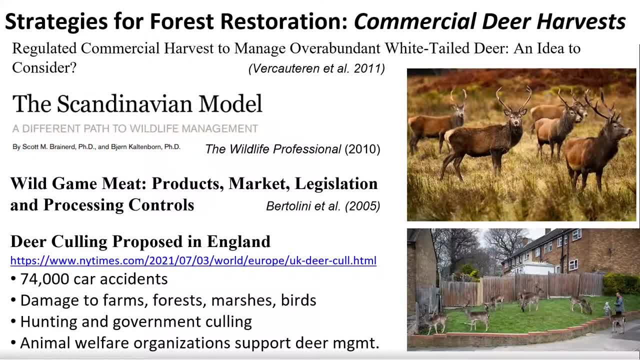 England's been doing it for years and pretty much every country in Europe, as well as Australia, Argentina for other games. they've been doing it for years, And so we can see that there's a lot of risk to the species as well. 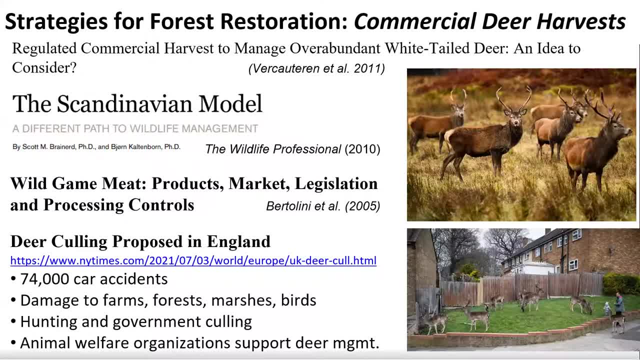 The risk for returning to commercial harvesting, of course, is that we theoretically could drive deer back down to extinction in the ways that we saw nearly a hundred years ago, But if you look to the places that have been doing this for decades, the encouraging thing is that many of them have found 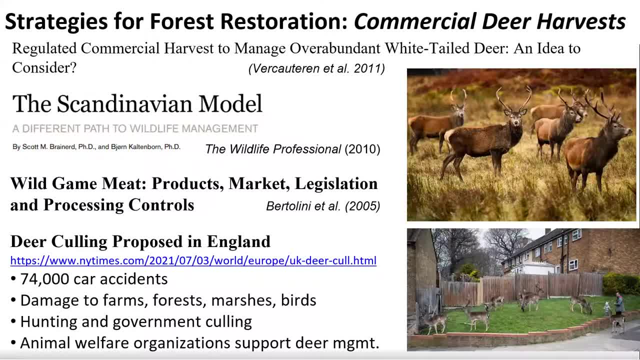 that not only are the strategies successful at managing deer populations, but there has actually been a reduction in the amounts of illegal harvesting. that's taken place, because it provides economic resources that make it easier for populations to be implemented, to manage the hunting, to make sure that it's being done at sustainable levels. 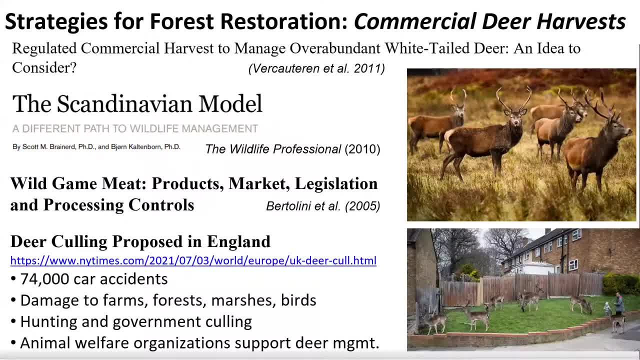 and enforce penalties against people that are hunting illegally, And so there's a lot of examples around the world I think we could turn to, and there are many groups in New Jersey that are starting to consider the possibility of trying to reinitiate commercial deer harvests. 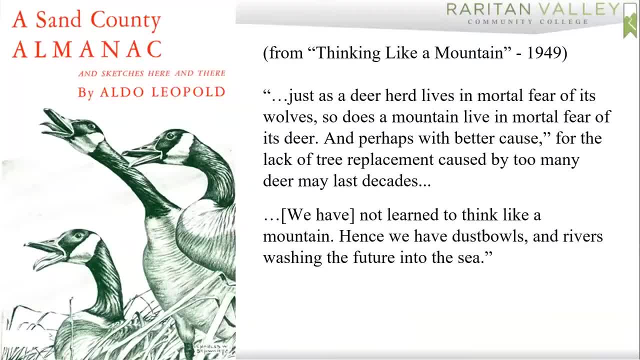 and other states are as well, And these concerns are not new. We're essentially dealing with the legacy effects of how deer were managed and wildlife in general were managed hundreds of years ago, when we had eradication programs to eliminate these predators from our landscape. 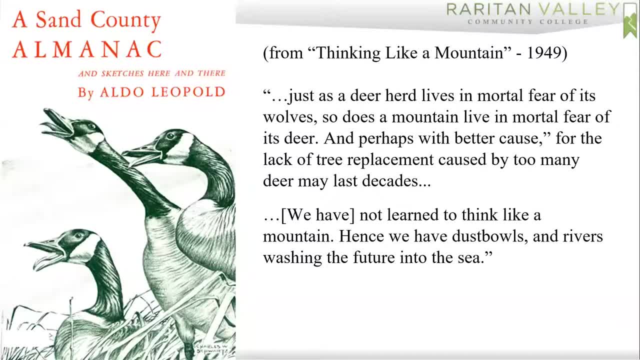 Aldo Leopold was the first to write a book on wildlife management. He had participated himself in these wolf eradication programs out West and realized the mistake that was being made, And you can read his accounts of that in his famous book, The Sand County Almanac. 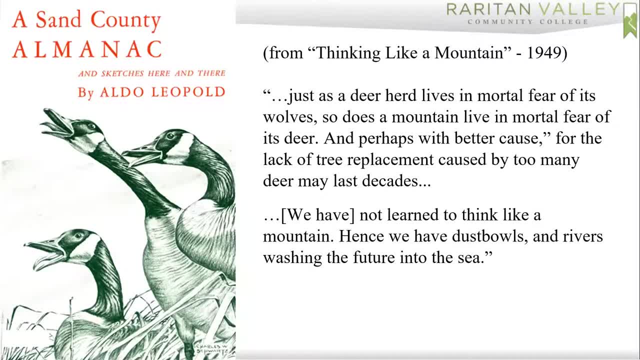 But he said: essentially we need to learn to think, like we have to think about how these things work, How these things are interrelated with each other. You might want to eradicate wolves and panthers to benefit your livestock, but then you're gonna have legacies of impacts. 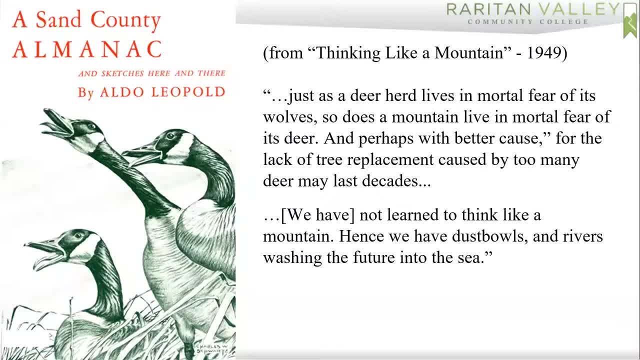 to forest regeneration, to erosion and losses of water quality and, ultimately, consequences that can extend generations into the future as a result. And so he said, we need to think like a mountain, And you can apply the same thing locally here as well. 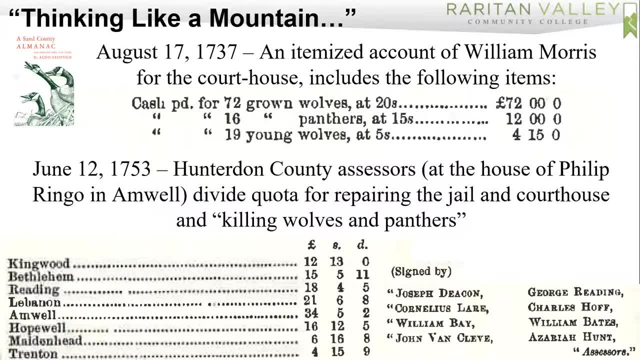 whether it's historically or today. So just this past week I stumbled over some historical accounts of these same wildlife eradication measures that were taking place in Hunterdon County, in our region, And you can see from the mid 1700s. 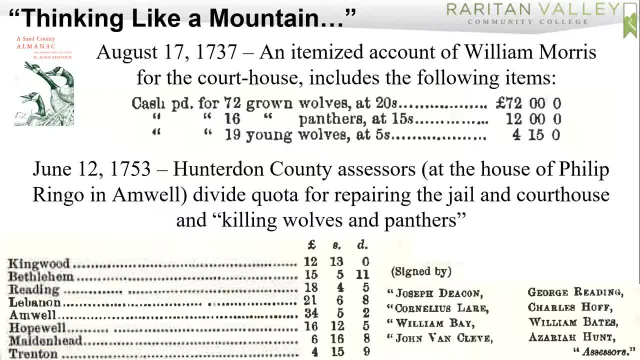 the bounties that were being put on place on wolves and panthers in our own area, with a single court settlement providing a hunter with rewards for bringing in almost 100 wolf and panther pelts, And all of the townships locally were engaged. 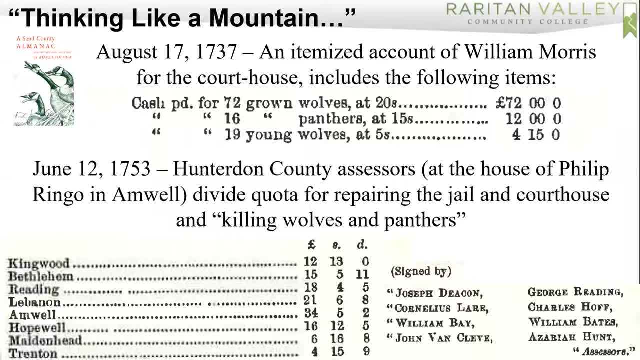 in those same kinds of activities, divvying up the amount of resources that it would take to eradicate wolves and panthers from our region, And we're still suffering the consequences of this today. So while they thought that they were doing, you know, 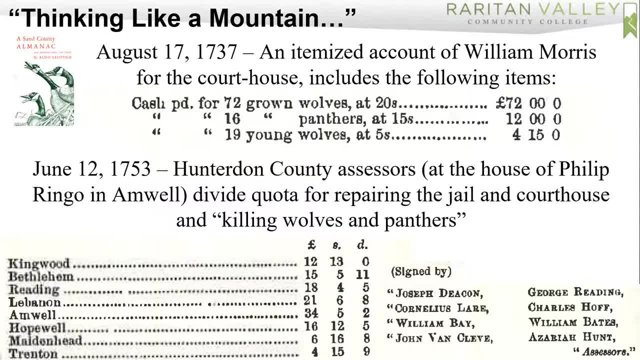 look good. during that time period, they weren't thinking like a mountain in this way that Leopold encourages us to do: to think outside of our single-minded efforts to eradicate predators for some sole benefit, because the predators have an important role to play. 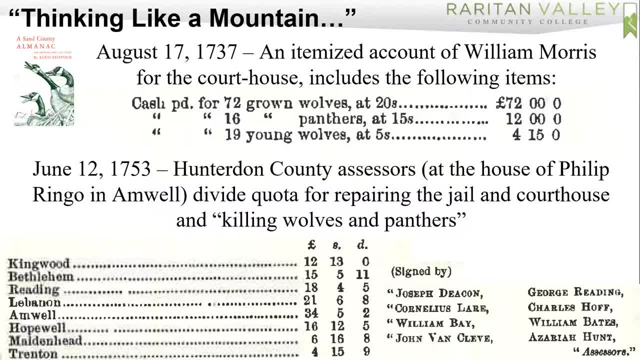 as deer do themselves, And it's up to us to think about this in this, from this perspective, to try to bring positive benefits back into the future, And that's very likely to occur if we begin to take this approach to ecosystem management in general. 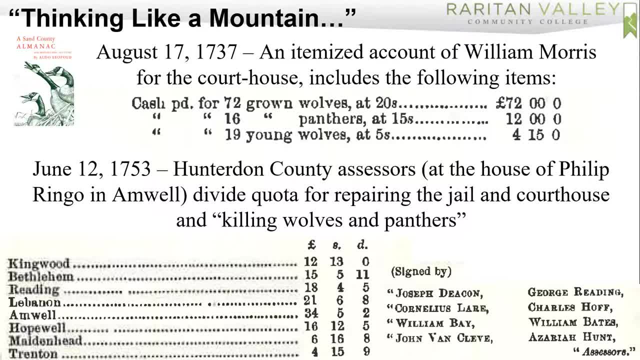 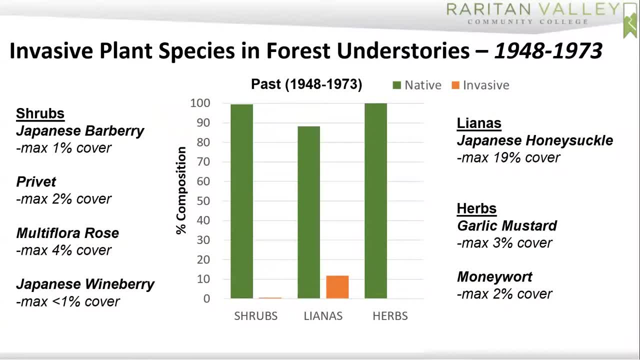 And we should be holding our public servants accountable for this, but ourselves as well, because we're all part of this story and have a role to play. So that's the issues with deer in a nutshell, And I'll go through a little more quickly. 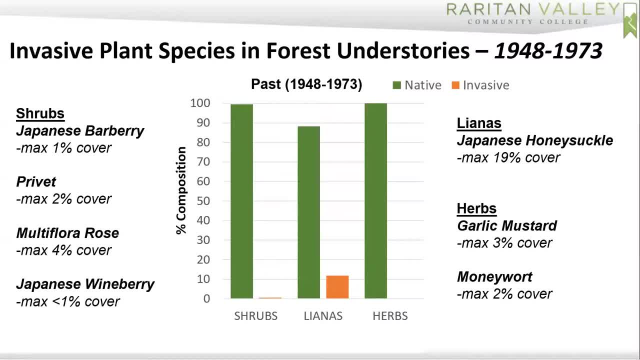 with the problems of invasive plant species. It's an equally complicated story and requires different strategies in some cases to address. If you look back to the historic data set that I was talking to you about earlier, you can see in the mid 20th century. 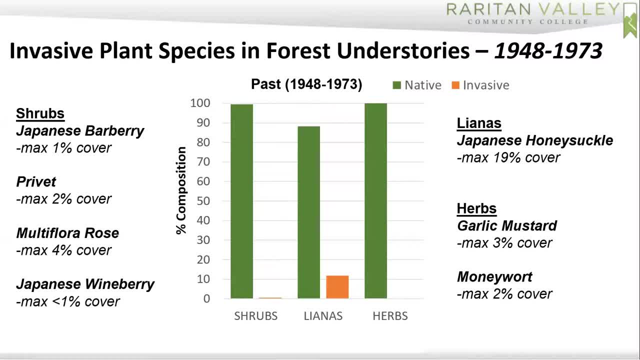 there were invasive plant species present in our forest, but they were not frequent at all. Most of these plants that are now widespread and overrunning our forests and our farm fields only occurred at about less than 5% cover in any of these forest studies that were conducted. 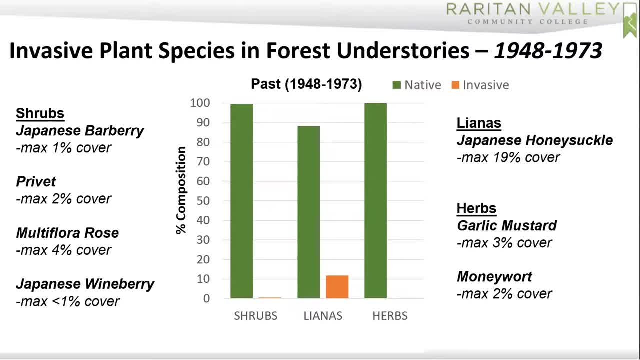 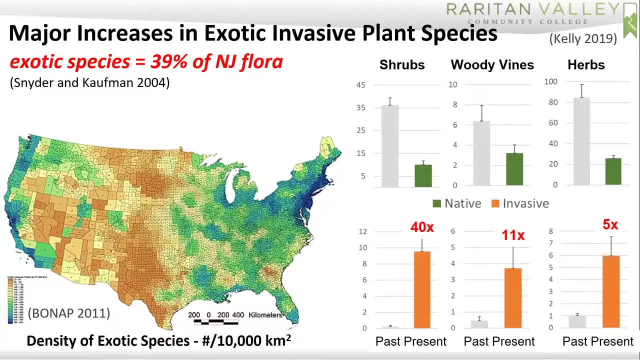 Only Japanese honeysuckle was prevalent, with two forests having about 20% cover. Most of the understory was comprised of native species, as you can see in the green bars there, But of course the invasive plant species have risen dramatically during the same time period. 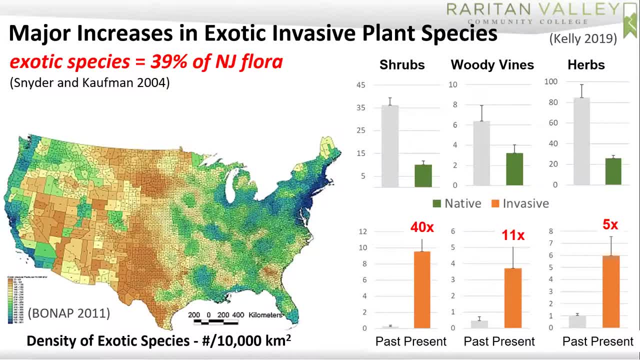 that deer populations have increased. So while we saw declines in our native understories, invasive plant species stepped in to fill that void, because these are unpalatable to deer And in our region in the Northeast corridor from Boston down to DC, we have some of the highest concentrations. 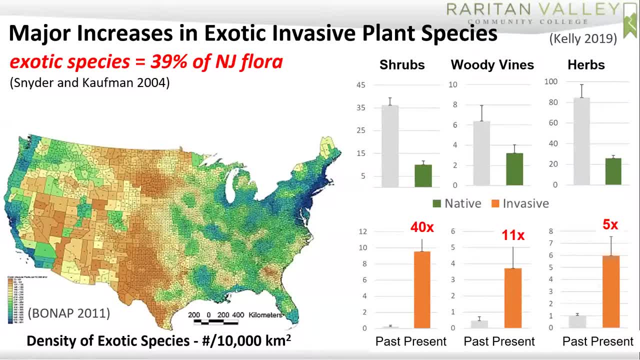 of invasive woody species of anywhere in the continent. The only places that are comparable in the country are the San Francisco Bay area, And you can see just how in the dark blue areas there on the map how much more elevated these levels are in our area. 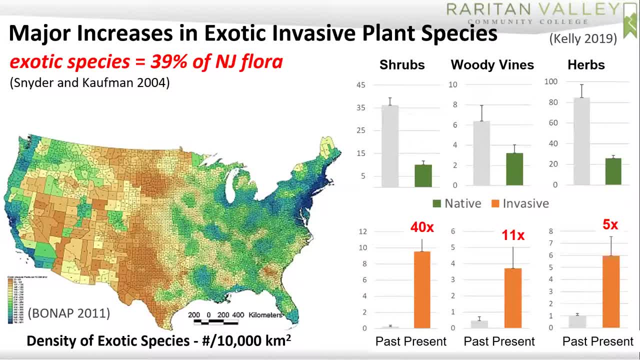 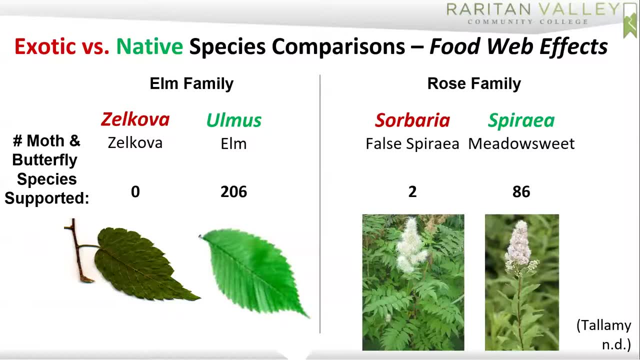 Today in New Jersey we have about 4,000 species. In New Jersey, non-indigenous species represent about 40% of all the plant species that occur in the wild in our state And that number is increasing. And while the impacts are many, they have the same kinds. 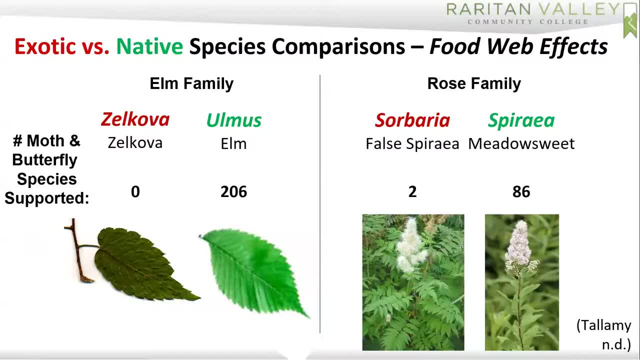 of food web effects that we saw taking place with deer. Dr Tallamy, who, we're lucky to hear from this morning, has done some of the most important research in this regard. Some of the early data he published showed comparisons of these introduced species and some of their native relatives. 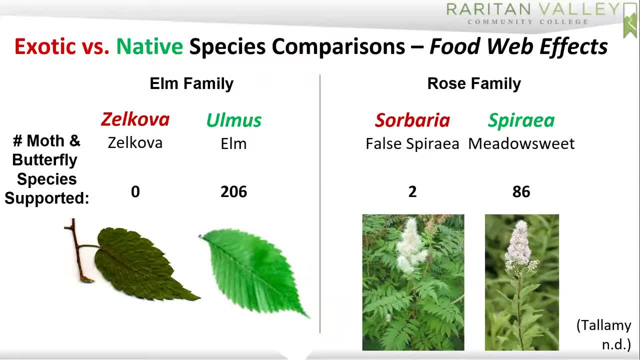 And so I just took some excerpts from his research that had been published on his website, And you can see that in the elm family, within the tree group, our native elms are supporting hundreds of different moth and butterfly caterpillars And the close relative that's been introduced. 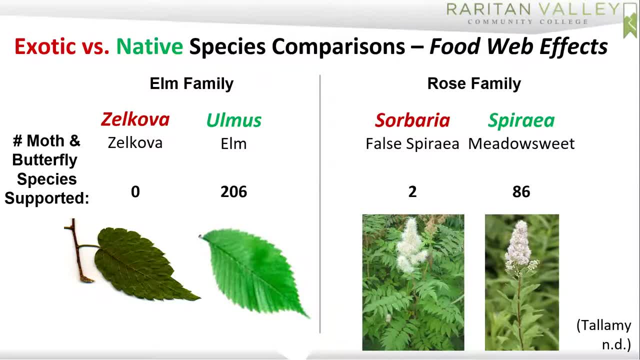 from the old world. the Zelkova doesn't support a single one, according to his research, And so, while they're very similar species that can occupy similar niches, they don't have the same kind of benefits for our native invertebrate. 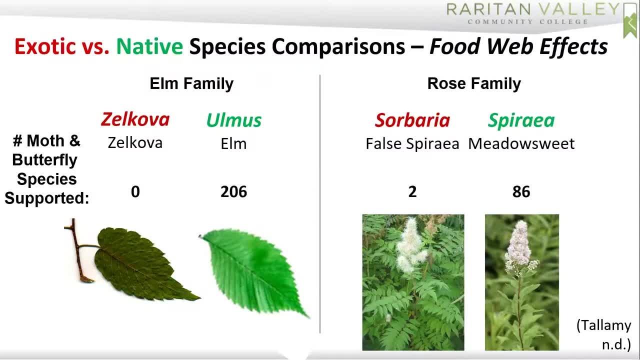 fauna In the shrub layer. just two examples from the rose family you can see our native spirea supports dozens of different moth and caterpillar, sorry moth and butterfly caterpillars, The close relative, the false spirea from Asia. 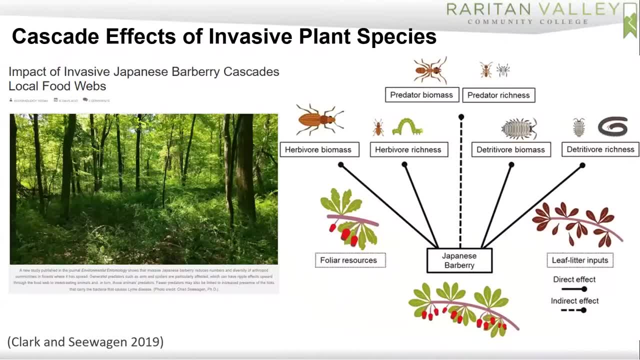 has been found to support only two, And this translates again throughout the food web, with some research from New England showing that forests that are infested with Japanese barberry have found major declines in other kinds of herbivores as well. It's not just the insect herbivores that decline. 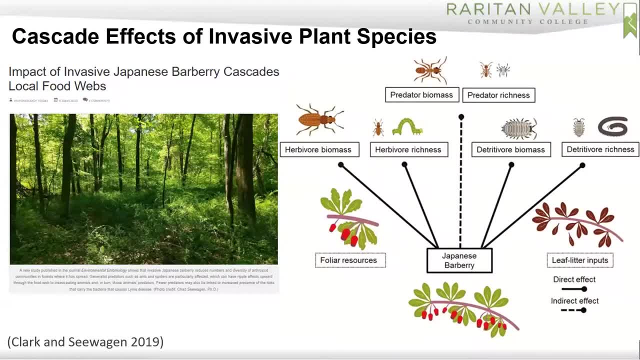 but the predators that decline in response to their populations decreasing, And even the detritivores decrease as well, because all these invertebrates are operating primarily on chemical cues that tell them what's food and what isn't. And these invasive plant species? 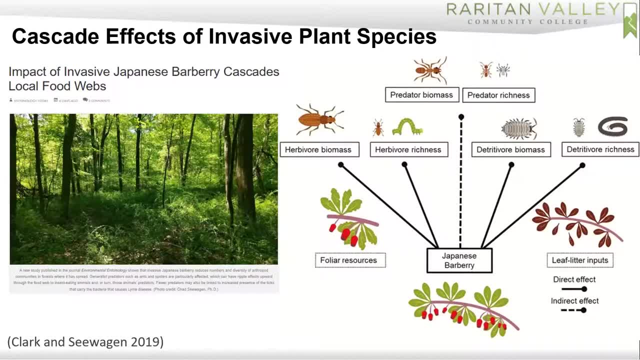 while they do provide some benefits to our forests, they're still sequestering carbon to some degree. They're still providing some nesting habitat, for example. They don't provide anything like the same sorts of quality resources for food, in particular for invertebrates. 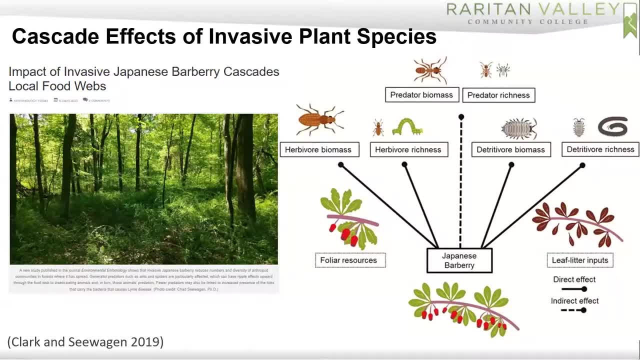 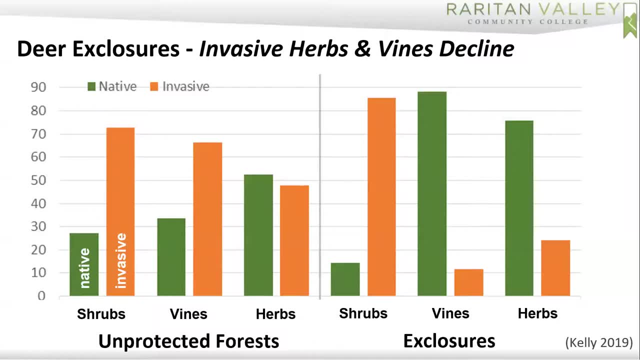 as our native species do, And so the same cascade effects are resulting from invasive species. Deer are part of this equation as well. As we mentioned, the invasive species are the least palatable to deer, So they will eat invasive species, but they choose to eat them last. 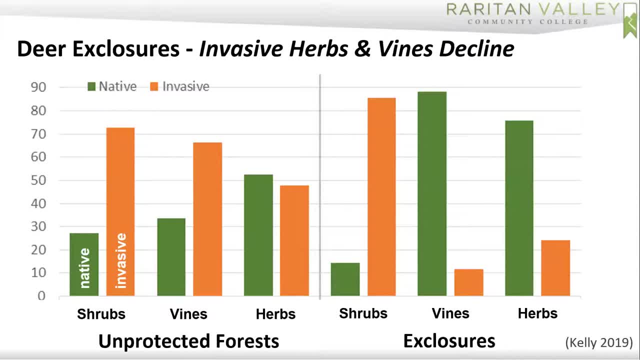 And so if you look to the deer exclosures that we've studied, in those places where deer have been removed from the equation, you can see native vegetation bouncing back and out-competing invasive species in many places, The vines and herbaceous layers in particular. 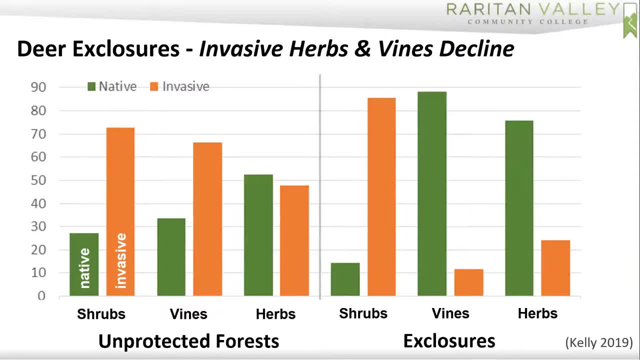 have been really successful in out-competing the invasives once you take deer out of the equation, And so what's happening essentially is the deer are suppressing our native species, And that's what's allowing the invasive species to rise up to the levels that are occurring. 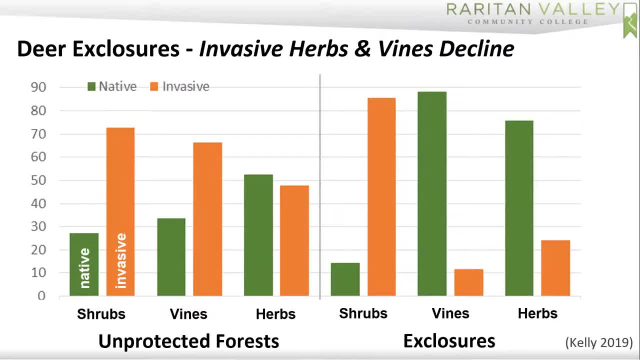 The shrubs haven't bounced back to the same degree, Primarily because of seed source factors. There are so many invasive shrubs in the landscape at this point that when you remove deer from the equation, there's still an abundant seed source available that brings them right back into those places. 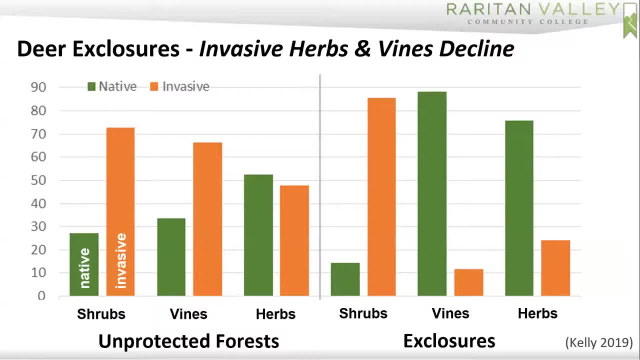 and they still out-compete our native shrubs, Because there are so few native shrubs around in many of our forests, especially in the fragmented forests in central New Jersey, that they just can't bounce back on their own, And so additional efforts might need to take place. 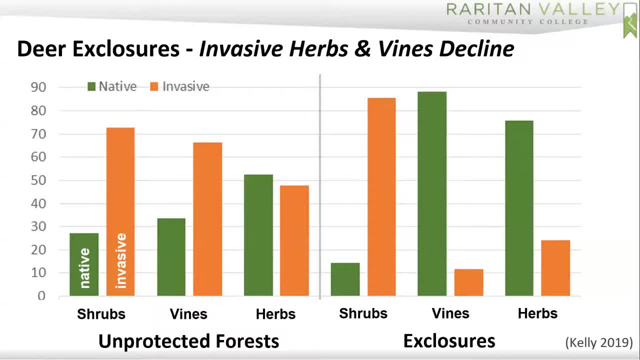 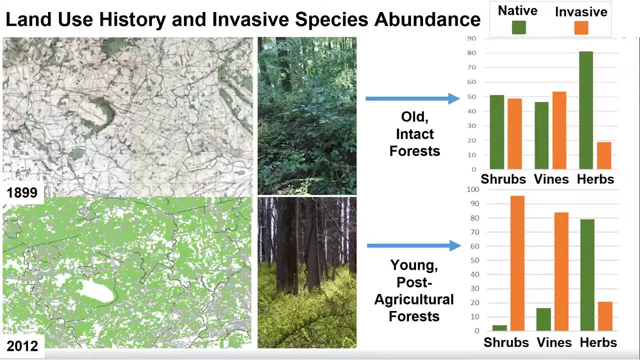 in suppressing invasive shrub species or supplementing the native shrubs by planting them into the forests directly. The other factor that's really important to consider, that's favoring the prevalence of invasive species in many areas, is forest history and land use. Much of our forests today are fairly young forests. 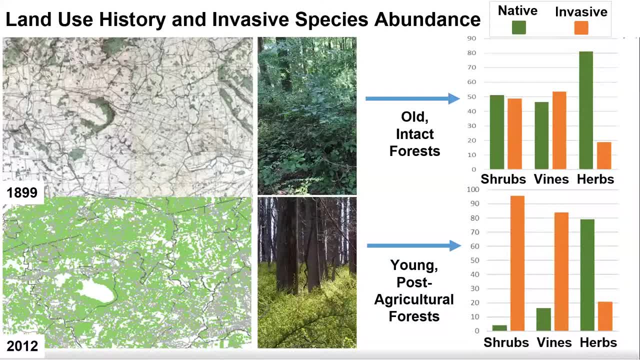 that are growing up on abandoned farm fields. As economic conditions changed in the early 20th century, many farms in our region were abandoned and farms reverted back into forest environments, And so we've benefited from dramatic forest recovery as a result. The problem is that these forests that are growing up 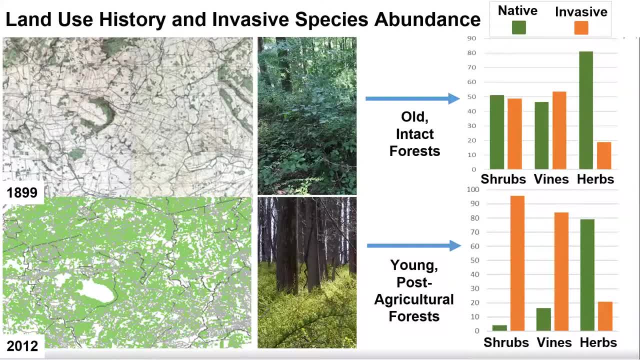 on soils with a history of disturbance and, in some cases, degradation from agricultural activities, look very different than the old, intact forests that have been around since the pre-colonial era. And if you look to those forests that are old and intact in the landscape, 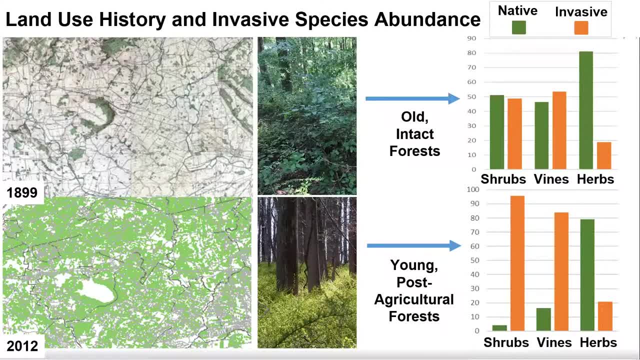 if you can compare them- native and invasive composition- they're about equal parts native and invasive. in terms of the woody species present, The herbs are still holding out a little bit better, But if you look to these post-agricultural forests that are growing up on abandoned farm fields, 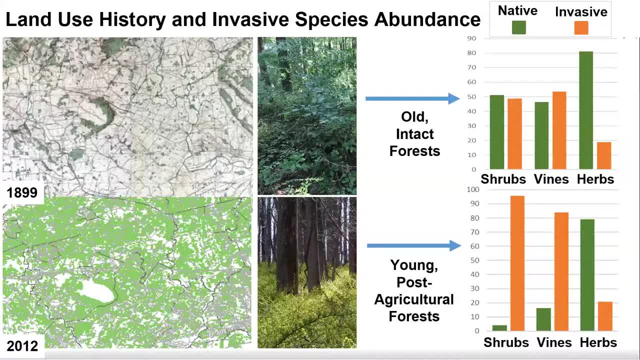 they are far more comprised of invasive species in the understory than native species, And so these forests look radically different than any kind of forest that have ever existed in these sorts of areas, And so, in addition to deer, we have to think about land use history. 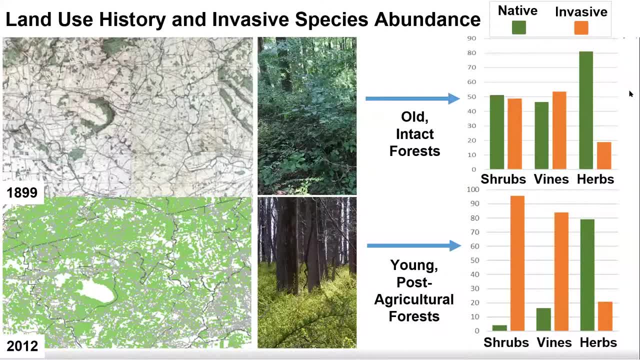 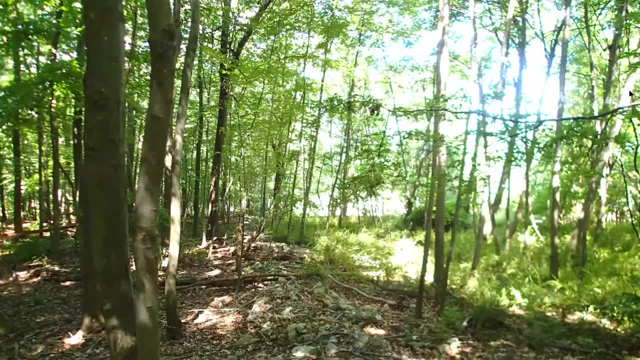 and those sorts of contexts that might favor invasive species growth over others. And you can see this really readily as you walk through any of our local forests. You'll cross an old stone wall on a trail and that indicates that on one side of that wall 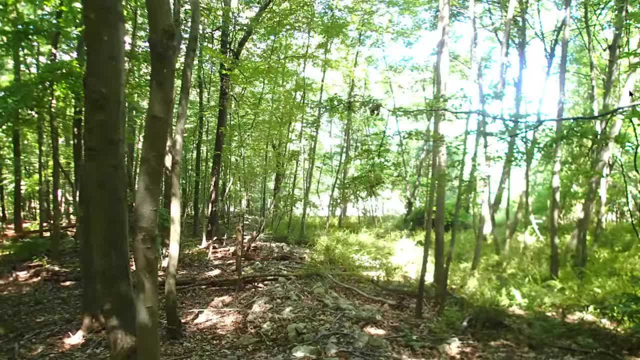 there was a farm field at some point historically. even if there's a forest there today- And if you look at this image, you can see on the left side- there's next to nothing in the understory of the forest. That's an old, intact forest. 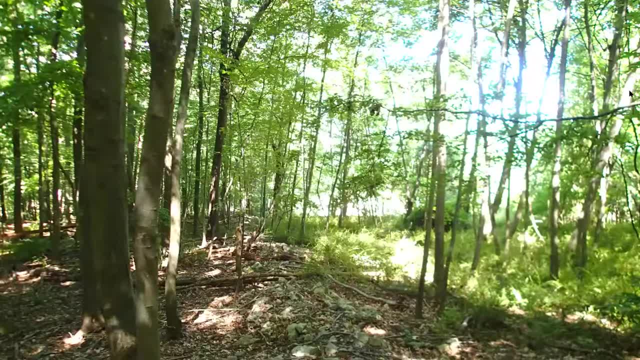 And on the right side, the forest is lush with green vegetation, where that's all invasive species- Japanese barberry and wineberry, and multiflora rose in this case- And so it's like night and day, and you can still see these legacy effects. 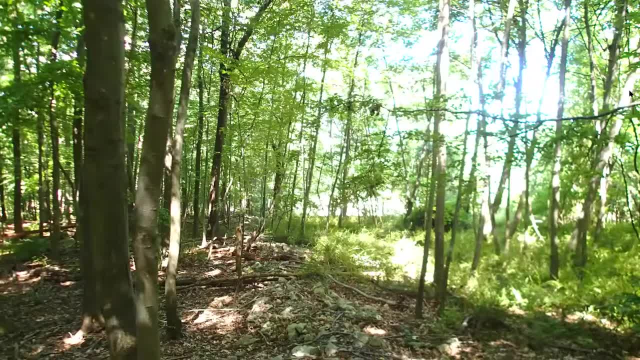 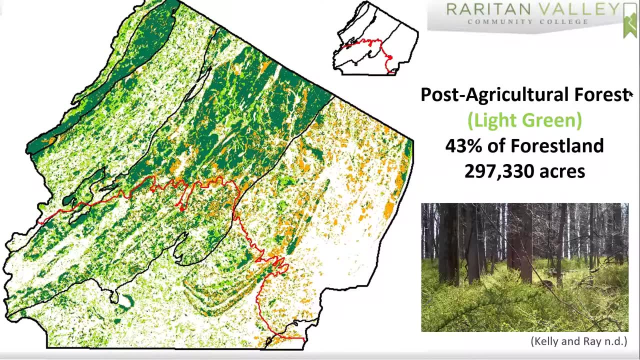 from agriculture nearly a century later, taking place in our forests, And this is important because the scale of these forests in New Jersey is enormous. Almost 50% of the forests that occur in Northern New Jersey are comprised of these post agricultural forests, And so, if they're this infested with invasive plant species. 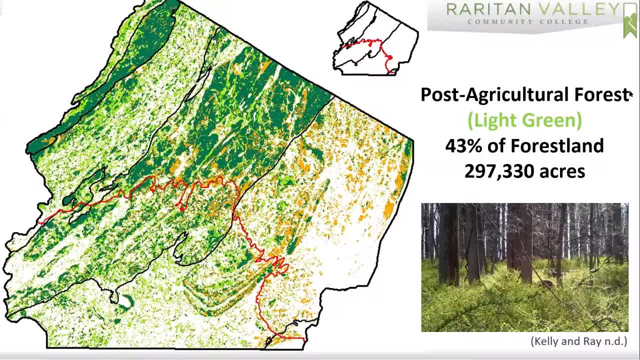 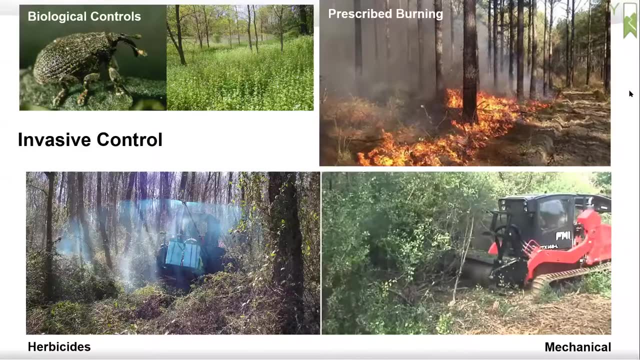 this clearly has to be a priority for forest restoration in the future, And targeting these forests in particular for suppressing invasive species and trying to recolonize them with our native species that are so lacking and so needed to support wildlife in these places. In doing so, and trying to knock back 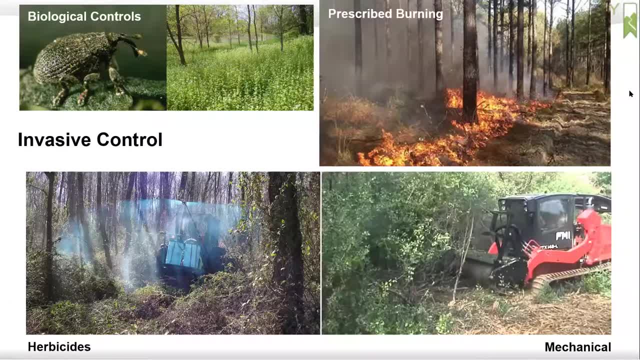 this incredible wave of invasive species. there's a couple of different tools available that are useful to consider at this scale. Herbicides and mechanical treatments are possible, but they can lead to collateral damage, impacts to native species or fauna, or water quality, or soils for that matter. 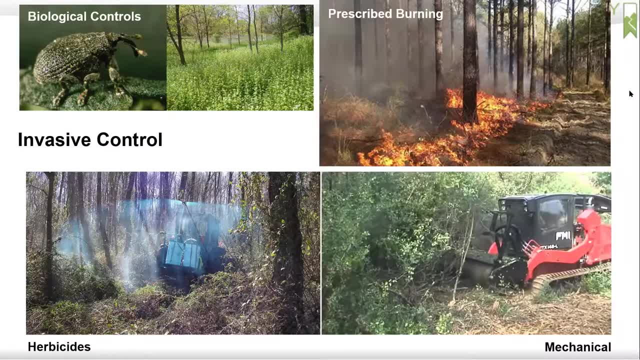 And they also tend to be much more expensive. The more affordable and more endemic sorts of approaches involve either using biological control, biological controls or prescribed burning. Unfortunately, with biological controls there are, it can be a really useful strategy for tackling invasive species in general. 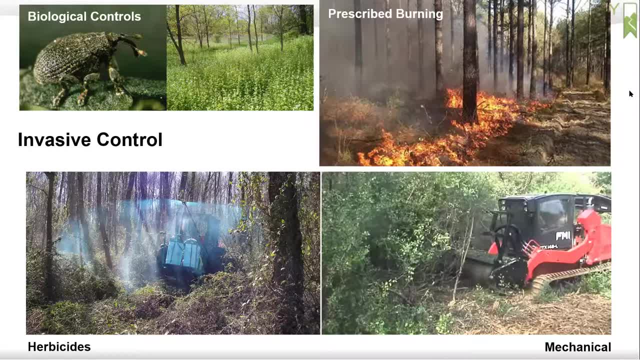 but there just isn't enough research to provide solutions in this regard for the hundreds of invasive species that are already occupying our landscapes, And so, while that's a really potentially fruitful avenue to pursue in the future, right now it doesn't really offer a meaningful solution. 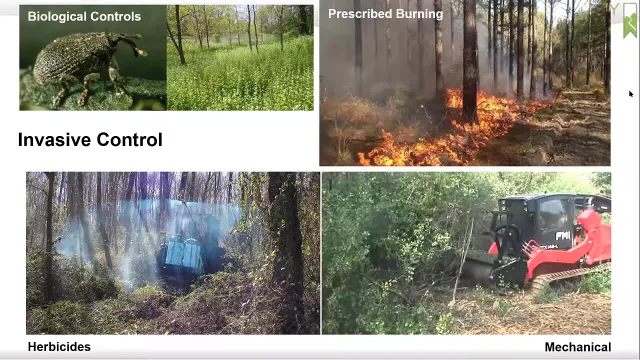 for tackling most species that we're trying to deal with. Fire, on the other hand, is an endemic part of our landscape. Many of our species are adapted to fire And we know that for thousands of years, native Americans were burning our forests regularly. 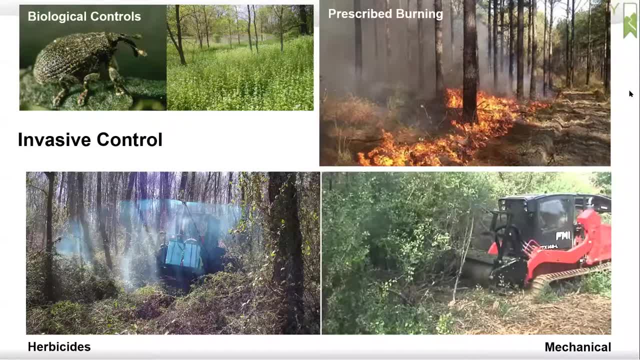 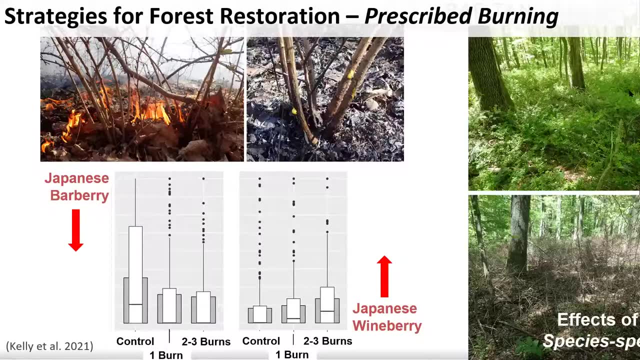 for hunting and for agriculture and other uses, And so we've been doing research for the past three years to try to determine whether fire might be useful as a tool for suppressing invasives as well, And we've found some pretty hopeful signs. Some species like Japanese barberry, Japanese wineberry, 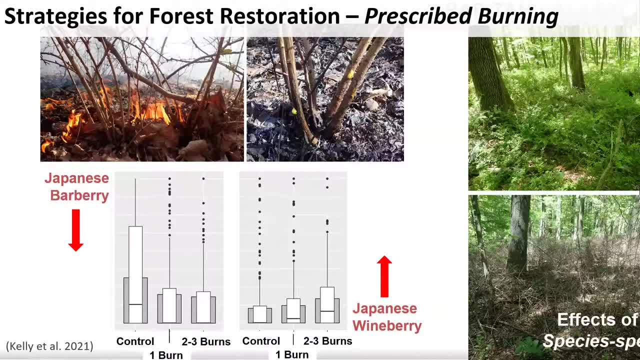 I'm sorry, not. wineberry, multiflora, rose and Japanese honeysuckle are hit pretty hard by fire. Even a single fire will reduce Japanese barberry by about 50% And subsequent fires can reduce it even further. And when you see a fire moving through, 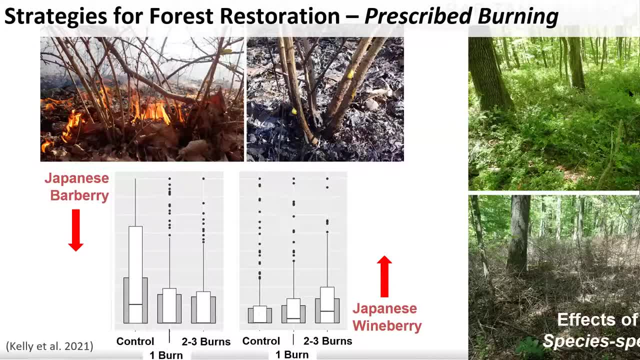 a Japanese barberry stand. it's really clear how that takes place. The fire it's got very thin bark And after the fire passes through you can watch that bright yellow sap just boiling out of the cambium of the barberry. 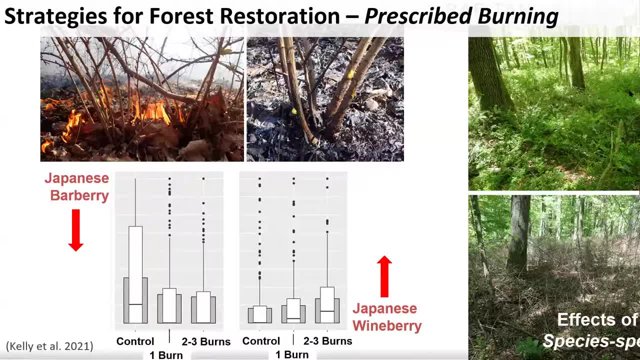 And it really knocks it back substantially. Other species, however, are just as adapted to fire, as many of our native species, Like Japanese wineberry, for example, actually increases in response to fire. So if you're gonna be using fire as a tool for invasive species suppression, 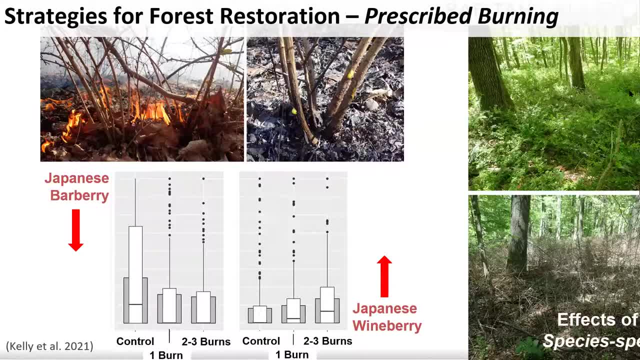 it really is important to do a survey first to figure out what species are invading your forests, before you think this is gonna solve anything, Because if you have wineberry or some of the other species that respond positively to fire, you're actually potentially gonna make the problem worse. 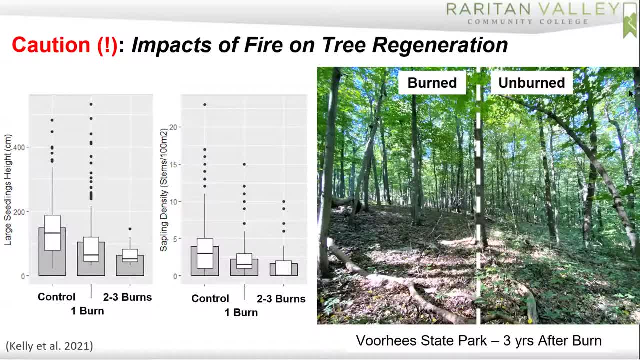 The other factor to consider is that, in this world of increased deer populations, if you burn a forest understory where there's healthy regeneration taking place and there's either a healthy shrub layer or young trees growing up, it'll knock those species back as well. 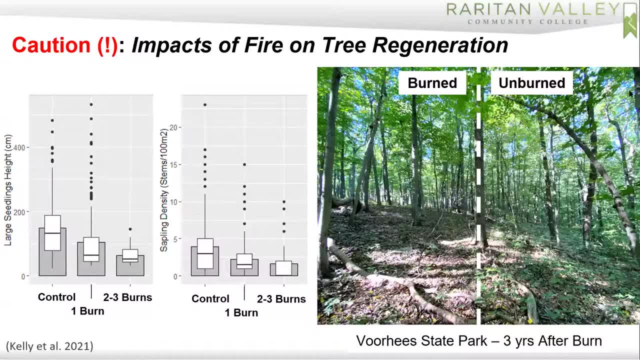 And the deer will keep them knocked back, And so this is just an example from Voorhees State Park. It was burned once, three years ago, And you can see the area on the left had been burned Even three years later. there still isn't very much regrowth of young trees. 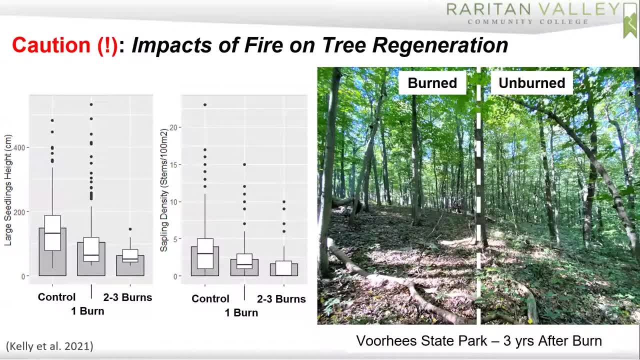 compared to the adjacent area in the forest on the right which was not burned, And you can see the lush growth of spicebush and maple leaf viburnum and young trees growing up in that area. So if you've got a high quality forest, 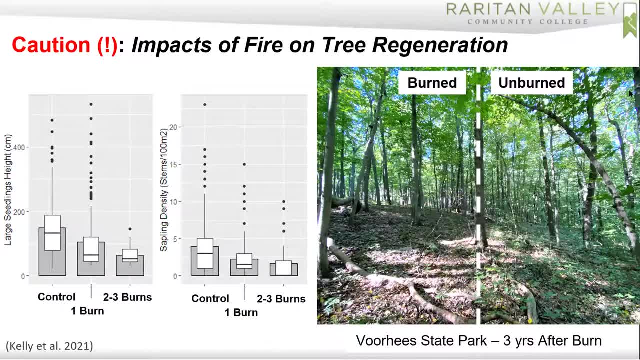 where there's a healthy understory already in place, it can actually be really detrimental to knocking back that advanced regeneration and understory quality because the deer again are waiting there to potentially browse it back down to the ground once it's put into reach. 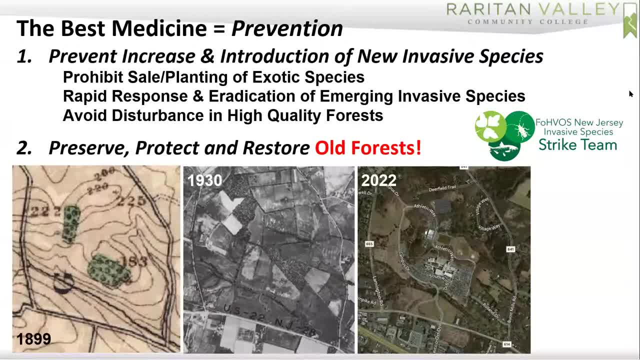 So, in terms of tackling this strategy of, or this problem of, invasive plant species in the landscape, the best strategy is prevention. We're continually introducing new species into the landscape. It's almost entirely uncontrolled at this point at the state and the national level. 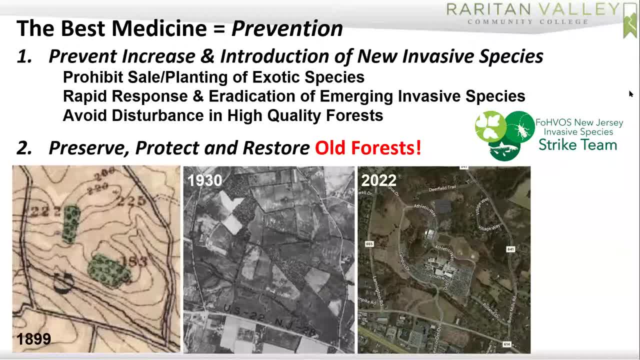 We have new species being imported to North America every year- or exported from it, for that matter, into other parts of the world, And we really need to start thinking about enacting some legislative controls against this in the future to have any chance at restoring our forest in the long run. 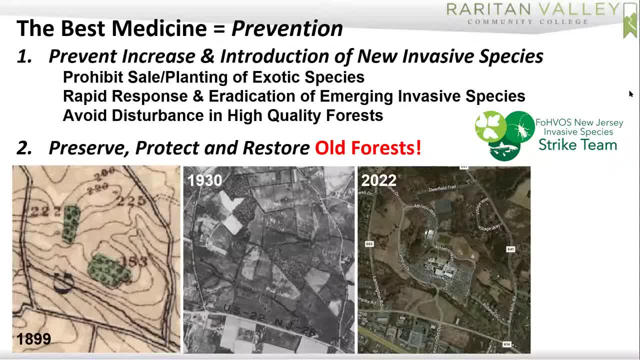 Because even if we knock back the species that are infesting our forest today, we'll just be dealing with another one tomorrow or 10 years from now if we don't address this from the standpoint of prevention. And again, we're all part of this story as well. 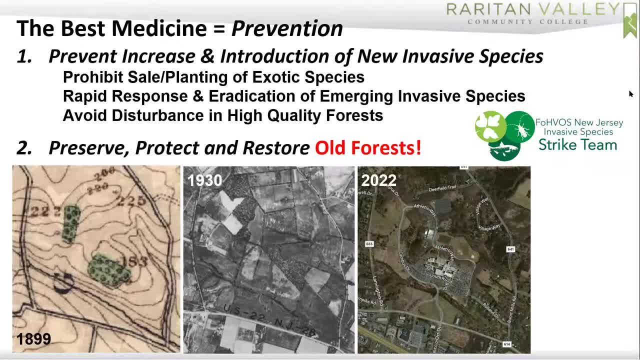 So we can get involved either in choosing what we plant in our landscapes wisely, making sure that we plant native species, which I don't have to tell anybody in this group about, I'm sure, engaging with groups like the New Jersey Invasive Species. 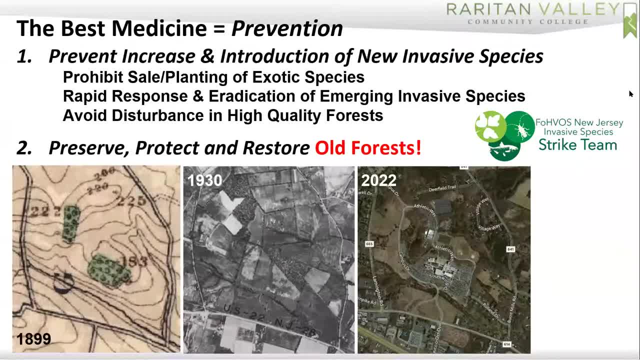 Strike Team that are trying to identify emerging invasive plant species and tackling them before they get to these problematic levels, and doing our part to try to reduce disturbance to the high quality forest that still remain in much of the state. making sure that the wrong kinds of forest policies. 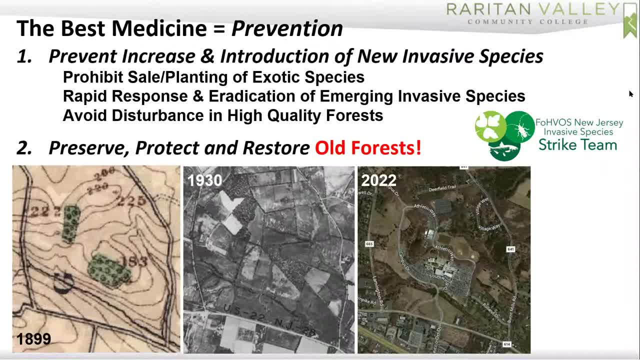 aren't implemented in those places. that could be really counterproductive and need some worsening quality in those forests over time. One of the best things that we can do locally is to try to identify and preserve our old forests. We're really fortunate in New Jersey. 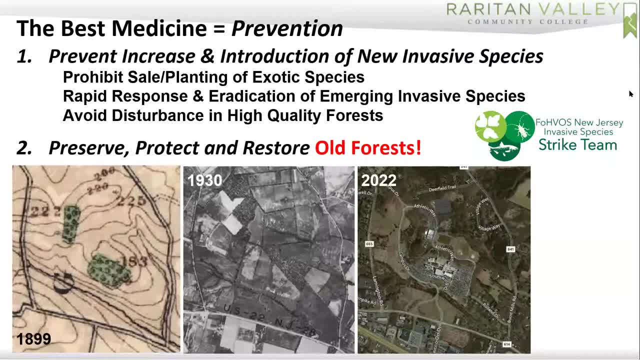 to have maps of old forests going back to 1899. And with the aerial imagery that's available today on websites like the Conservation Blueprint or the GeoWeb or other online tools, you can see where these old forests were in 1899 and follow them all the way to the present. 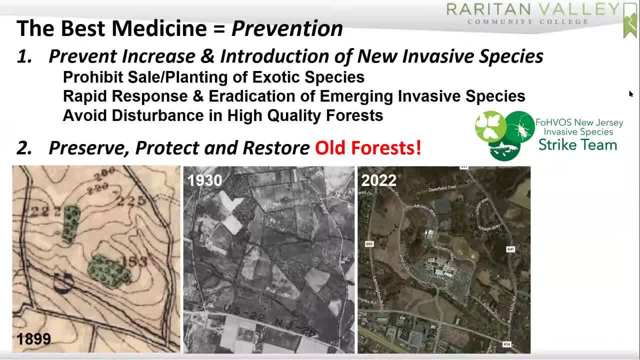 in the succession of aerial photographs that are available, identify them in the landscape and try to target them both for preservation and restoration, because they tend to be the highest quality forests, as it is, with the most intact seed banks and soil, And it's gonna be the easiest to revive them. 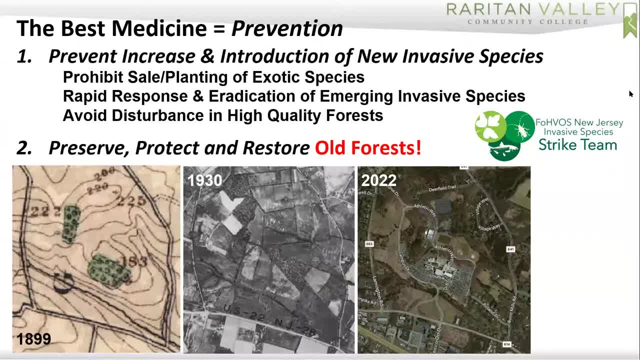 into the kinds of conditions that we need to support wildlife, And right now, they have no status for conservation or protection other than what people voluntarily give them, And so those of you that are on open space advisory boards or environmental commissions in your communities, these are really important resources to target. 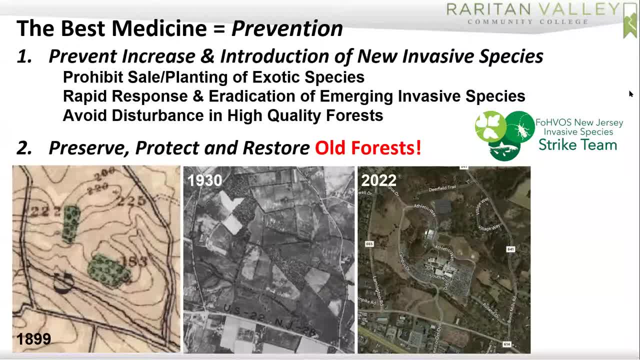 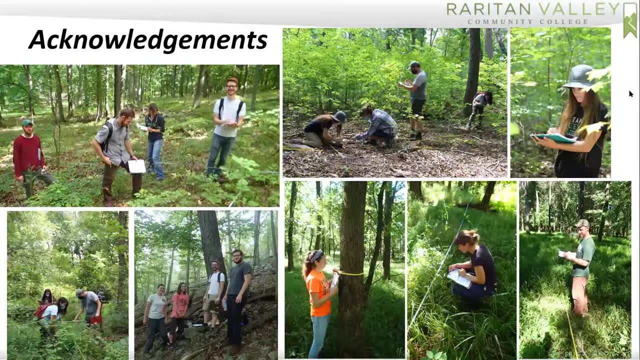 for conservation and restoration purposes that require us all locally to get involved until some sort of protective status is implemented for these old forests in the state. I have an enormous number of people to thank for putting all this together. We've had really great fortune in having cohorts of students. 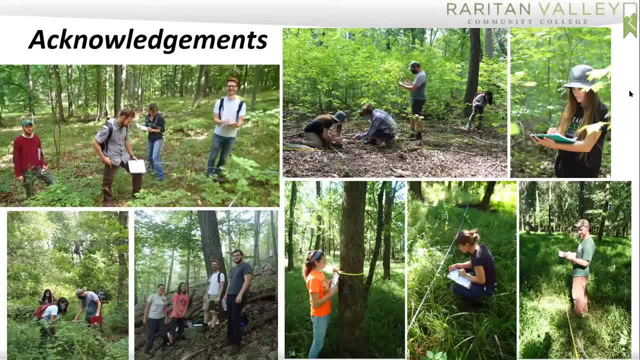 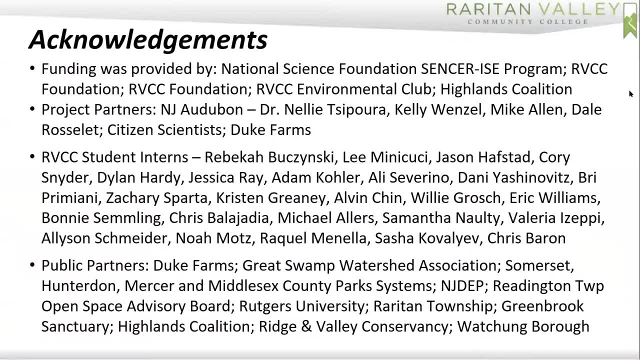 move through and contribute to our research program. that have just been phenomenal, And this is some of the smiling faces that collected all the data for us. here at Raritan Valley, We also have community partners that have supported our work, giving us permission to study. 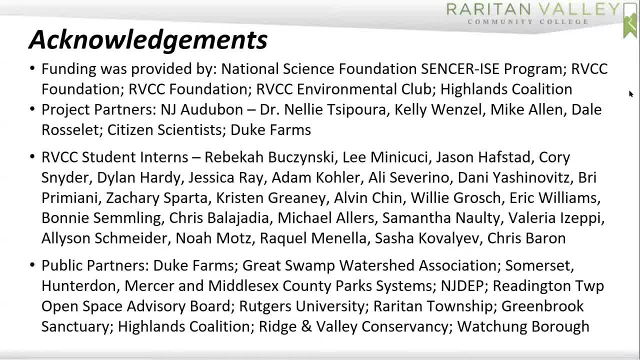 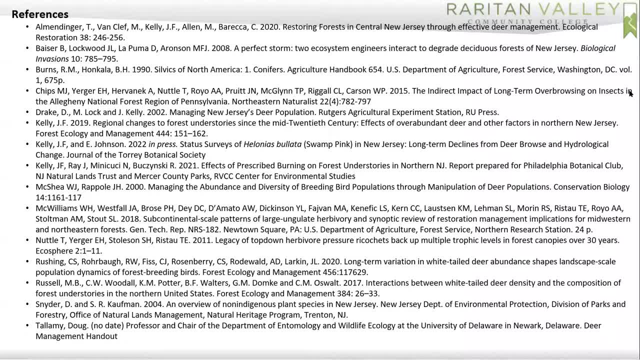 their forests or, in some cases, providing resources to help pay our interns to get this work done, And I owe them a lot of thanks as well. Some of the research that was cited in the study is here in case you wanna look more into it. 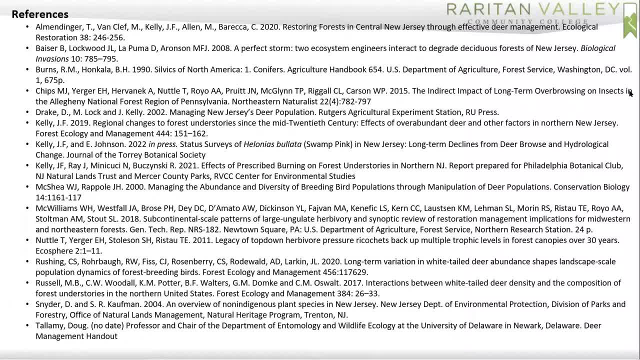 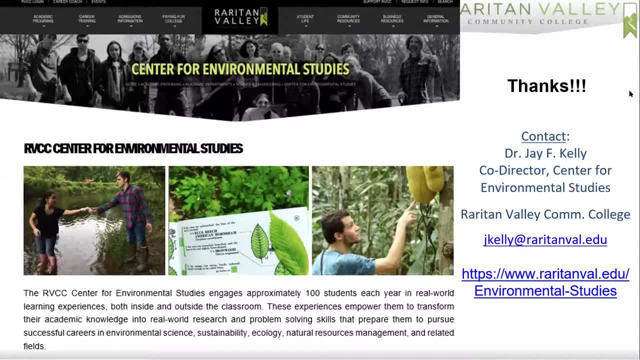 And I can provide you with any additional literature that you might be interested in if you wanna look into these complex issues in more detail. Best way to get in touch with me is by email, And we are creating a website so you can see all the other fun stuff. 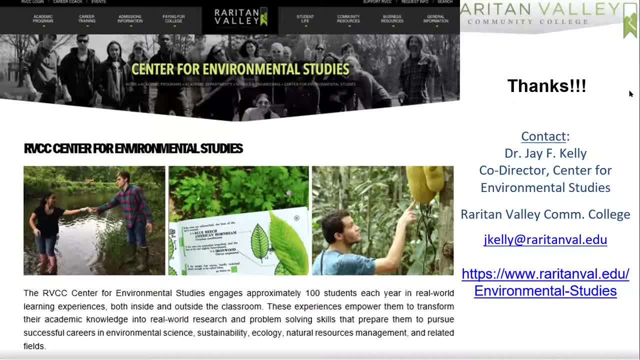 we're getting ourselves into in the world of plant conservation and research in New Jersey. So, before I take questions, Hubert asked me to give you a little bit of information about this new partnership that we've created with them on sea beach amaranth conservation. 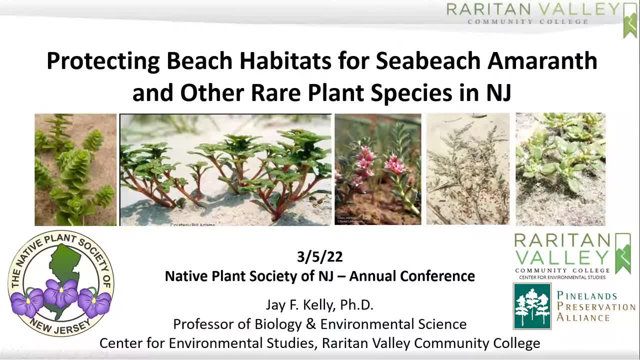 So I'll try to give you a little bit of backstory as quickly as possible. We've been working on coastal plant conservation for 20 years at this point, And this year we're engaging in a partnership with the Native Plant Society to team up and try to do even more to protect our coastal beach species. 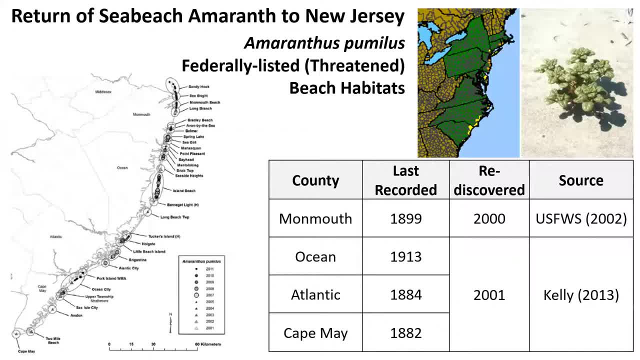 Sea beach amaranth in particular, is a federally threatened plant species that occurs on beach habitats in the mid Atlantic, And it's an exciting species to work with because for a hundred years it was gone from New Jersey. It hadn't been seen since 1913. 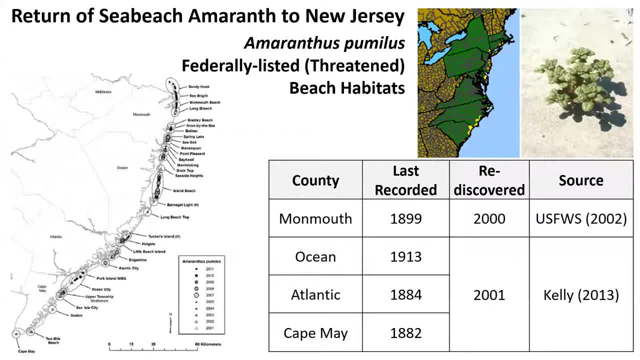 And in the year 2000,. it reappeared in Monmouth County up by Sandy Hook. The following year I was sent to survey the rest of the beaches in the state, and we found it in all the other coastal counties as well, And so we've been every year doing surveys for this species. 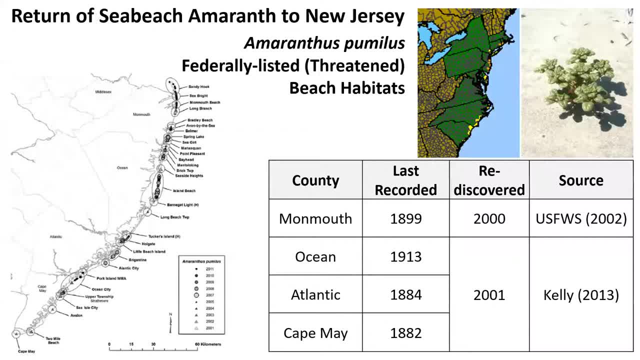 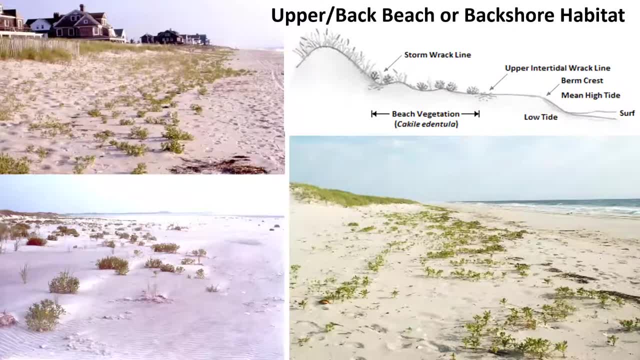 and for other coastal rare plants, and trying to protect the habitat so that it has a chance of sticking around and hopefully increasing into the future. Sea beach amaranth occurs only in this narrow strip of land above the high tide line and up to the foot of the dunes. 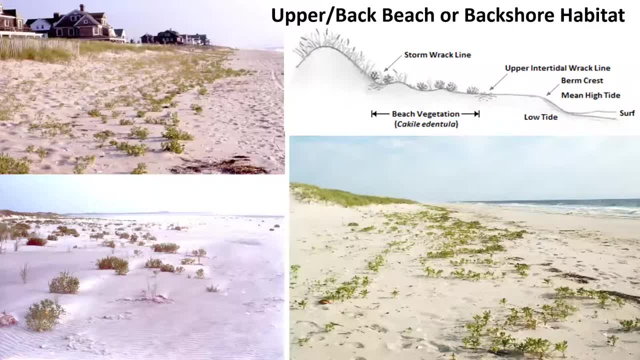 It won't grow in the dunes at all, It's just on that upper beach surface. It's an annual plant and it travels by wind and waves, And so wherever it occurs one year, there's no guarantee it's gonna be there the next. 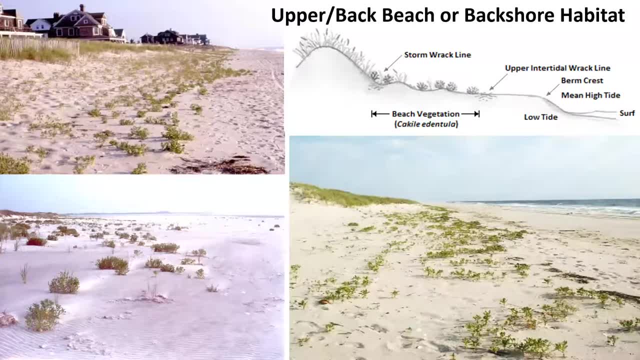 And it could appear a mile down the coastline or even farther, And unfortunately, of course, in a place like New Jersey. these habitats are subjected to all sorts of human impacts. Some of the more important human activities that are affecting sea beach amaranth. 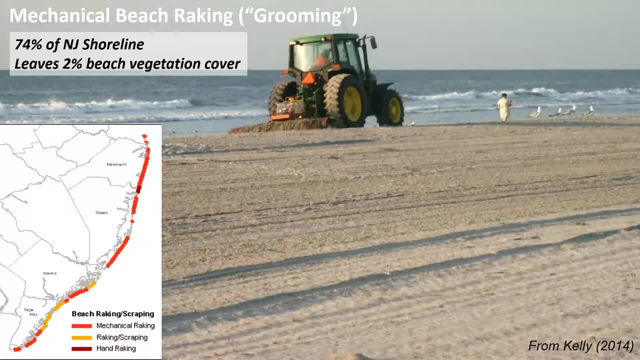 and these habitats in general are beach raking or grooming, which occurs on all the recreational shorelines of the state. Trackers and other tools are used to groom the surface of the beach every morning to prepare it for beach goers, And that, of course, destroys any plants. 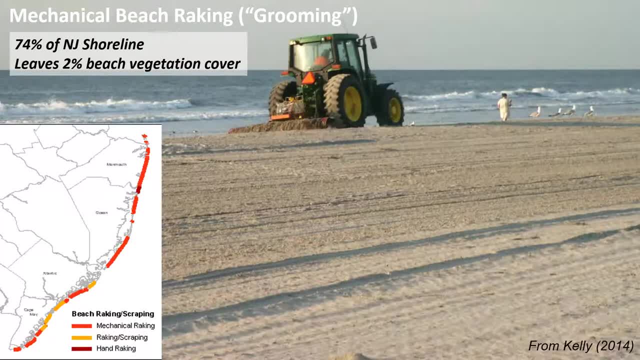 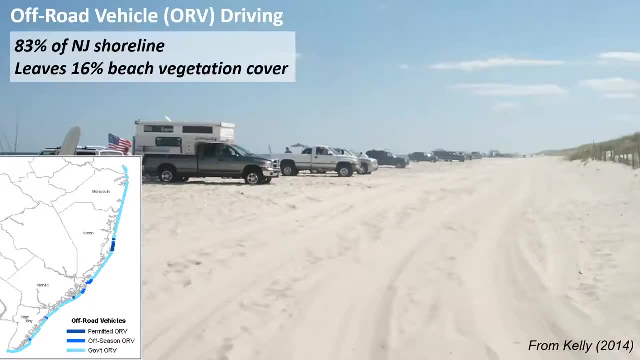 that are trying to grow on the beach, or beach nesting birds for that matter- And this is occurring on about 75% of all the beaches in New Jersey. Even more widespread is off-road vehicle driving, either for official uses by park staff or municipal staff. 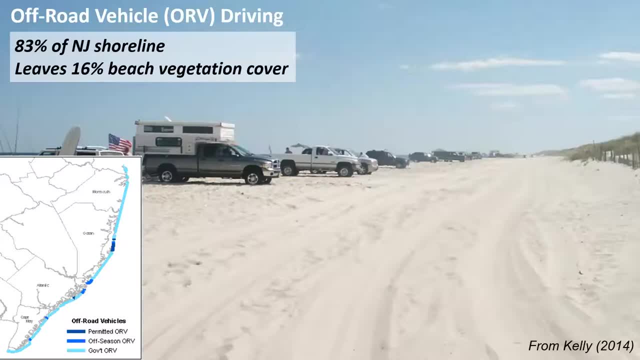 or for garbage collection and public safety, or for recreational use for sport fishing. Over 80% of our beaches are affected by these activities And there's no better place to see the impacts of off-road vehicle use than Island Beach State Park In their northern natural area. 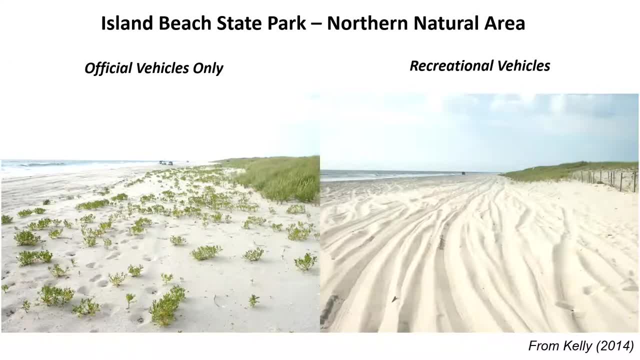 recreational driving is restricted and only park rangers are able to drive up there And you can see really lush beach vegetation growing in those places. Immediately to the south of the northern natural area it's open to recreational vehicle use. You can see the beaches are rutted with tire tracks. 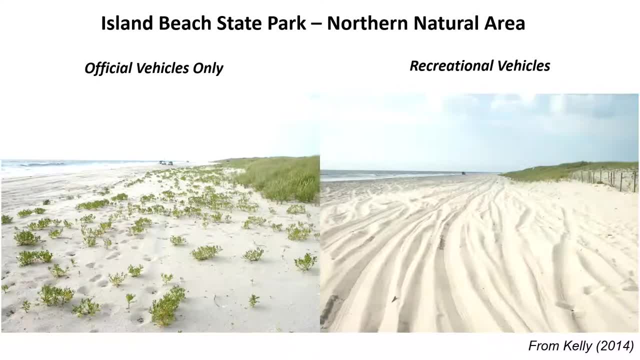 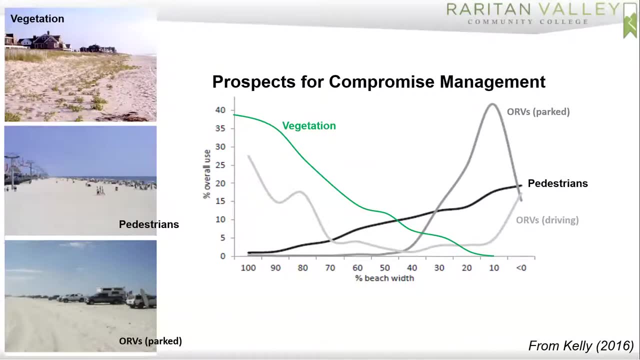 and there's no vegetation- amaranth or otherwise- growing in these beaches. So the good news is that there's really strong room for compromise to improve natural resource benefits in these beaches, because the upper parts of the beach are rarely used by people. 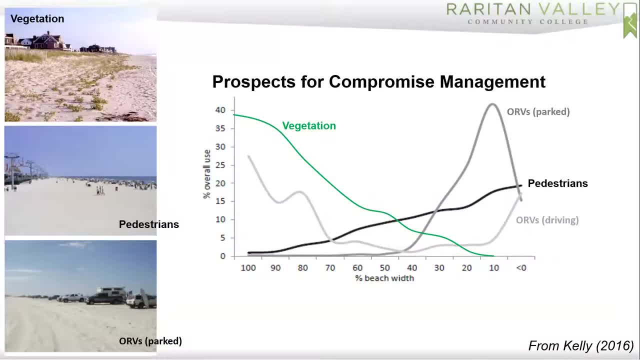 So we did some research on peak tourist days throughout the year, looking at where people were located on the beach surface, And you can see in Seaside Heights there in the central photo the places that would be occupied by plants have been raked clean. 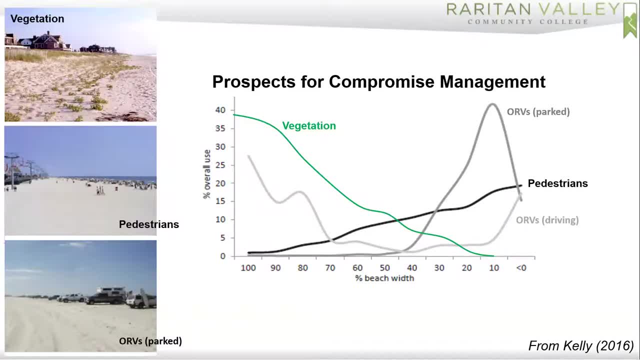 but people aren't really using those parts of the beaches, And the same is true for the places where people are driving on the beaches as well. So we can potentially protect the upper parts of the beach and allow for these plant species to occur there. 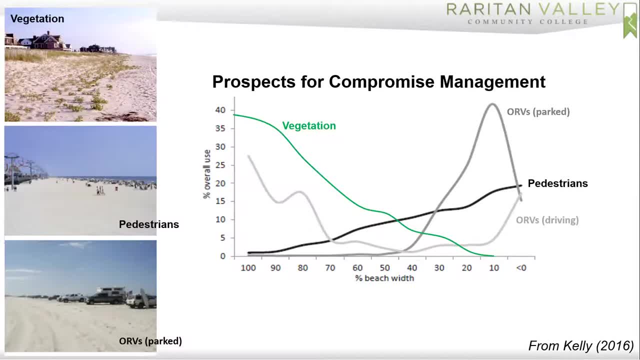 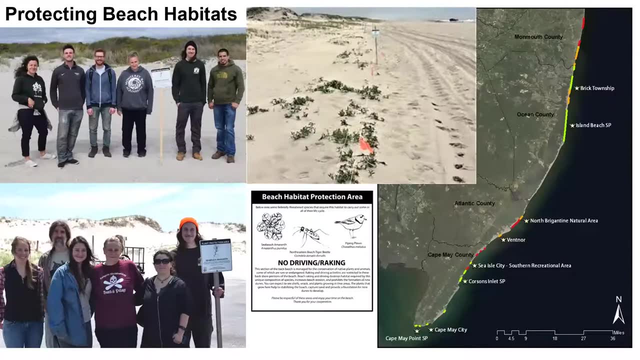 while at the same time still allowing for recreational uses to occur, which are so important economically and culturally in New Jersey. And so we've been doing that for the past 15 years, working with partners like Pinelands Preservation Alliance, the state parks and other groups to try to keep people. 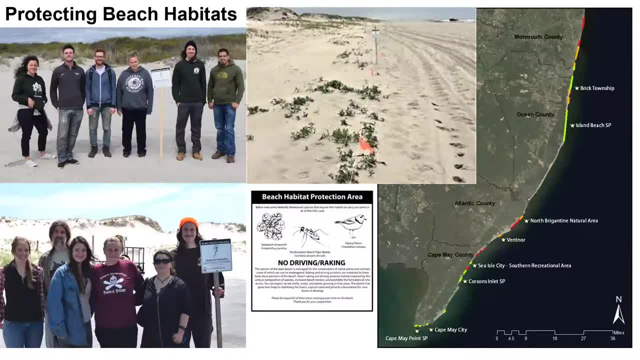 from driving on the upper parts of the beach, And the beauty of this is that it's really cheap. It costs about a hundred dollars for a mile of protection. You put a stake in the ground and tie some string between the stakes, and all the seeds wash back up. 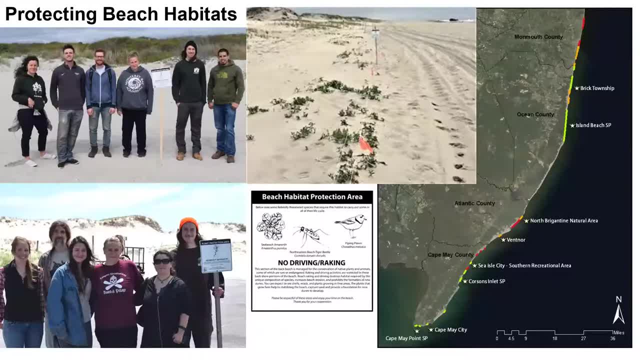 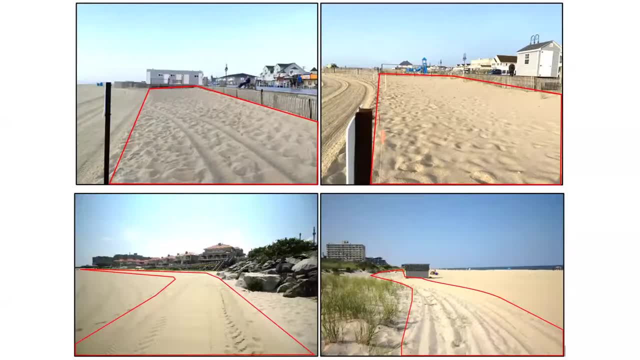 on their own. You don't have to do any planting whatsoever, And so this has been really successful. We're working in about 20% of the New Jersey coastline at this point doing these kinds of activities. We're also monitoring townships and parks. 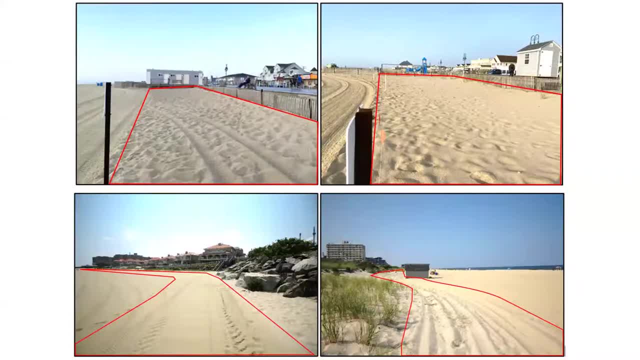 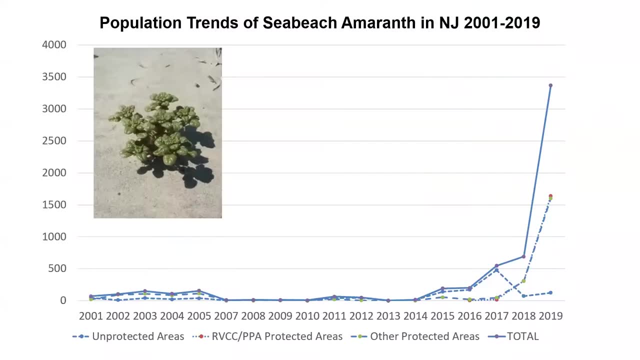 where there's agreements in place with the state government to make sure that the protections that are parts of the beach that are supposed to be protected are actually getting protected, And that doesn't always work out that way, But what we've seen since we've engaged in these activities. 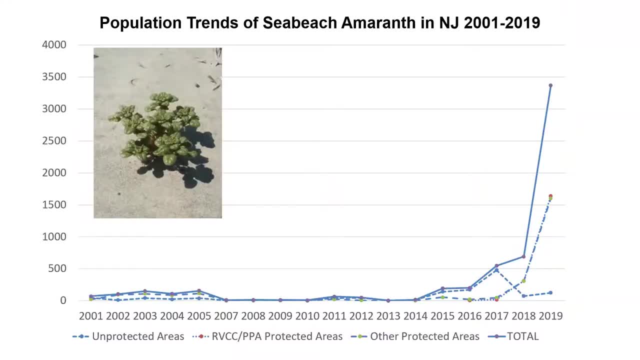 are. Sea Beach Amaranth, in particular, has really responded dramatically to these improvements in habitat, increasing several hundred fold from the low levels that we observed through most of the past 20 years, And again with no more effort than just putting stakes in the ground with volunteers. 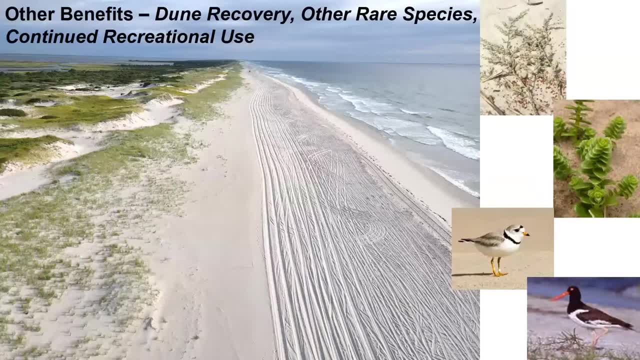 and letting nature do the rest of the work for you. The other benefits that you get from this are: these beach species are also the first step in dune succession, So as soon as the plants get established on the beach surface, they anchor the sediment in place. 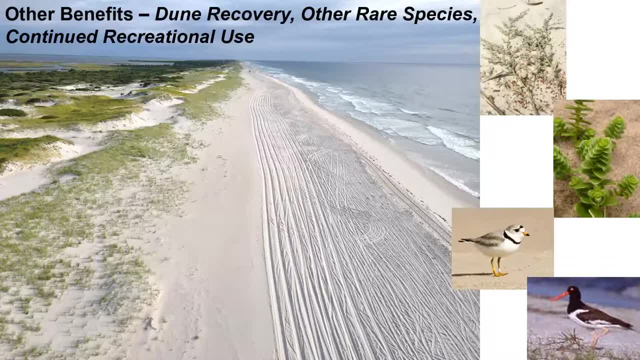 and they start to accumulate sand that gets blown in the wind, And so, a few years after those plants establish, you typically get low-lying dunes occurring, And so this is an aerial image from one of our drones at Island Beach State Park. 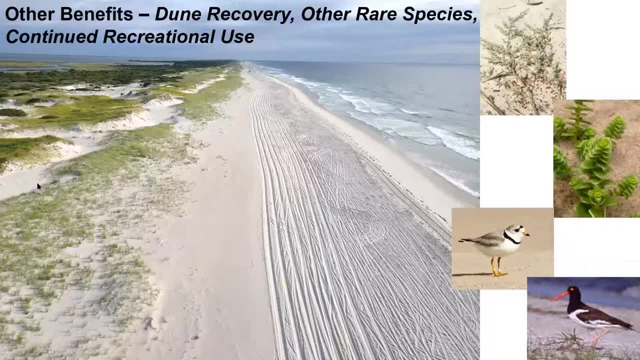 And you can see here this whole strip of dunes that are growing at the foot of the larger four dunes on the left has all come in completely naturally as a result of these efforts of us putting these posts in the ground since Island Beach has been since 2008.. 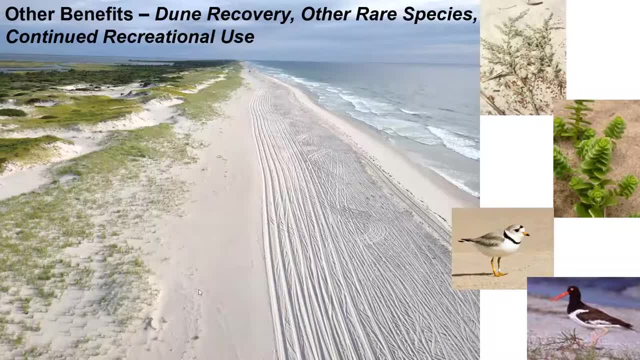 You know, this would cost millions and millions of dollars if we had done this, artificially constructing the dunes and planting the beach grass. But just by putting these wood stakes in the ground and keeping people from driving on the beaches, the dunes have recovered entirely all on their own. 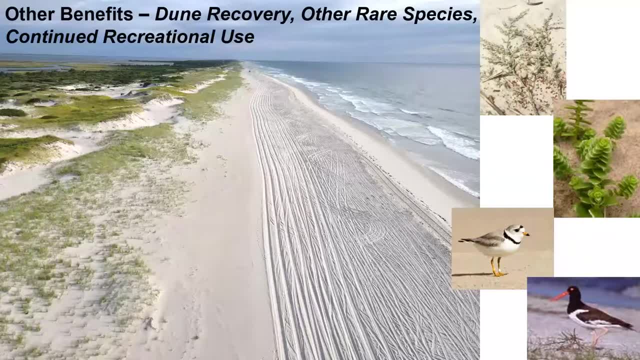 since Hurricane Sandy came through in 2012 with no additional effort, And in addition to the dunes recovering, we've seen other rare plant species like sea beach knotweed and sandwort coming back. The beach nesting birds have come back to Island Beach State Park. 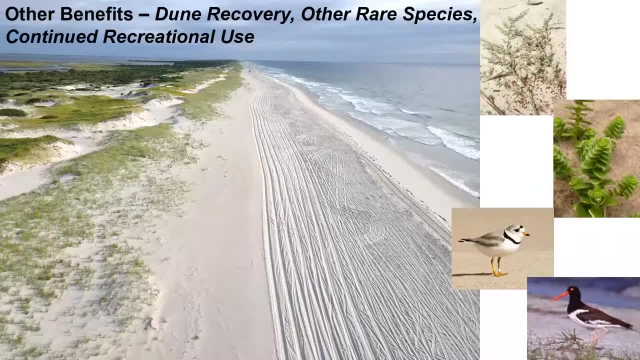 in places where they hadn't been seen in more than 20 years. And so nature does all the work for us if we just, you know, pull back on those limiting factors that are preventing that restoration from occurring or recovery from occurring. There's been a really nice story map put together. 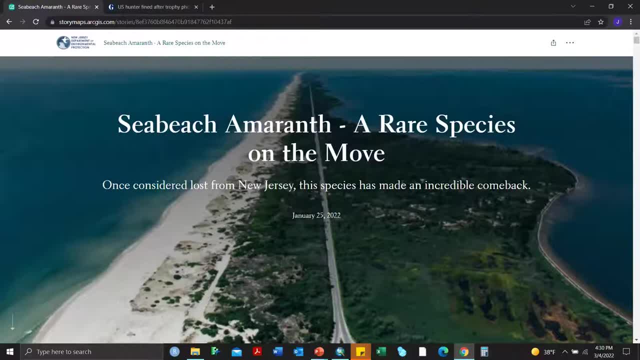 by the NJDEP on Sea Beach Amaranth and these coastal dynamics in the past couple months that I'd encourage you to take a look at. It's really informative and full of lots of great historical information about shoreline change and Sea Beach Amaranth and the state. 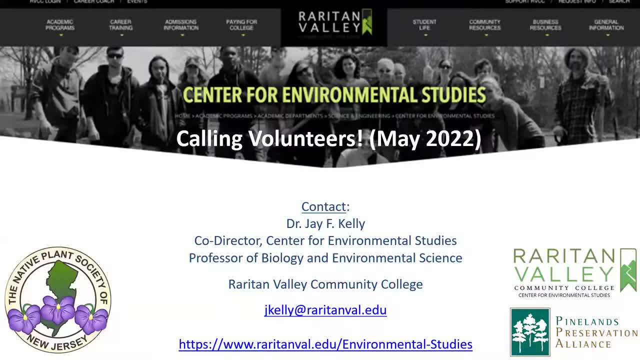 And you can find that online. Here's my contact info. We're going to be looking for volunteers very soon to go install these beach fences around the state to try to protect our rare beach plant species and dune development, And we'd really love to have some folks from the society. 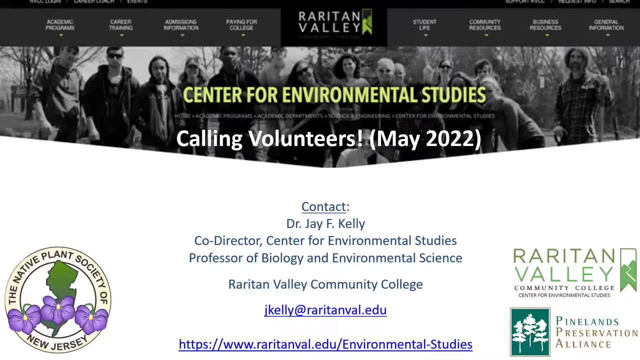 in your membership to come out and join us. It's a lot of fun out there and we could certainly use more help because we got a lot of ground to cover. So thank you for all your attention and interest And if there's time I'll be happy to answer. 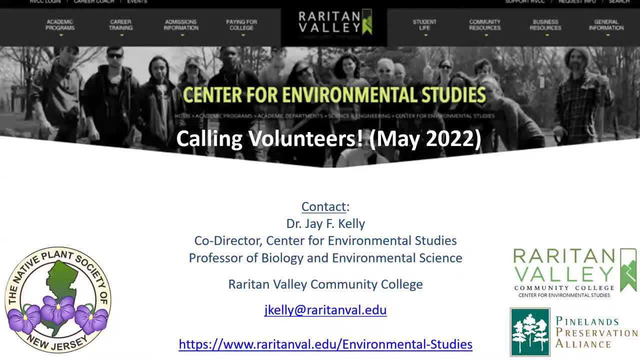 any questions you might have. Okay, well, let's see, We have A little bit of time. Okay, we're till 12.30.. Okay, Oh, okay, We have quite a bit of time. All right, We have a whole bunch of questions. 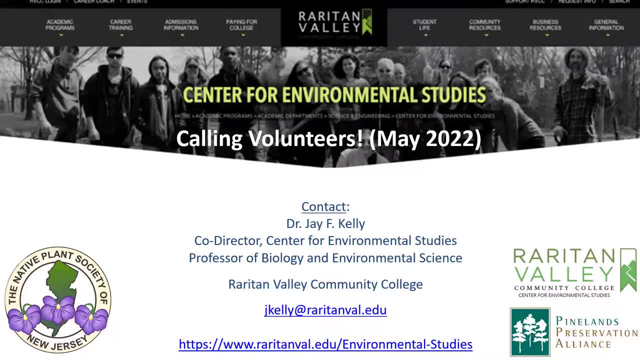 and I think Kim is going to work on the chat And she has done some already, but did you want to say anything, Kim? Well, okay, I'll go ahead with some of these questions here first and Kim can think of anything that she wants to say. 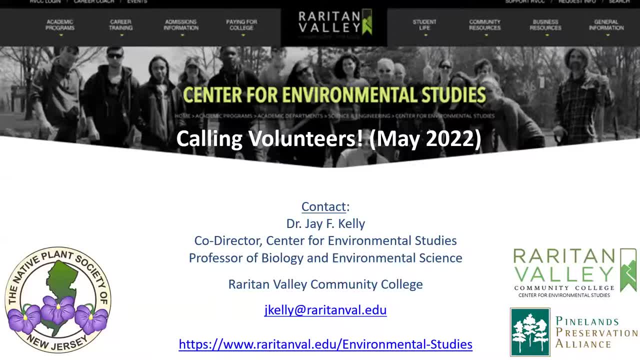 What kind of state response do we have to the The deer problem? Are they looking at it or are they thinking about doing anything? What's happening? It's variable. It depends which part of the state government you're considering: The Division of Fish and Wildlife. 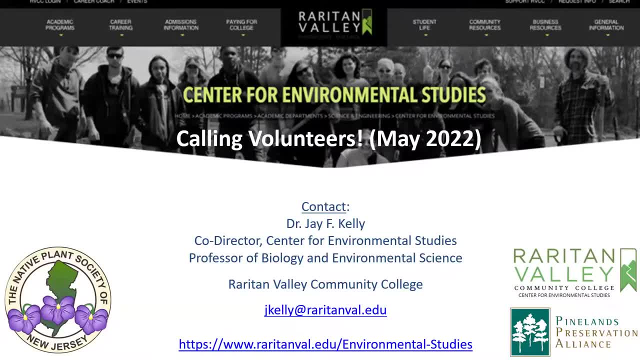 has a number of different tools that farmers in particular can rely upon. They can get depredation permits to help reduce populations on their farms. There's grants available through NRCS and other sources to put up deer fencing around farms, And so farmers have gotten a lot of support. 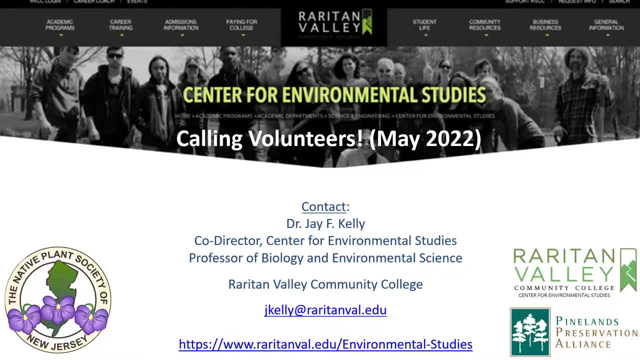 and attention that they need. for sure, There's been less effective policies in place to benefit natural areas of various kinds. The same kinds of tools could do a lot of good in those places, but there aren't always the same sorts of policy solutions in place. 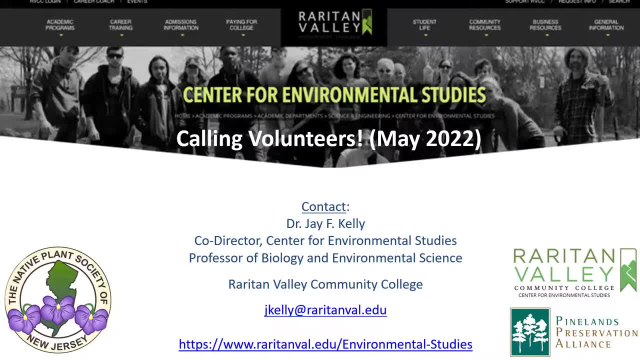 whether it's depredation permits or resources to help fund deer exclosures. The division as a whole has recognized the impacts that deer are having on forest environments, but in many parts of the state their policies that they're implementing are still designed to actually increase deer populations. 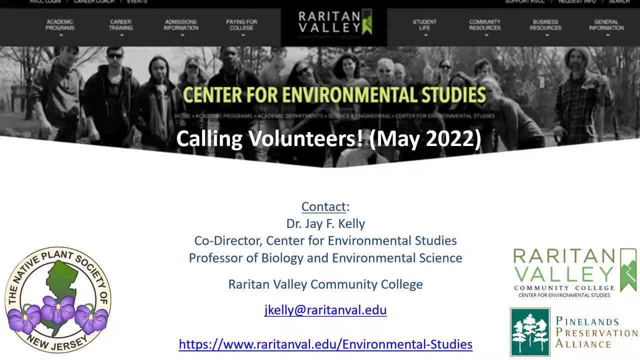 And so they do have a toolbox available for local townships and landholders to try to tackle deer populations locally, but I don't think that they're taking the issue seriously enough as they need to at the state level, where these impacts are happening, And different approaches really should be taken. 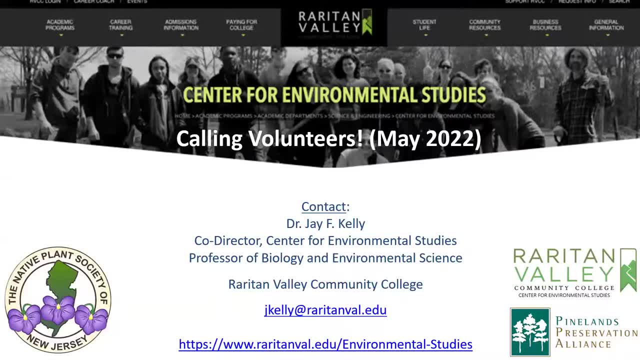 A lot of their efforts have been focused on opening up areas to hunting, which is a really important first step that a lot of communities need to consider to try to address the problem. But, as we've talked about, recreational hunting alone is not likely to bring down the deer population in any meaningful way. 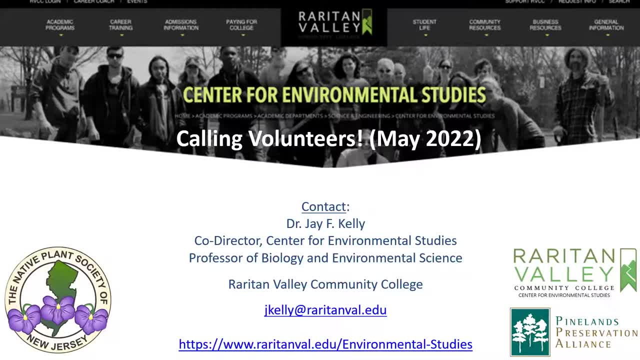 for these kinds of environmental benefits that we're interested in, And so we really need to think more broadly about other kinds of solutions, And I haven't seen the same kinds of positive responses to those ideas coming from the state level, unfortunately. One person asked: 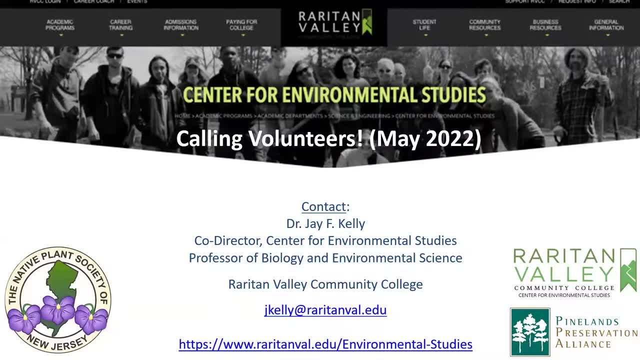 why doesn't the recreational hunting work any better? Is it just because we have too many limits, too many regulations for the recreational hunting, And could we really relax some of those regulations? No, New Jersey actually has some of the most liberal hunting regulations in the country. 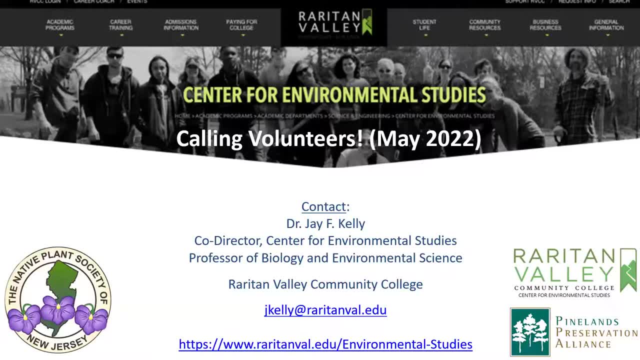 We have a hunting season that extends from mid-September to mid-February in most parts of the state, with a whole host of different tools that you can use as a hunter to harvest deer. There has been, I think, somewhat of a decline of hunters. 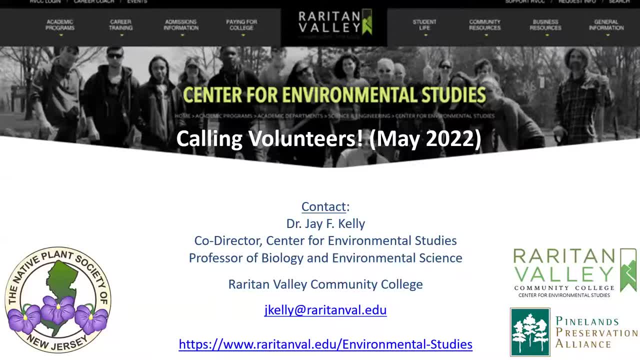 and interest in hunting compared to historic levels. that factors into this, But the bigger problem is that I think people don't spend as much time hunting as they used to. It takes a lot of work to kill a deer, Even the people that are most skilled at hunting. 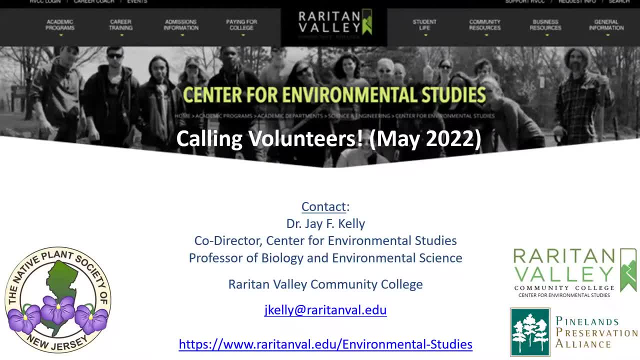 I've heard from Mike Van Cleft, working at Fovos, that his hunters that are really skilled and know what they're doing. it takes on average about nine to 10 hours worth of work to get a single deer, And so if you've got a population, 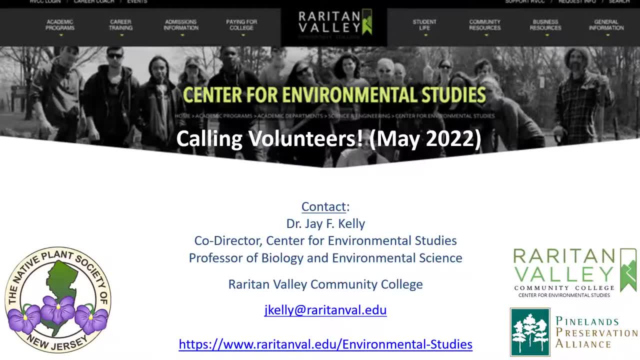 where you're trying to reduce the deer population by hundreds. that's a full-time job for several people to try to bring down the deer population And people- recreational hunters- just don't have that luxury to go spending all their time in the woods. 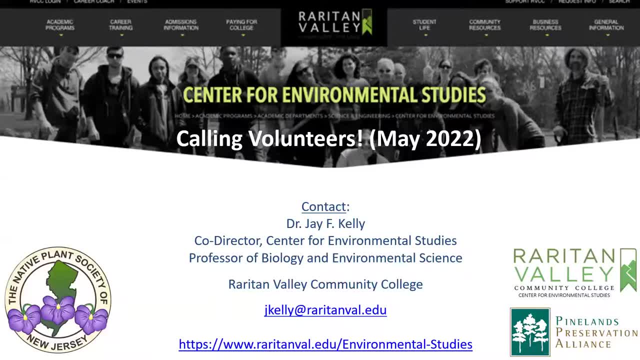 to benefit the public good in this way. Most hunters are just trying to get a deer or two to fill their fridge. put a trophy on the wall and maybe in some cases, if they get extra deer, they'll donate them to hunters helping the hungry. 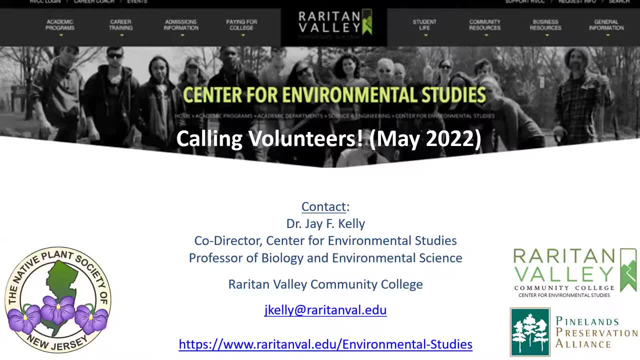 But the amount of work that's required to really tackle the deer populations that we're seeing requires far more time and energy and resources that we can really expect from our hunters. It just wouldn't be fair to expect private hunters to be putting all the weight of this work. 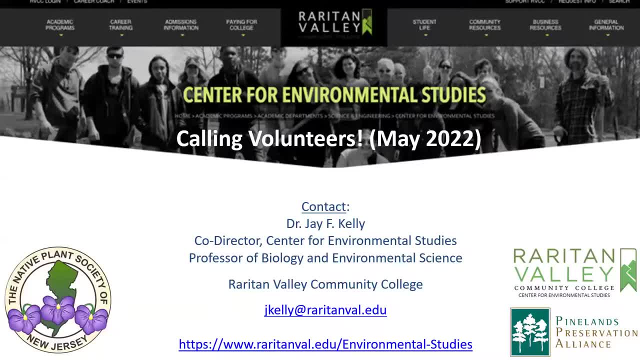 on their own shoulders when there's no economic benefits or advantages necessarily for them to engage in it. And that's why opening up market hunting, potentially so that they can actually have an incentive to take extra deer and put the work into it that's involved, so they could sell the meat to local restaurants. 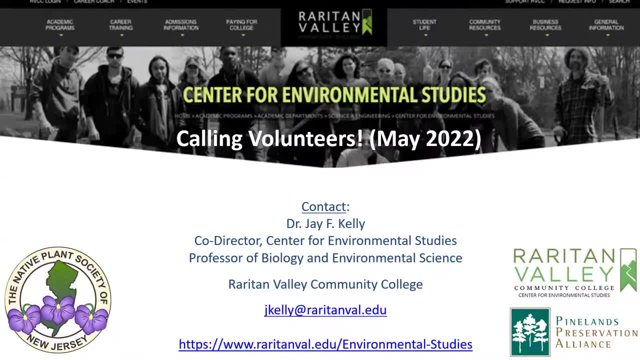 that would be a potential solution that could make better use of recreational hunters and the services that they're providing- because they are services. It's just not incentivized in the right sort of way that we can expect the kinds of- I guess- reductions to take place that we need. 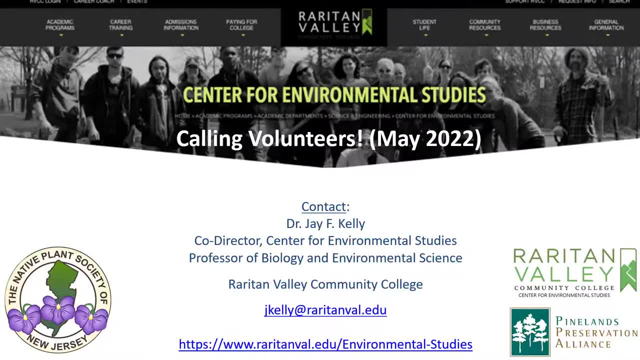 We have another question on the deer wasting disease and possibly other diseases from deer. Would that be a problem in expanding the deer as a market commodity? It could be The chronic wasting disease. there's no record of it yet in New Jersey, but we do have other diseases. 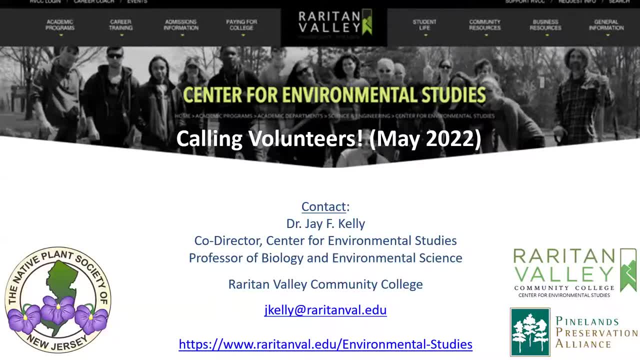 EHD and blue tongue and other diseases that are affecting deer populations locally. You know I'm no specialist on wildlife diseases and we have no. you know there's no programs right now taking place that engage in these kinds of market incentives, So I would have to look to Europe. 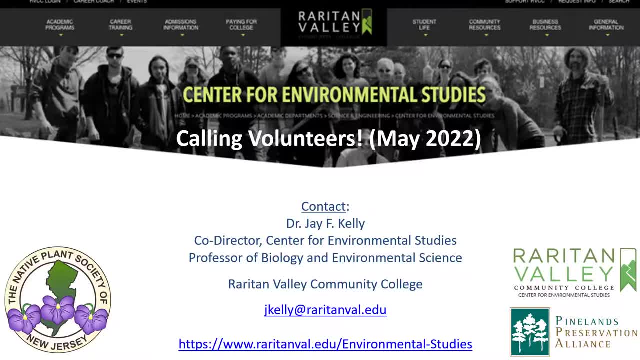 and these other countries that are engaging in these activities, because I'm sure there's diseases affecting those populations elsewhere And you know, again, the benefits of market solutions is that creates a revenue stream that could be used to monitor or deer populations the prevalence of these diseases. 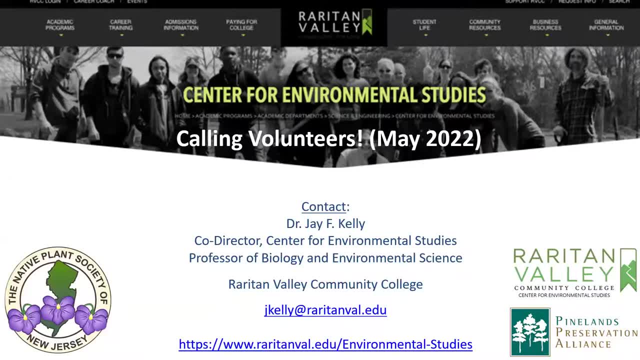 that could be tested before they get sold, for example. So there's all kinds of ways that resources could be made available to tackle those sorts of questions and concerns, which are legitimate concerns, But I don't think we have any evidence, unfortunately. 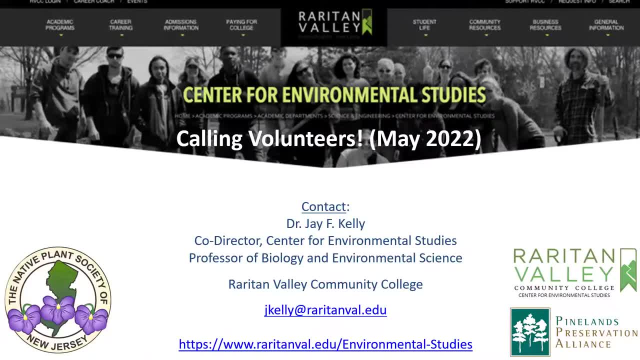 at this point, to draw from, at least on this continent. So I don't have any other answer than that, And so the articles that I put on one of the slides here have really nice surveys of these programs from around the world. So look to those as potential resources. 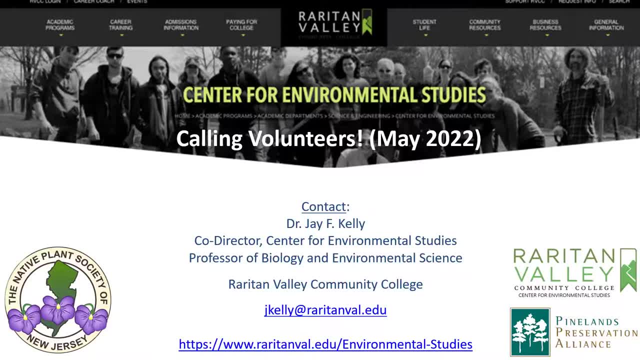 to answer some of those questions. OK, and it's being recorded so that should be available for them, And I'd be happy to share the PDF to anybody that wants the presentation as well. OK, thanks. People asked how can they help right now? 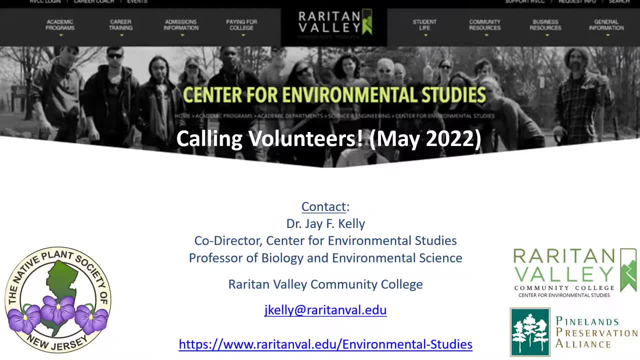 Is there some steps that they could take to alleviate the deer problem and make a positive impact? Yeah, I mean, this needs effort at every level. So, from the household level, thinking about how we can protect the properties that we own from the impacts of deer. 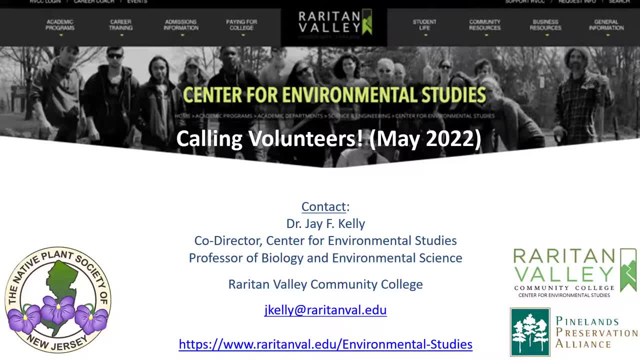 and providing little arcs to encourage native plant diversity, to improve and hopefully seed into surrounding areas. there are things that we can do at home, even at just that level, But in our communities there are things that you can engage in a larger scale- Most townships in central New Jersey. 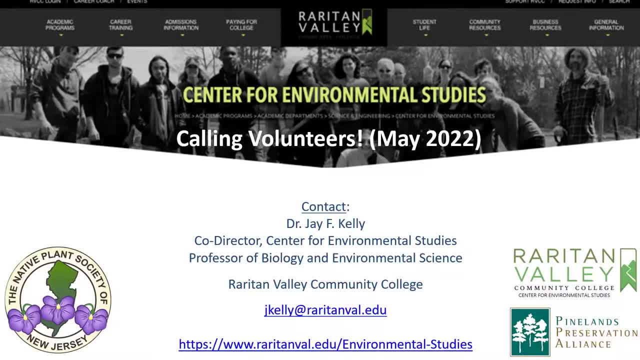 have several thousand acres of open space that they own that are not necessarily being managed for deer at all in some cases, And so making sure that your townships are doing their job at managing deer in their open space properties is a simple first step that can take place. 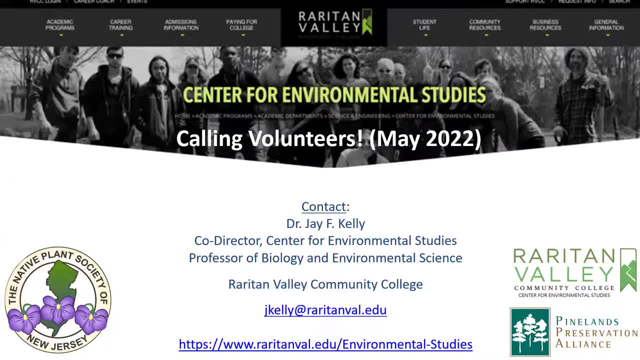 Many local townships still have ordinances on the books that prevent people from firing, from discharging firearms at all, even for hunting purposes, or from hunting using bow hunting as well. So making sure that the ordinances on the books and the local policies are in place. 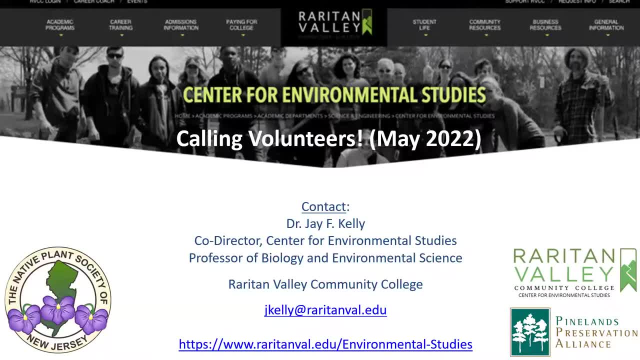 to try to tackle these problems, And that's something that we can all get involved in, pressuring our local officials or just getting involved through our local advisory boards. And then, of course, at the state level, the same sorts of concerns are in place. 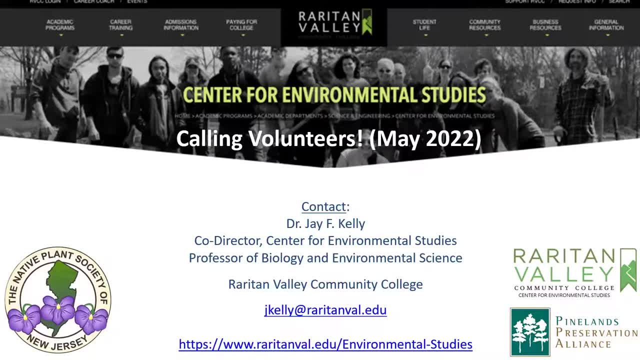 And so I'm working with groups like the Partnership for New Jersey Plant Conservation, New Jersey Conservation Foundation, the Farm Bureau in New Jersey, the Highlands Coalition, the Sourlands Conservancy. There are many groups that are really for decades have been concerned about this deer issue. 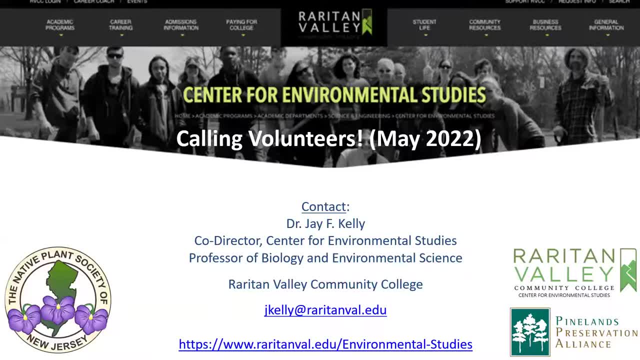 and have been interested in policy changes And hopefully in the next few years, with the right amount of public awareness and support for these new initiatives, we can see some meaningful change at that state level that we need the changes to occur. So 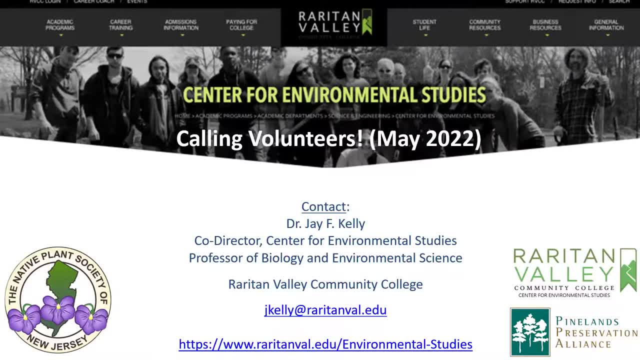 There's any number of ways that you can get involved at the different scales that you might find suits you or are available to you. How high do you suggest that a deer fence should be? It depends how big the disclosure is. If you've got a small exclosure where you're just trying to protect the plants next to your house or a small island of native plants in your yard. deer don't like to jump into enclosed places, And so I have a garden in my backyard and the fence is only four feet high and there's never been a deer jumping in. 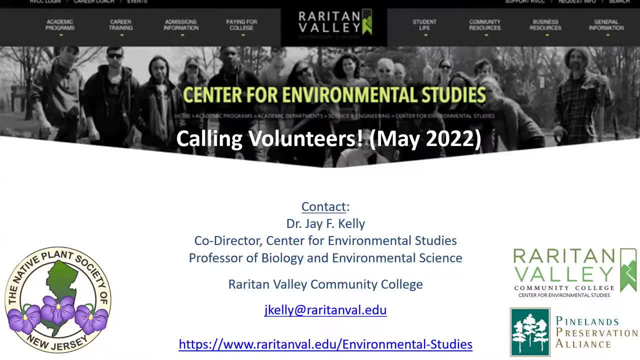 It's only about 20 feet by 20 feet. If you have a larger patch of woods or an area you're trying to protect, the recommendation typically is a minimum of eight feet, And deer can even jump over eight feet, So you're still going to have to monitor it. because sometimes they'll just barely make it and then drag the fence down. The other strategy is you can have a smaller fence, whether it's four or five feet, and then put a wire on the outside of that fence, whether it's an electric wire. or just a wire with flagging, And that'll keep the deer far away from the fence, that they can't easily gauge how high the fence is And it will also prevent them from jumping into the fence because they don't like to jump into those smaller spaces. between the wire and the fence. So it really depends on what you're trying to protect, But in general, if it's a large area, a minimum of eight feet is typically required. Hey, how would you answer the golden warbler question? 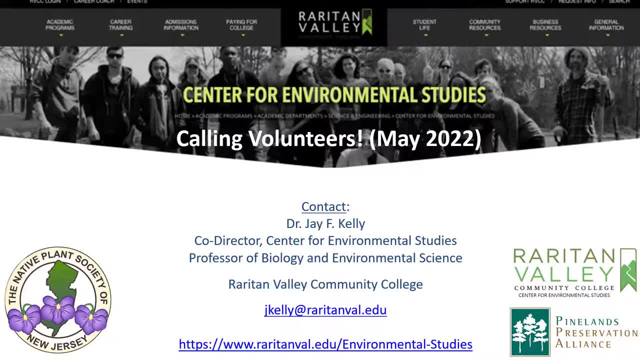 I'm not sure what the question is. Well, the question is that we have to chop down the mature forest in order to give the golden warbler room to grow and prosper. That might be necessary in some places. There are other things that we could do. first, 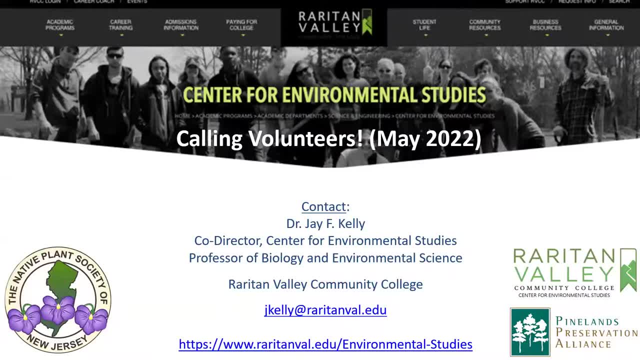 The golden wing warblers, for example, occurred in power lines in northern New Jersey, And one of the reasons for the decline has been the change in management policies of how the power lines are maintained, And by working with those companies we could potentially benefit the warbler in those places. 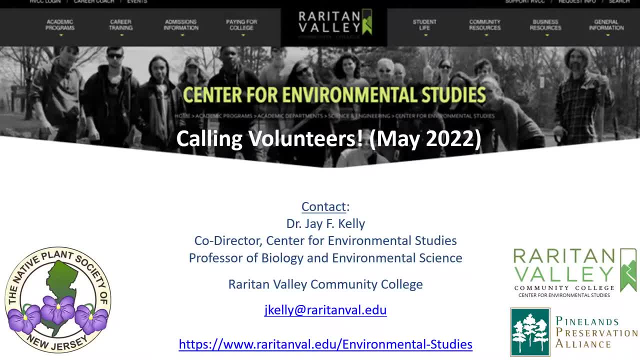 We can create it: Expanded habitat, clearcutting areas adjacent to those power lines to create some additional habitat for the warblers, And that's being done in places like Sparta Wildlife Management Area. But it's important to be smart about how we do that. 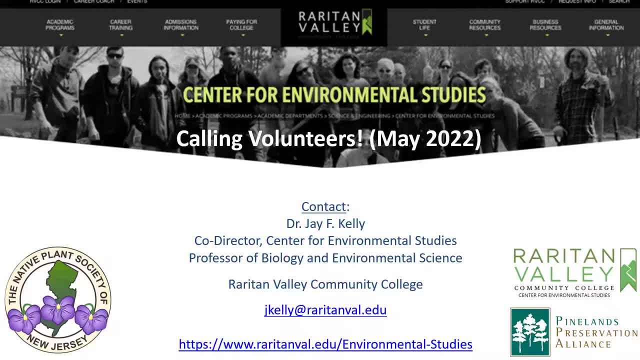 Make sure that you're not increasing edge for deer that's going to increase local deer populations or impact native wildflowers or rare plant species or other habitats and species of concern. So golden wing warbler deserves our attention. It's an important species that we're. 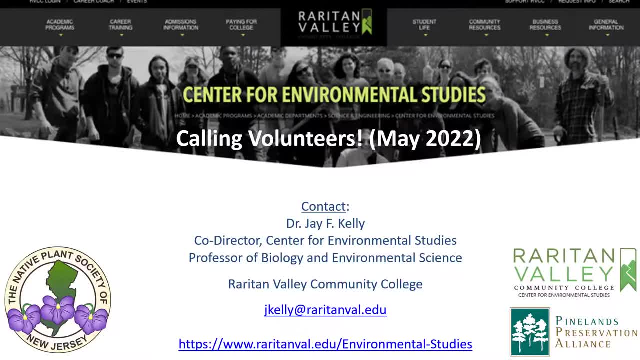 interested in protecting, And I think that the gold wing warbler is declining in our landscape And there are tools that we need to take to address it, But they don't necessarily need to be done in ways that are counterproductive for all the other kinds of things that we're concerned about. 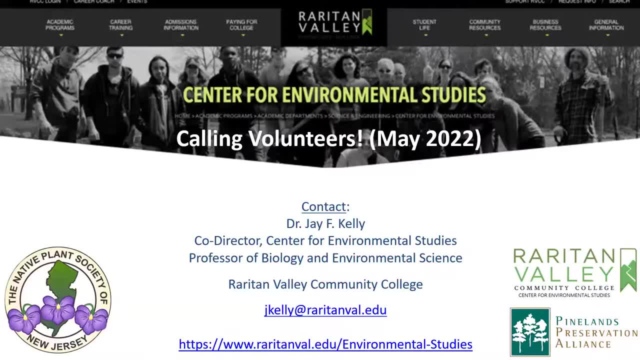 And those concerns need to be given, I think, equal levels of attention and effort. as the golden warbler OK. has any serious consideration been done for introducing carnivores, predators Or deer in New Jersey? Not to my knowledge. So after the successful introduction of wolves, 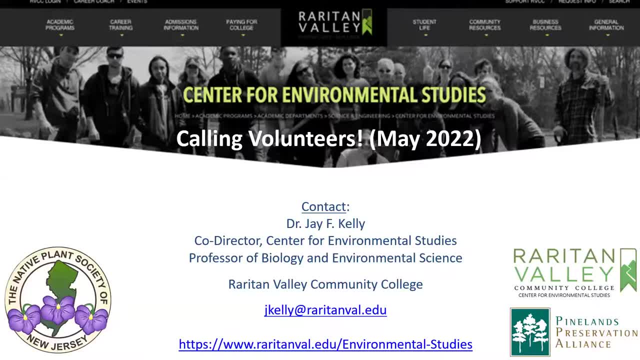 to Yellowstone. the Fish and Wildlife Service apparently tried to do the same thing in the Smoky Mountains in Western North Carolina And it wasn't successful, And, from what I understand, the reasons for that were a couple of factors, But one was that there are a lot of domestic dogs in the area. And the wolf population suffered from I don't know diseases of domestic dogs. They got distemper and other diseases that caused their populations to decline. The wolves also did not stay in the park. They went into the surrounding landscape, which caused problems. 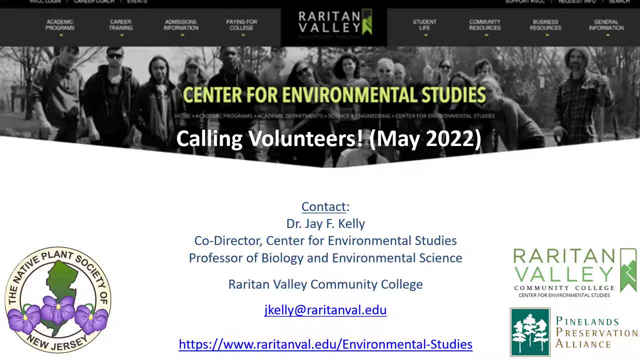 And they also interbred with domestic dogs, And so that's in a place like the Smoky Mountains, which is a much larger intact forest than we have in New Jersey, And so the prospects of wolves being introduced to New Jersey for me. 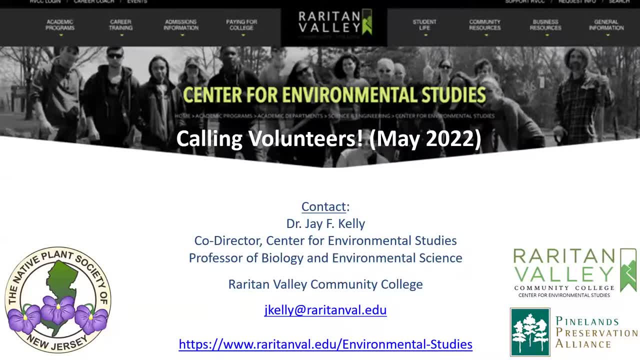 doesn't seem very hopeful. It might work way up in the Adirondacks or in New England, But around here it's hard to imagine that that could be successful. Cougars, on the other hand, I think could recover quite easily in New Jersey. They're much more secretive and solitary And they've arrived on their own. There was a cougar that appeared in Connecticut a couple of years ago. that got hit by a car And using genetics, they actually tracked it down to. I think it was a population in Montana or Wyoming. And it had traveled all the way across the continent entirely on its own, only to get hit by a car in Connecticut. There are also occasionally cougars that get released as pets People. I don't know why have cougars as pets and then realize: 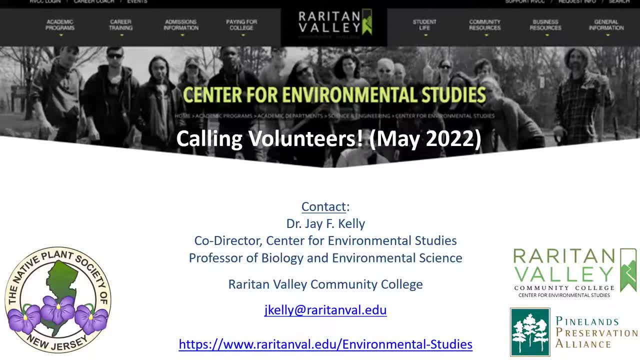 that's a bad idea when they get fully grown and then release them. So there was one in the Sourlands for a while that had been living there for a few years that I don't think there's any signs of recently. So I think there's some hope that cougars 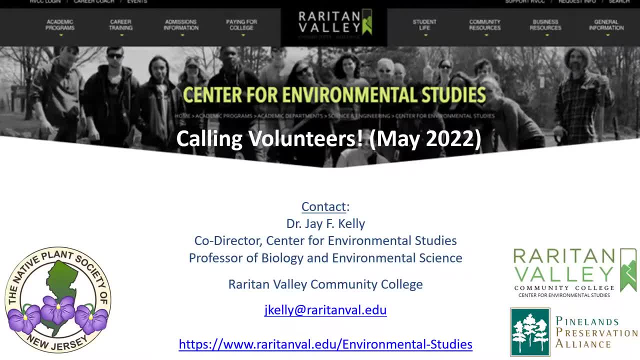 could be reintroduced into the landscape. But whether people would tolerate that's another question, Because cougars, unlike wolves, are actually predators of people as well as domestic animals and pets. So it's hard to imagine that people would accept the intentional reintroduction of cougars. 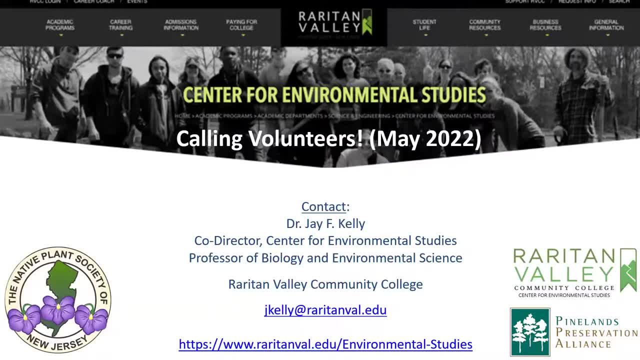 Maybe in time we'll see them return on their own And hopefully we'll be enlightened enough to figure out ways to tolerate that and to adapt ourselves to their presence. It's hard to imagine that wolves could be successful in these kinds of fragmented landscapes that. 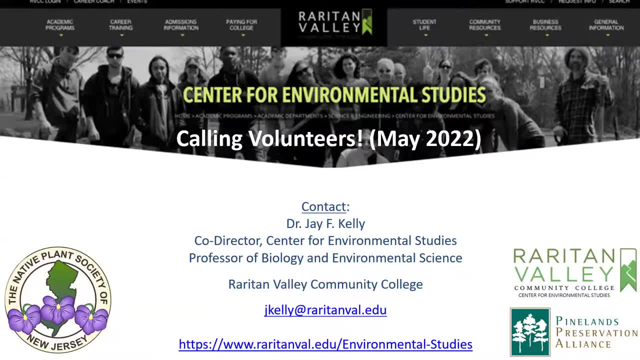 are so heavily populated by people and domestic dogs that they could actually recover here. But it's a world of possibilities And I think all those things are worth thinking about and considering and, in some cases, trying. Is there any word on deer birth control methods? The studies that I've seen in the literature show that that's a much more expensive means of deer management. We mentioned that sharpshooting costs about $200 to $300 per deer. Birth control can be upwards of $800 or $1,000 per deer. 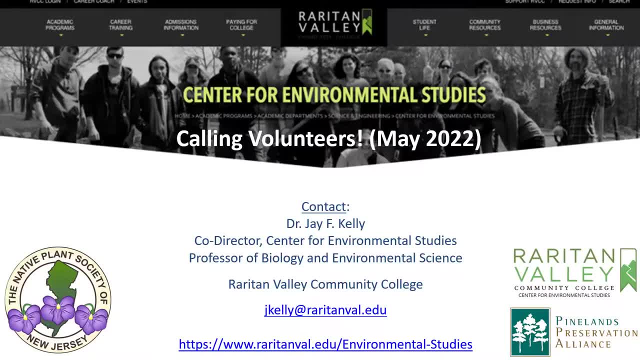 And the problem with birth control- at least the pharmaceuticals that have been approved for use in New Jersey and tested here- are that you need to re-inoculate the deer every couple of years, And so that means you have to tag the deer to figure out. 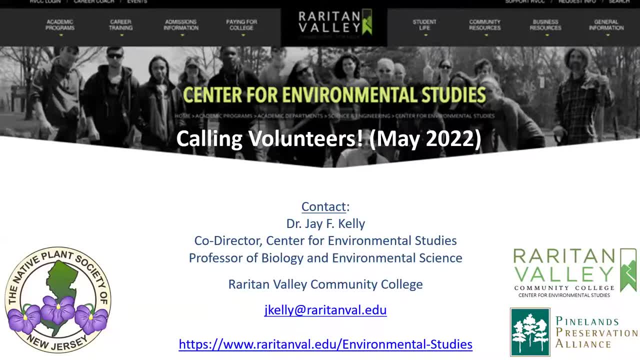 which ones you've inoculated, keep track of them, And so it's much more time intensive than just shooting a deer with a dart and walking away. You have to figure out which ones you've already shot, keep track of those, And so it's a much more intensive effort. that's. 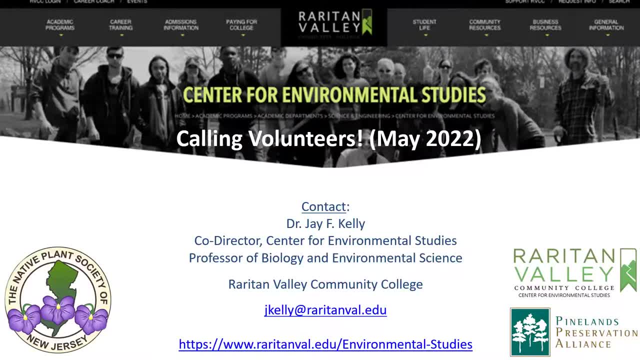 required. The pharmaceuticals themselves are often unreliable, And so, in general, it's not really, even for economic reasons alone, very feasible in the kinds of open landscapes that we have, And when we're talking about hundreds of thousands of deer that are occupying these areas. 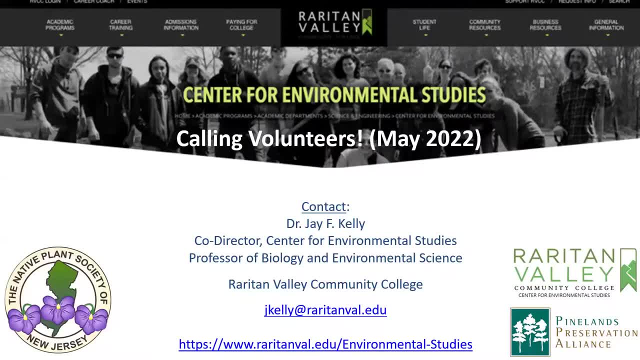 that we would have to begin to manage that way. Yeah, Yeah. So if you have a captive deer population in a zoo, then these kinds of pharmaceuticals can work really well to suppress reproduction. But in the open world, where you can't contain the deer, 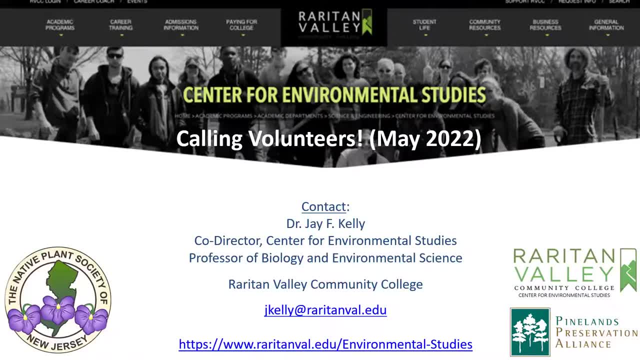 and you have to tag them and try to manage that deer moving across boundaries in ways that they do. it's not really feasible in the same sort of way. So there doesn't appear to me, at least with the current array of pharmaceuticals available. 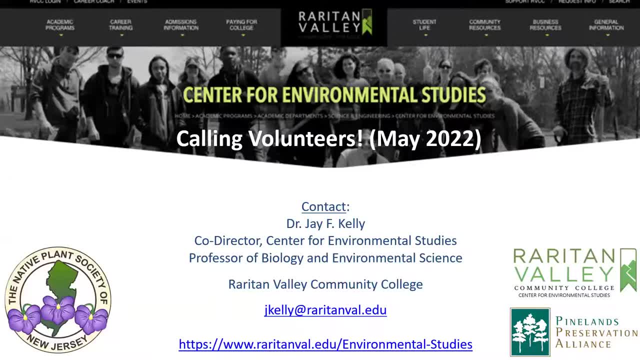 any hope for that being a strategy for deer management in the future. Well, how does the human activities- road building and house building- compare with the effect of deer pressure? human pressure compare with deer pressure on the native plant populations. Well, road building and those kinds of activities 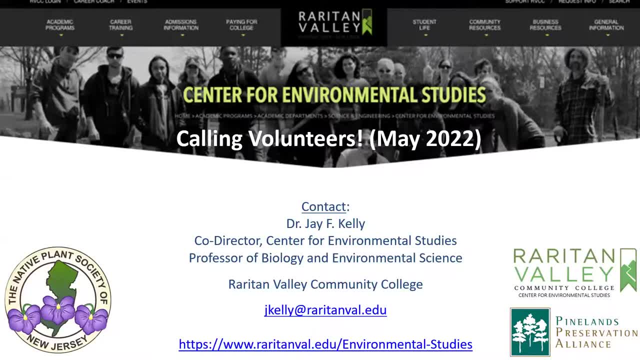 are important things to be aware of. The soil disturbance that's created by them favors invasive plant species. It creates forest fragmentation that favors deer populations and invasive plant species and leads to all kinds of other cascade effects. So it's an important issue to be aware of and to try to minimize. 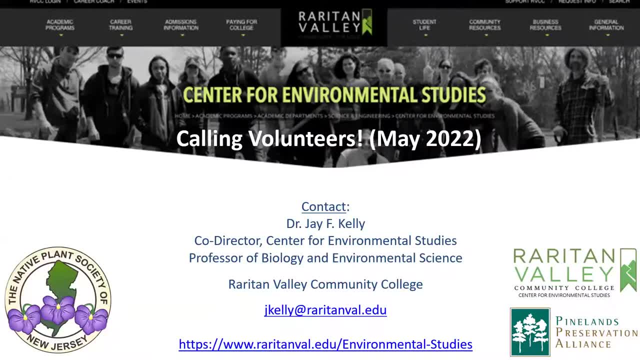 as much as possible, But deer are having impacts across the entire landscape, not just where the roads are located. They have free reign And they take advantage of that and have benefited as a result. So I think in terms of just the severity of impacts statewide, 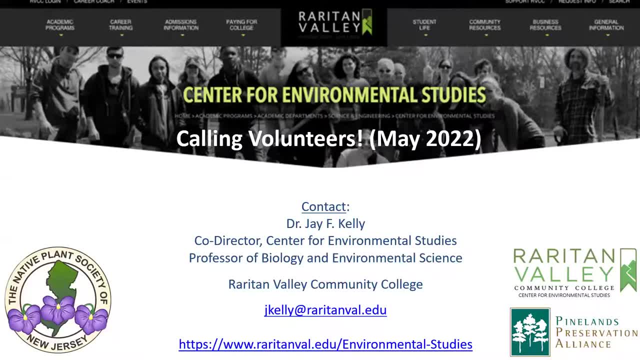 deer are having a much more pervasive impact on all the different kinds of ecosystems, not just forests in the state. The roads certainly do have impacts, especially on things like water quality and increasing sources of invasive plant species. Many of our roads are managed by herbicides now. 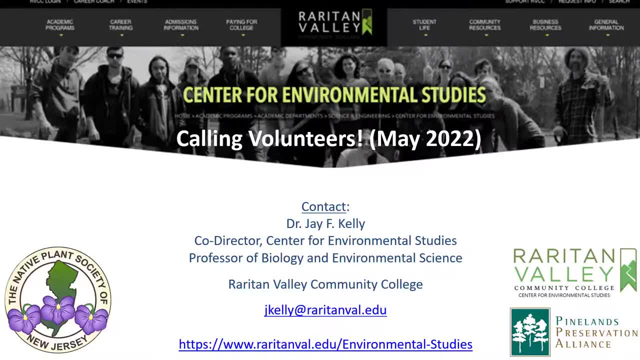 and that doesn't help our native plants either, and as well as fragmenting our forests. So they need to be taken seriously and efforts should be taken to minimize their impacts and to prevent them, as much as possible, from being put through new areas of open lands. 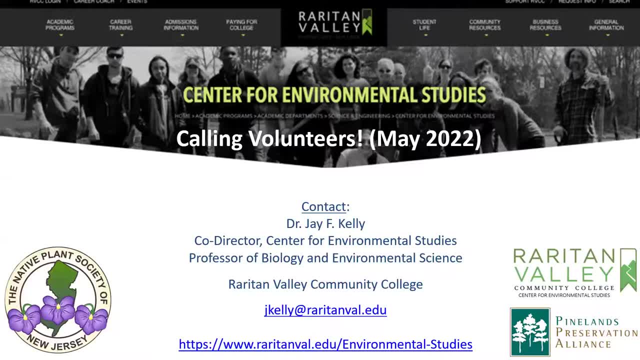 Thank you, I mean, and I don't think there's any longer possibility of deer being put through new areas of open lands, But I don't think they have anywhere near the same kinds of impacts as deer are having at the landscape level at this point. 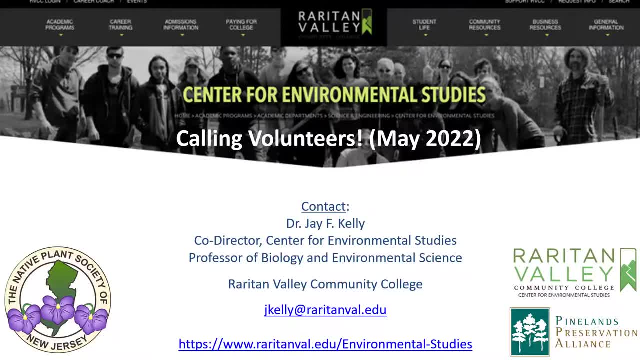 OK, Why aren't more environmentally-minded experts running for office? Maybe you should run. I think most people that are interested in how forest work want to spend their time in forests- things that our public officials have to do. unfortunately, There are really well-informed. 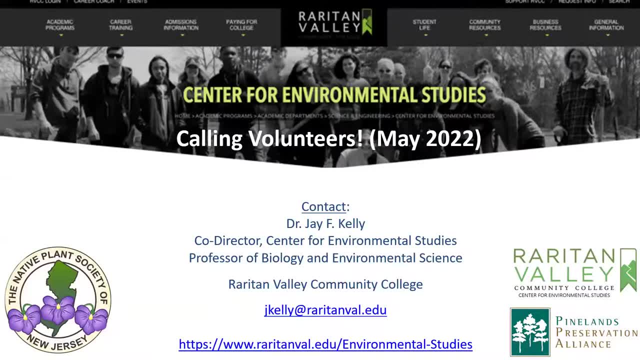 politicians out there, and it's important for us to support the ones that are already informed and to do our part to try and inform the ones that are not, at least the ones that are open-minded enough to listen, And I think there's still a lot of possibilities there, but we have to create. 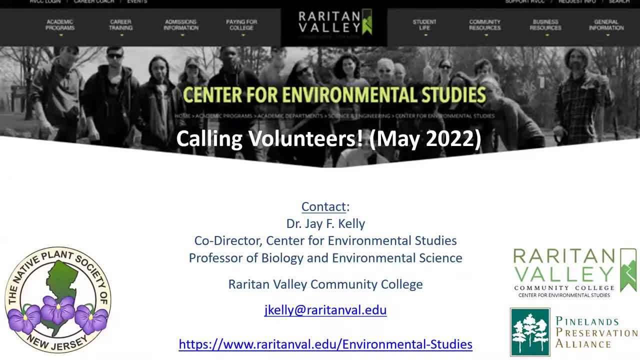 an environment where those public officials get positive reinforcement for making these kinds of decisions, because they're not necessarily popular, in some cases might be controversial or likely to invoke some kind of backlash- And as a constituency we need to have, I think, play a greater role in being advocates for these plant species that can't advocate for. 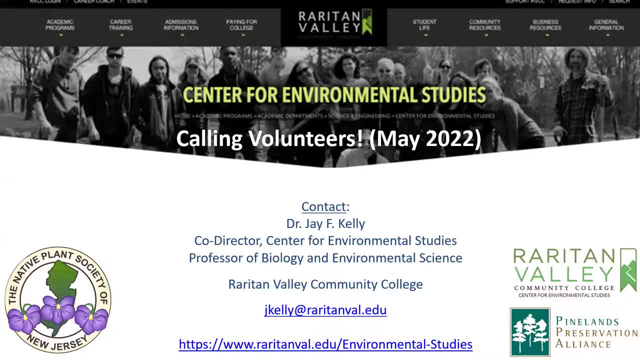 themselves and for the kinds of environmental restoration that we need to take place into the future. If future generations are going to have anything to do with this, we need to be able to do something about it. We need to be able to do anything worthwhile or anything like what we have today to enjoy. 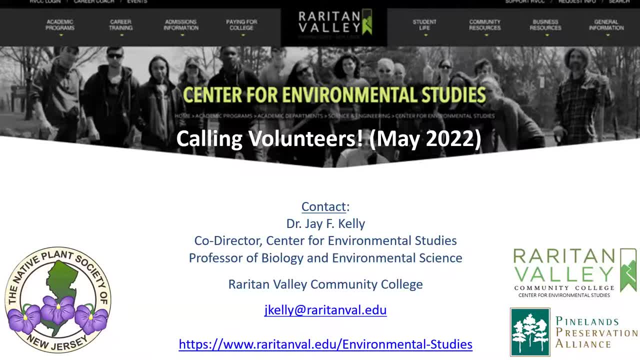 So, yeah, the more botanists that become politicians the better, but there's still plenty that we can do to educate our politicians and work with them to make the right decisions, regardless of what background we're coming from, because we all have something at stake here. 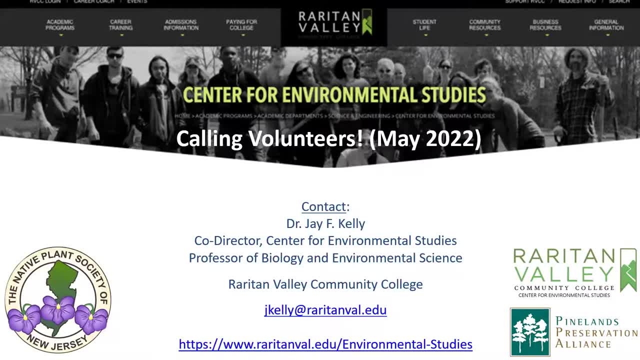 whether it's hitting a deer with our cars or trying to grow something in your yard or your farm. These impacts are really happening throughout society, not just with regard to our wildflowers and our birds in our forest. We have a lot going on in our environment that we need to Marshall. 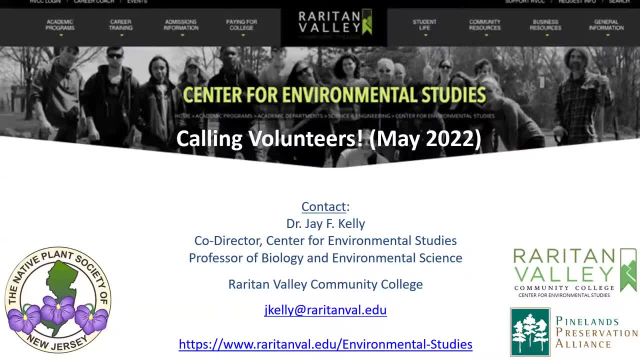 We need to do something about it And we need to do something about our forest And we need to do something about our natural resources that we care about. Can you recommend some trees to identify native trees, books to identify native trees and shrubs? 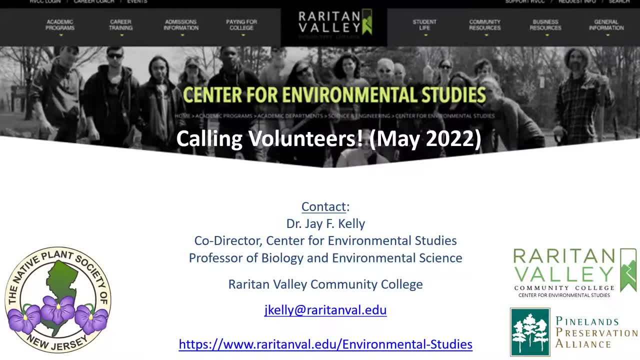 and tell which is native and which is invasive. Yeah, I'm seeing if I have some on my shelves right here. I don't. I think I have them in my lab right now, but there's some classic books. Maybe you could give us, send us a list or something. 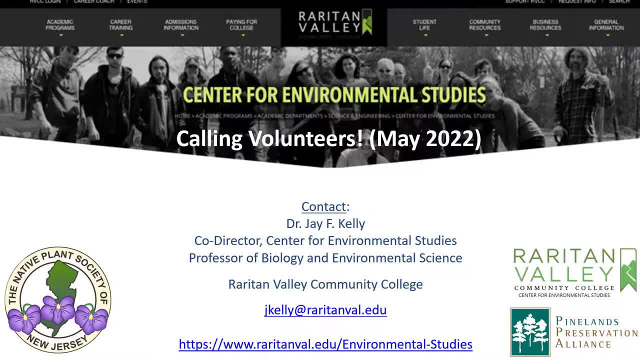 Sure, Collins and Anderson, Buell and Robichaud. There's a bunch of books on vegetation communities in New Jersey. There's a bunch of books on the area. There's a bunch of books on the area. There's a bunch of books on the area. 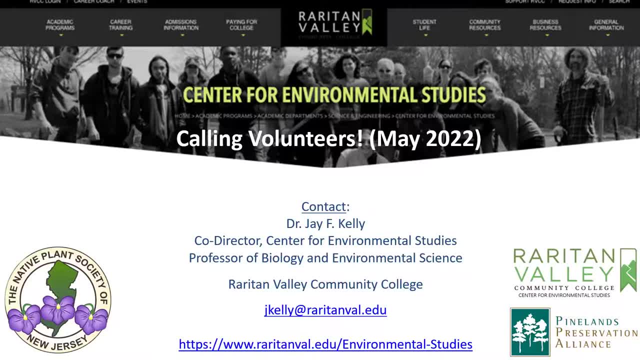 Jersey and those are great references to start with. Those were published largely in the 60s and 70s but they have good lists of the dominant species in each of the different habitat types throughout New Jersey and that's a really good place to start. So those books are titled Plant. 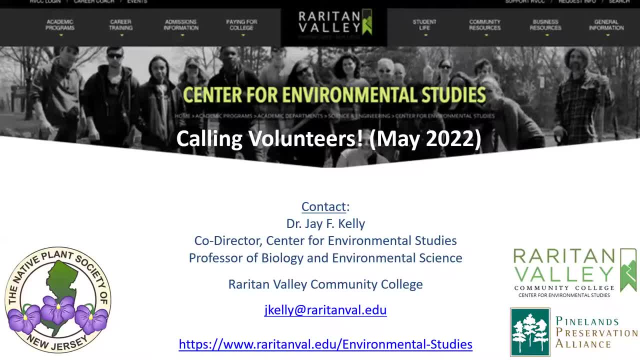 Communities of New Jersey, I think, is one title and Vegetation New Jersey is the other, if I remember right. Okay, so maybe we can post a list of those, after the conference, Which native vines will bounce back with the deer exclosures. From what we've seen, the ones that bounce back. 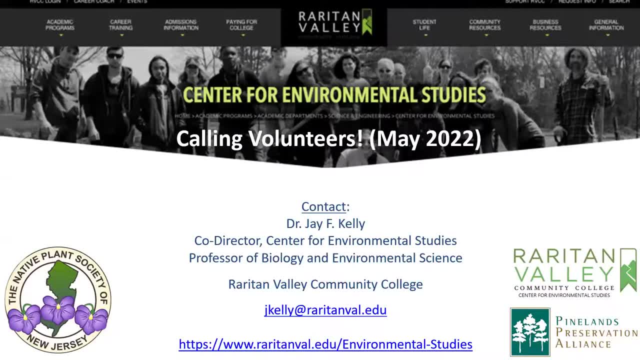 right away are poison ivy and grapes. Deer appear to be immune to poison ivy and so they munch it down, and that's one of the maybe unfortunate effects Of putting deer exclosures up is the poison ivy responds right away. Poison ivy is a beautiful 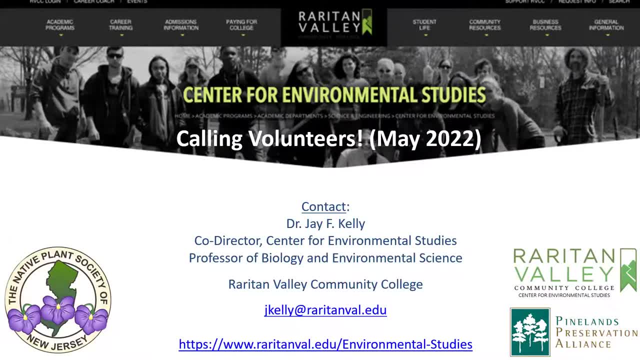 plant. It changes to lovely colors in the fall and it's really important for bird migration in particular because the birds feed on the berries as they move through. But you know, for those of us that are sensitive to poison ivy and its effects, it maybe isn't so pleasant. So yeah, 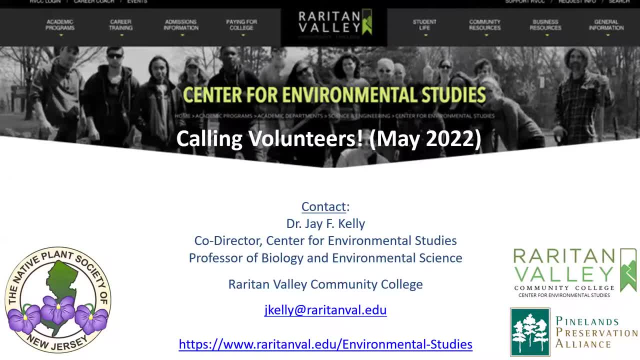 the vines come right back, including the grapes and poison ivy. I can't recall off the top of my head what other ones come back right away. Okay, Can you buy deer meat in New Jersey? I think you can buy imported deer meat. Is the local deer meat? excluded. Yeah, you're not allowed to sell deer meat in New Jersey unless it comes from, I think, a registered farm where there's a captive population that is licensed for sale. You're not allowed to kill a deer and sell it commercially in New Jersey or, I think, anywhere in this country at this point. 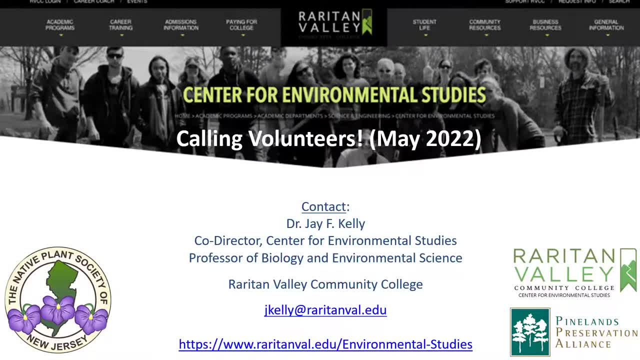 Oh, From the wild. From the wild, Let's see. You are sharing your PDF. I think you said Happy to. Okay, Let's see. I don't know if we have too much more. Somebody says they're pulling out their English ivy, which sounds like a good idea. 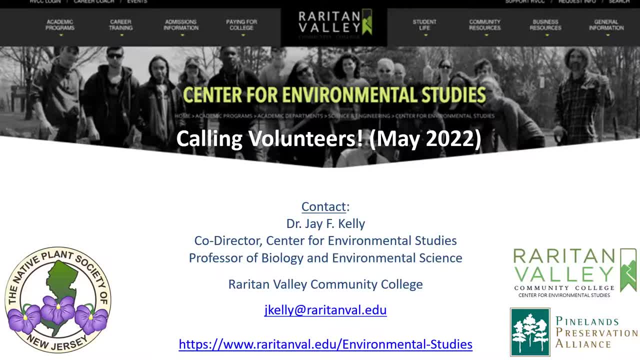 What could we replace it with? I guess a vine, A nice, lovely one, to replace it with Some of our native honeysuckles or trumpet creeper. They're beautiful flowering vines that are great for hummingbirds and many other species. So those are two easy ones to replace the ivy with. That's what we did in our yard and it is definitely worth it. Let's see Where can they get the white cages for the young trees that were shown. There's a number of different products available online. If you just search for it in Google- tree tubes or tree cages- they'll come right up. They tend to cost anywhere from $1 to $5 a piece, Depends on how tall you want them, whether they've got ventilation holes in them and so forth, But that's the approximate range of prices for them. Also, it's cheaper if you buy them in bulk as well. 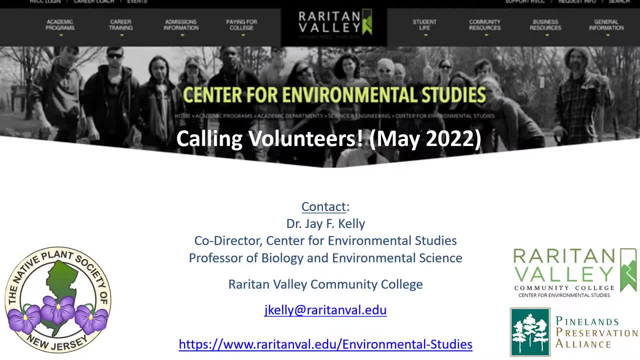 Okay, How can we get businesses to stop selling invasives? Well, you can go in there and start complaining. That's the first thing to do. Ask them if they have natives. if they don't complain about it, complain about the invasives that they're selling. But we really need to get laws on the books that prevent them from being able to sell these things, or at least tax them for doing it, so that we can use the revenue to try to tackle some of these problems in our landscape and fund meaningful restoration efforts in the state. 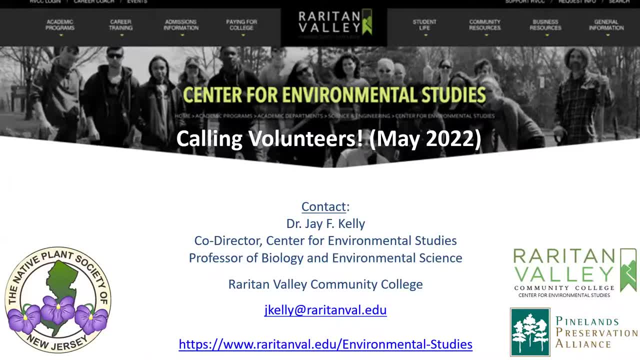 But it's really. you know, many other states have laws on the books. There's regional cooperative initiatives that Mike Van Cleft from FOBOS has been participating in, where you know groups are trying to coordinate their efforts and try to come up with strategic policy solutions. 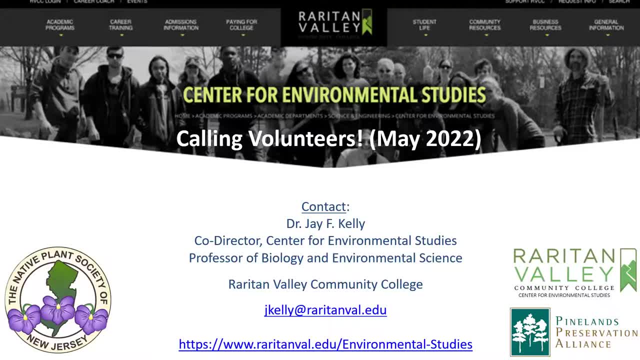 to prevent this from continuing in the state, But right now, the landscaping and nursery industry is a really powerful lobby in the New Jersey legislature, and they've prevented any or most proposals that have come up in the past 25 years from getting passed, And so that's why we need, you know, this constituency to really rise up and start calling up their politicians, and 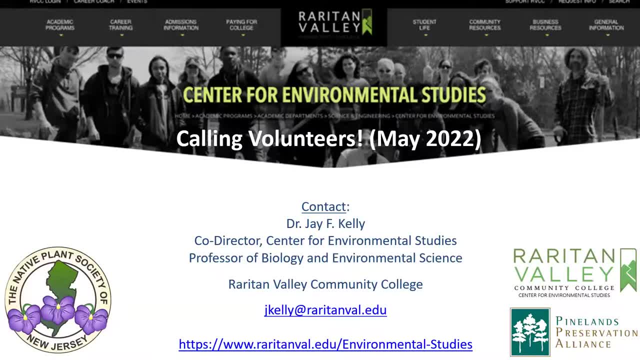 supporting the conservation groups in New Jersey that are working on these issues to try to get meaningful changes passed At the policy level. What's the definition of an old growth forest? There's dozens of definitions. I don't think I used that word. I used old, intact forests. Some people refer to them as primary forests. 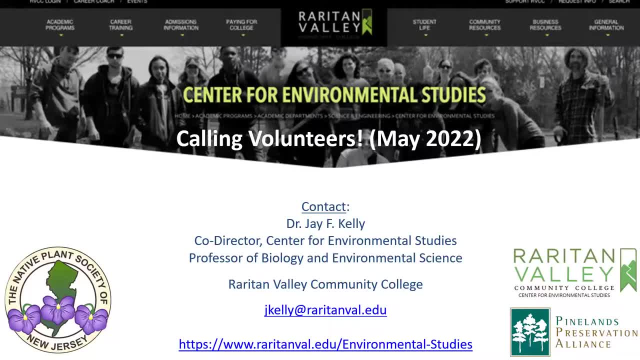 But in New Jersey there's only a few stands of trees that have no record historically of ever being logged. One of them was Hutchinson Memorial Forest at Rutgers, their research forest that I showed you some research from. There's another one called Bear Swamp, way down in the state. 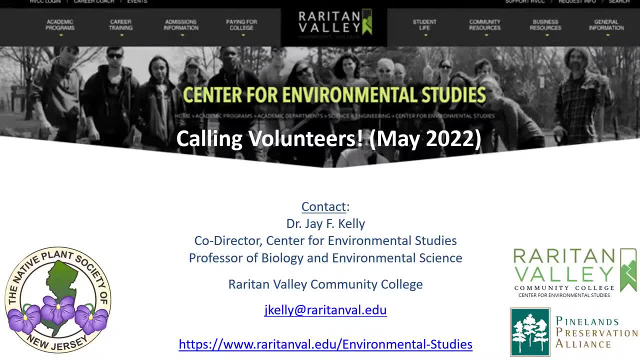 And there's another one in South Jersey and there probably are a few other stands here and there. Most of our forests have been impacted by logging, either selectively or through clear cutting in the past couple hundred years. But the forest that have intact soils, even if you cut the trees down and there's an intact seed bank and soil community, the forest can recover because the forests are adapted to those kinds of disturbances. 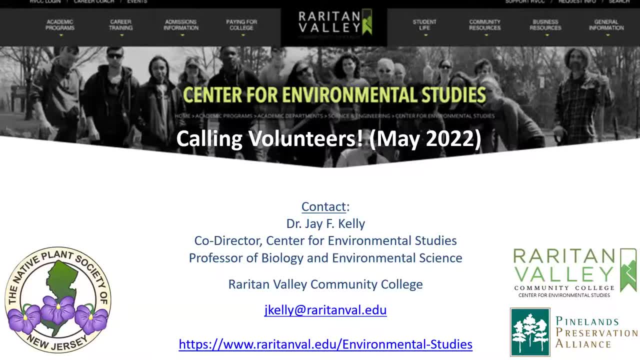 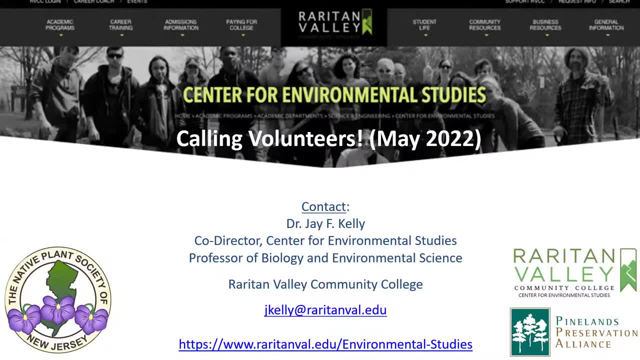 Whether or not you want to call it a forest or not, it's up to you. the clear priority for forest preservation in New Jersey. What's the best information I can share about what private landowners can do to address the deer problem? It depends what they want to do about it. 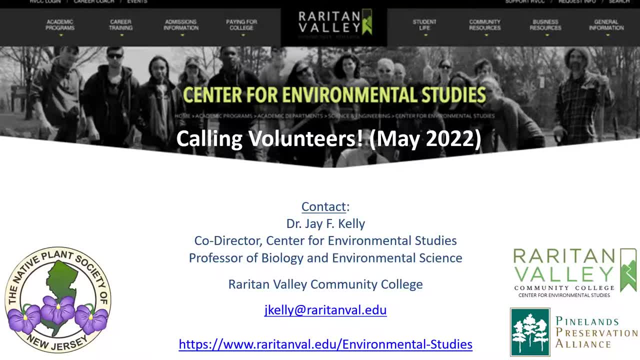 You know you can hunt on private property and so you can look to the state government for the regulations that you know implement safety zones from adjacent properties or structures. It depends if you want to install a deer fence, you know, then you could go to groups like Deer Busters. 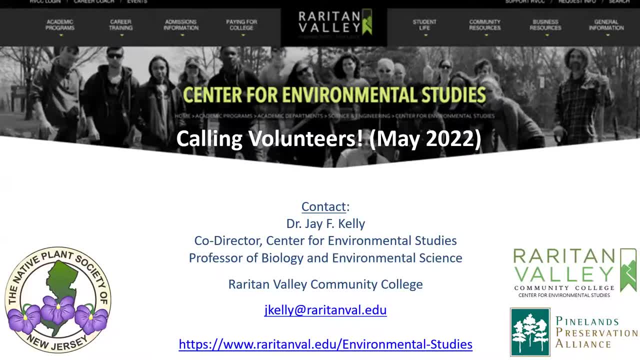 or Benner Fencing or any of the vendors online that sell these materials. If you're interested in planting native species, we've got, you know, wonderful organizations locally that are making them available to us, whether it's, you know, Randy's group at Toadshade. 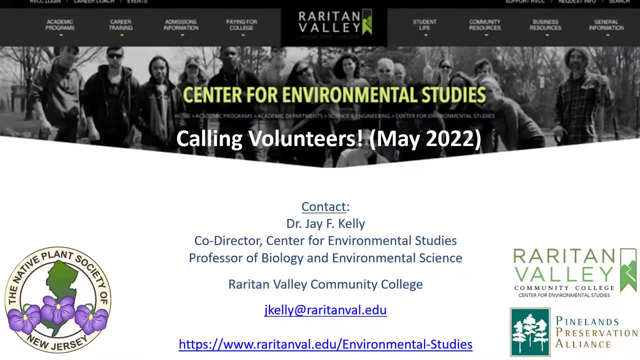 or Wild Ridge Plants that Jared Rosenbaum runs. Duke Farms is growing a lot of native plants and many of our local nonprofits have native plant sales throughout the year. You know, one of the best resources is right across the water in Pennsylvania at Bowman's Hill Wildflower Preserve. 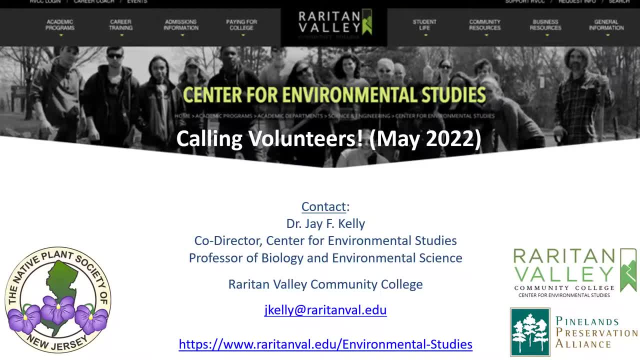 So you know, it really depends on what strategy you're hoping to make use of to tackle these problems that I could, you know, be of better help to point you to resources for them. Okay, is there any use to making small? 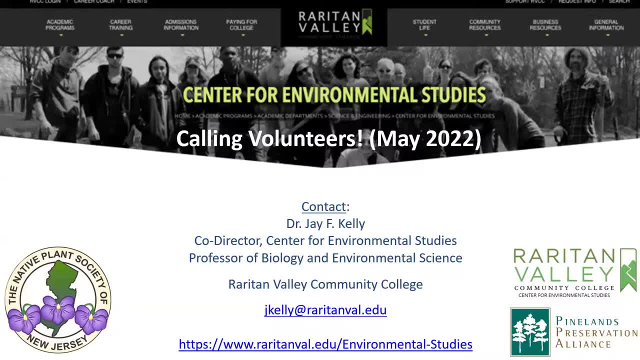 small plots of 60 feet by 100 feet into pocket parks, if financially possible, Absolutely. You know, at this point 30% of the land area in New Jersey is occupied by urban land uses right. That's a huge amount of land. 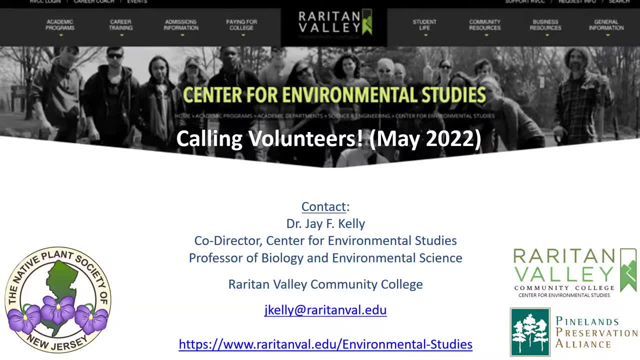 that we've displaced native species from through our suburban developments and our urban and commercial spaces, And every inch that we can reclaim for supporting native flora and fauna, you know, can be really vital for maintaining those species in those kinds of urban environments and just for providing additional resources. 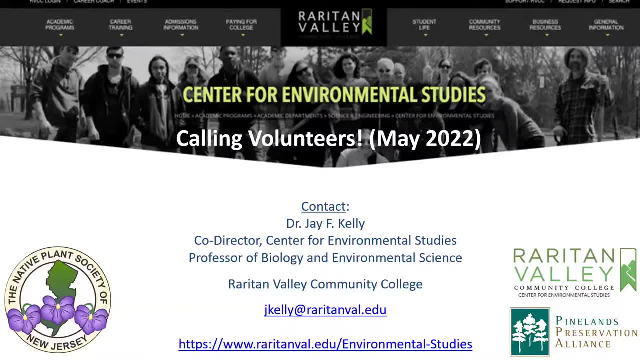 for them to occupy the state. We really have to start thinking about how we can coexist with these species in a mutually enhancing way in the landscape and not to the exclusion of everything else besides ourselves, And I think there's extraordinary opportunities for whether it's urban agriculture or urban restoration. 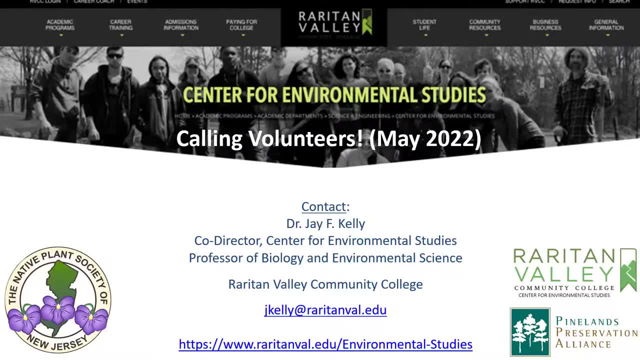 to take place in our own backyards and suburban and urban areas throughout the state And it really is another, I think, major frontier and priority for us. I think more than it's possible and many of us think for conservation in the future in this region in particular. 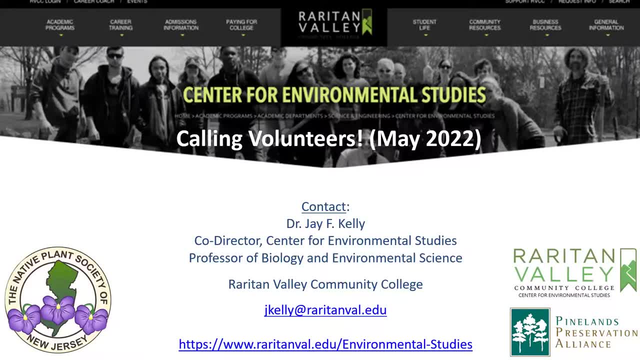 Question is: will you give this lecture on deer management to other groups? I've given this talk over a hundred times in the past seven years And so, yeah, I'm still at it and happy to give it some more, you know. 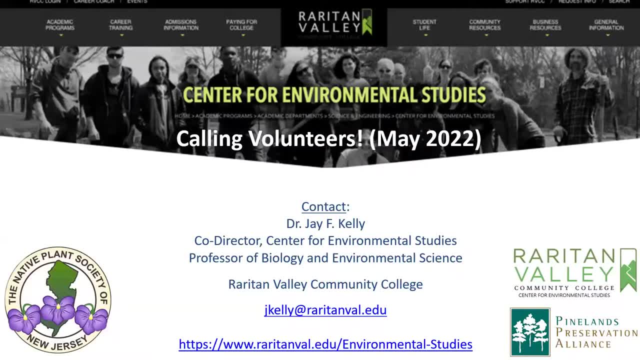 So yes is the short answer, but I'm certainly tired of it. I would love for these issues to get addressed so they don't have to give this talk anymore. It'd be nice to see some positive change so that it doesn't you know, it is no longer necessary. 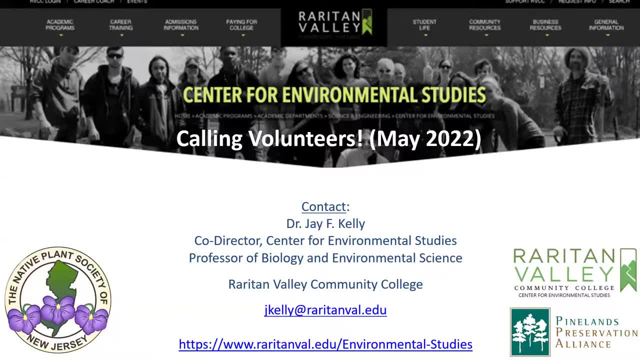 to bring such bad news to all these groups around the region. But, yeah, I'm happy to support any efforts that local groups are trying to engage, whether it's to inform the public. We give talks to local officials as well as to public groups of various kinds. 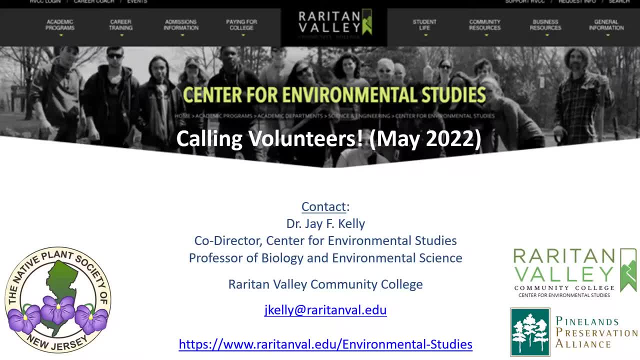 and anything we can do to support public education and conservation, we're happy to do so. Okay, here's not a question but a thank you. Thank you for a wonderful overview: Semester's worth of information in an hour. Hope we didn't lose too many people for you, Hubert. 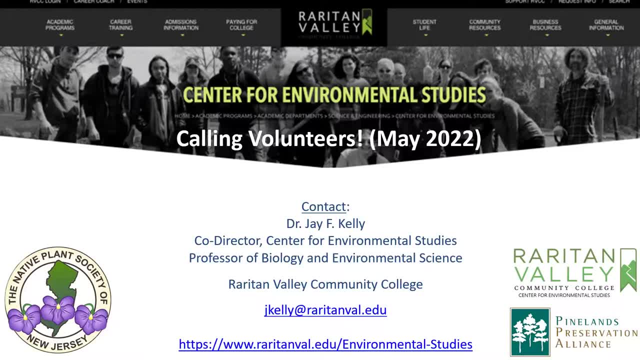 It was a lot. I think it was a great presentation. We'd like to thank you very much for your presentation and for your time and expertise in this area. Yeah, and don't forget to come join us on the beach, as this may and help put some-. 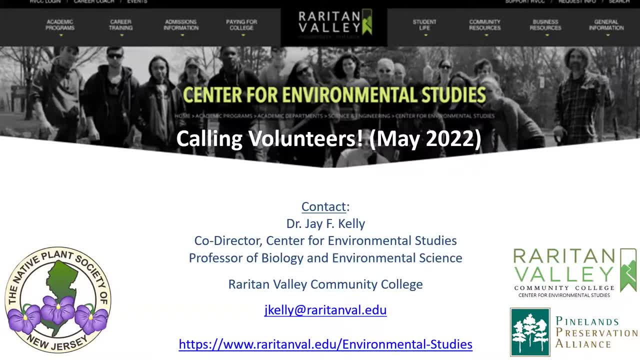 I'll be announcing that. Just let me know and I can check with your. I'll check with you and we'll make special announcements, All right? well, thanks again, everybody for your time and enjoy the rest of your day and the events that are in store. 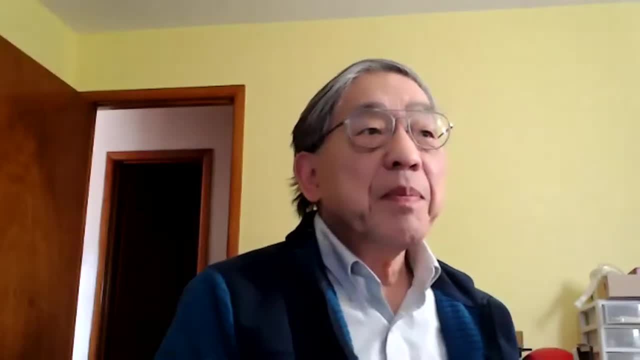 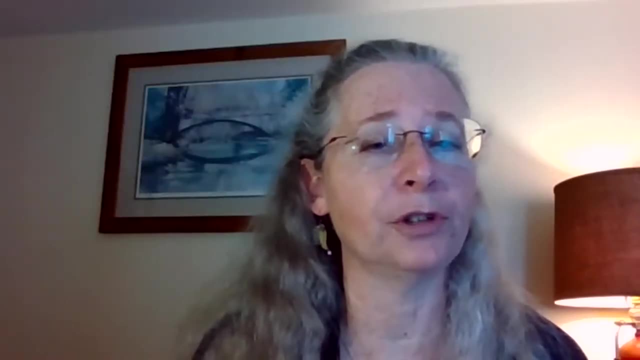 Okay, thank you very much. Thanks, Jay. I think I'm up to send people off to lunch here, Hubert, Is that true? Okay, yeah, and Amelia's gonna run a slideshow, I think. Okay, Well, I did wanna take just a few minutes. 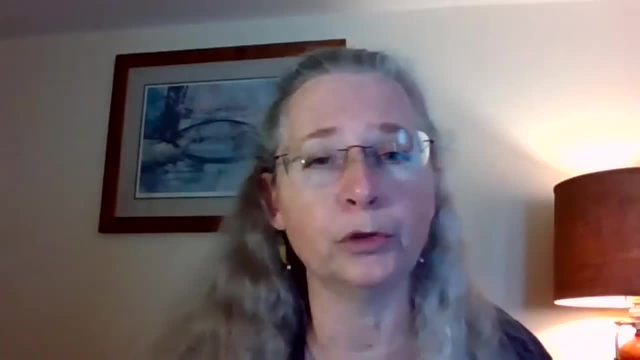 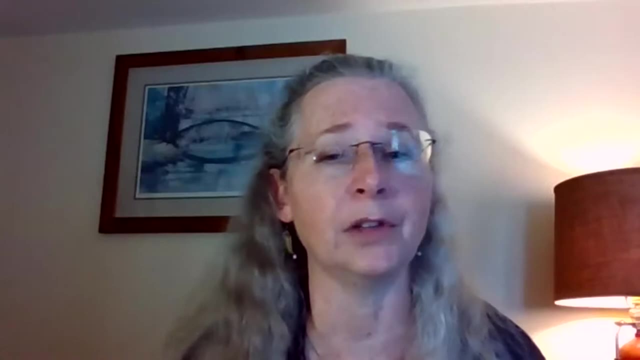 before everybody started running away. Don't start running away for lunch yet. Mm-hmm, I'm trying to keep-. Okay, Jay Kelly, on schedule there. We did sort of skip the introduction of the new officers so you didn't get to see their smiling faces. 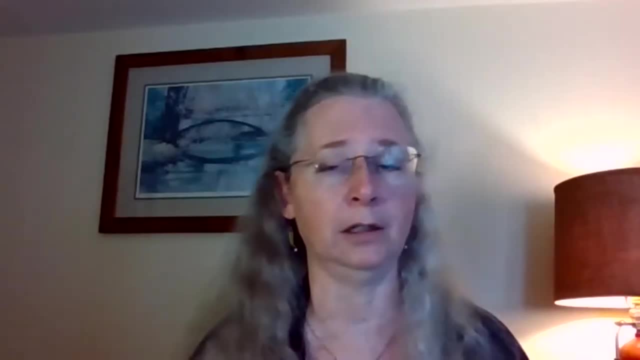 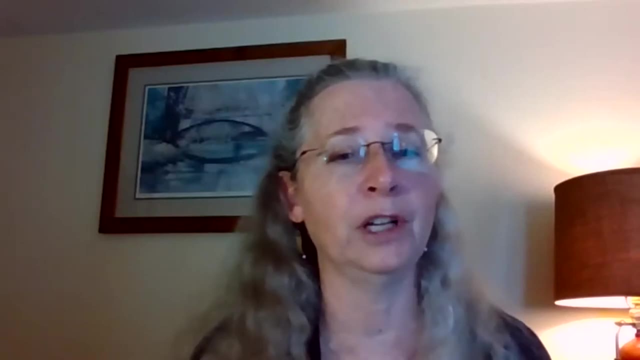 So I was wondering if the officers that just got elected- if you can, there we go. There's Bobbi Hearns, So she's our new corresponding secretary. There's Deb Ellis, our new vice president in charge of membership. Faces are bouncing around. 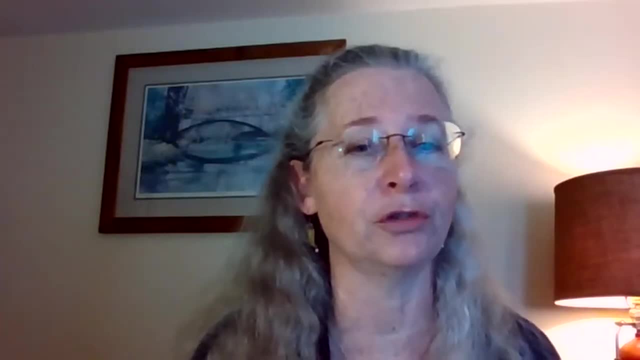 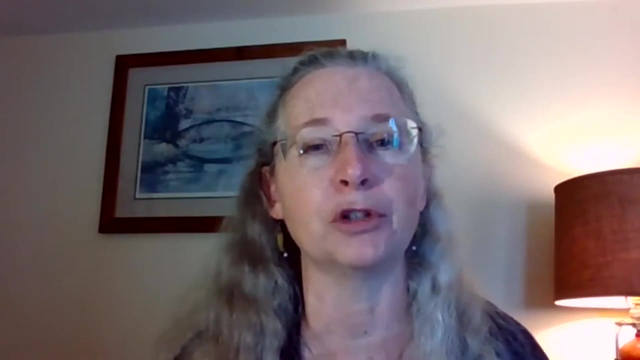 There's Bob Swain, our treasurer. I'd like to say: you're our new treasurer, Bob, but you've been treasurer for a while and we welcome you back at that. And there's Karen Sparrow, our new vice president of membership. 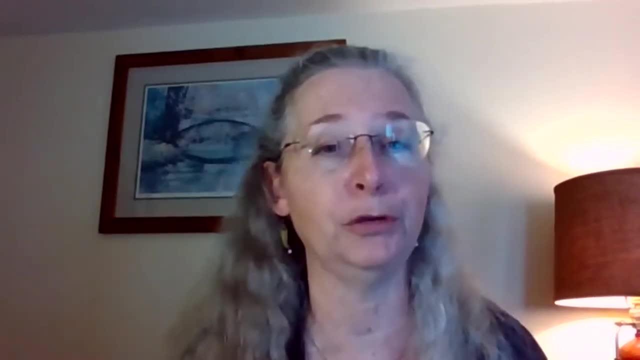 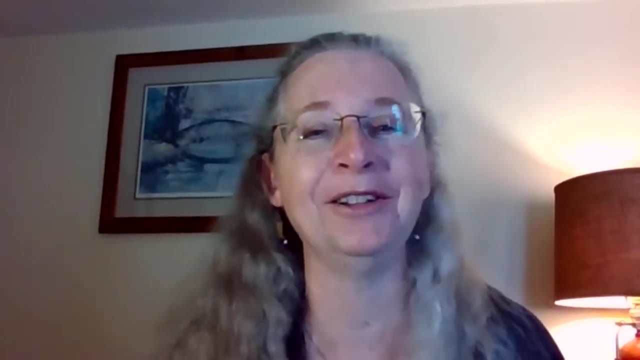 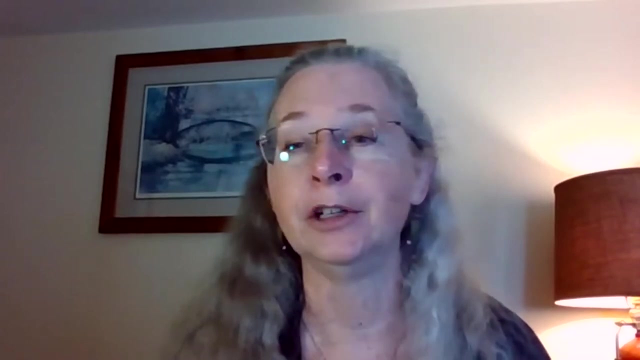 So now you have faces to put with the new positions that are there And, of course, Rusty Bell that you saw earlier. that, yeah, and the dog Rusty Bell that introduced us all earlier, He is our recording secretary. So thank you very much everyone.